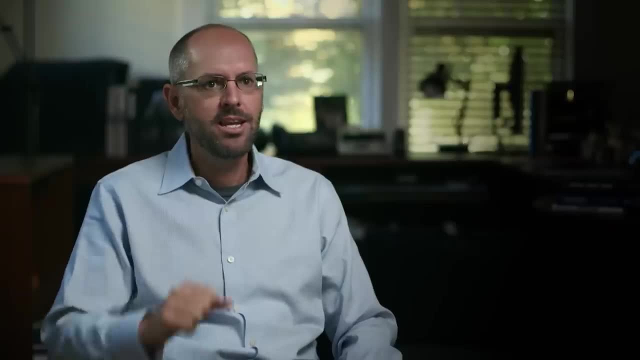 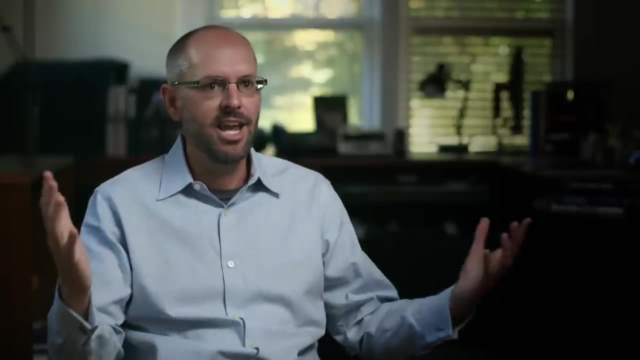 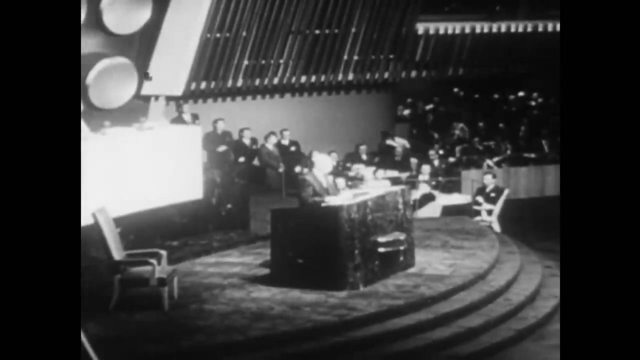 It began with a lot of gloom and doom, And then he circles around and ends with this beautiful, happy tale of how atomic energy is going to bring blessings and health and prosperity to the world. This greatest of destructive forces can be developed into a great boom for the benefit. 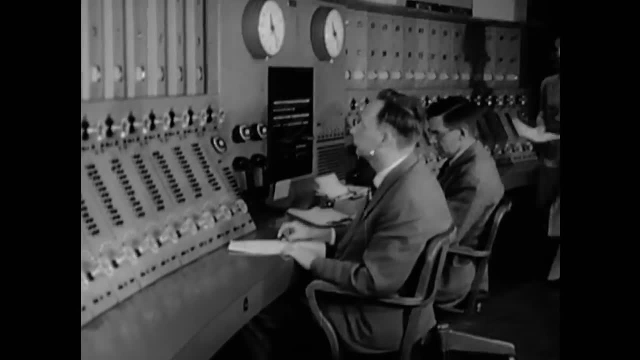 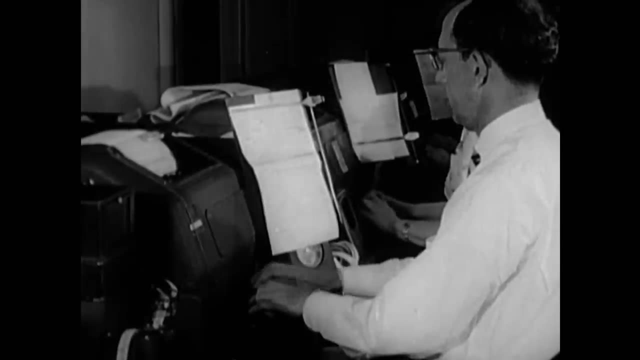 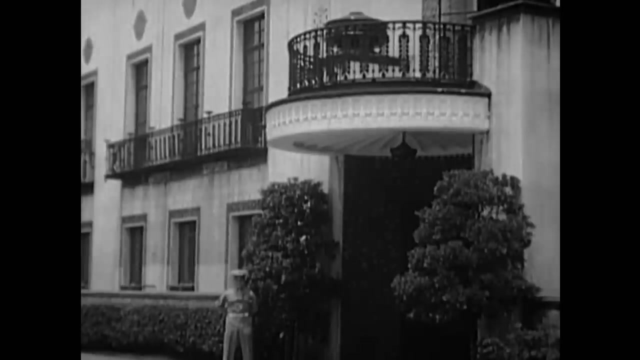 of all mankind. The president's speech was immediately transmitted to 74 overseas posts by the USIA press service. before the communists could distort and misinterpret America's proposals, Atoms for Peace quickly became international. At American embassies all over the world, the USIA campaign got underway. 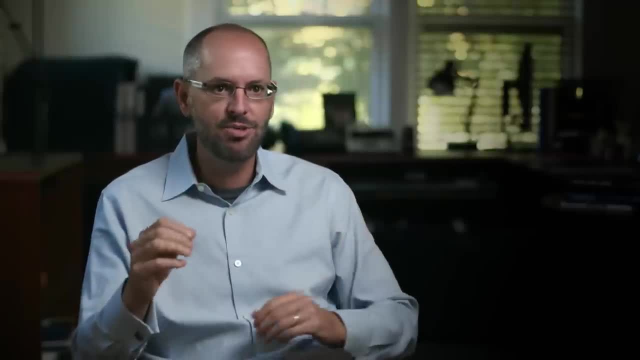 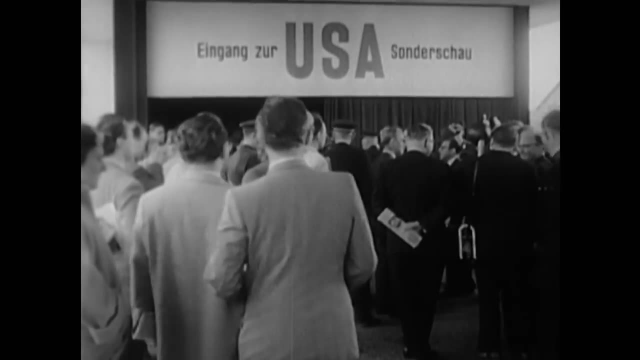 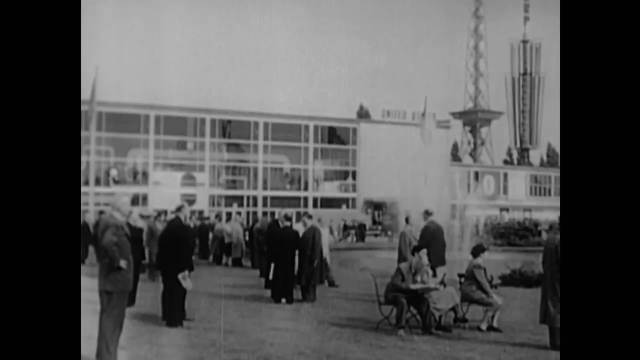 The propaganda around Atoms for Peace included traveling exhibits where people could go and see little nuclear artifacts, And these exhibits would attract throngs of people around the world. The exhibit in West Berlin was visited by a quarter of a million people, including thousands from the Soviet zone. 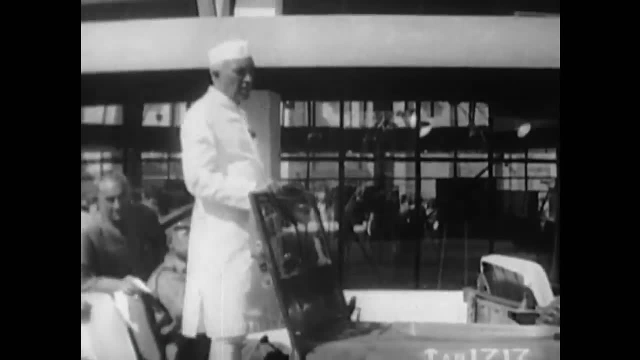 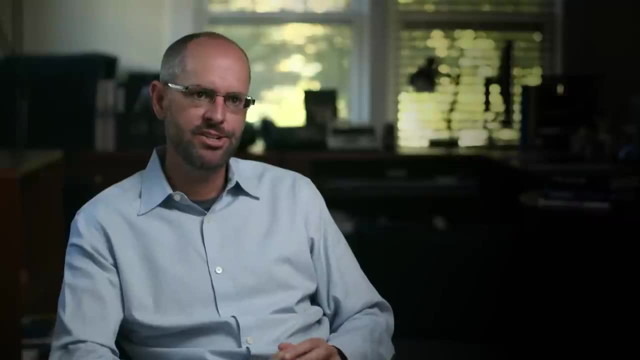 In India, Prime Minister Nehru came to view the exhibit. The exhibition was held in Berlin. The exhibition was held in Berlin. The exhibition was held in Berlin And shared the experience with thousands of his countrymen. Of all the countries that were targeted for Atoms for Peace propaganda, none was more. 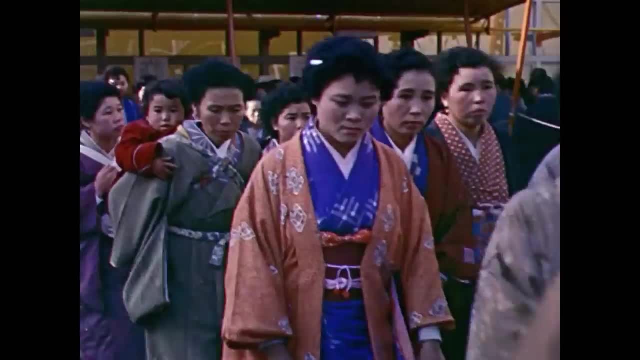 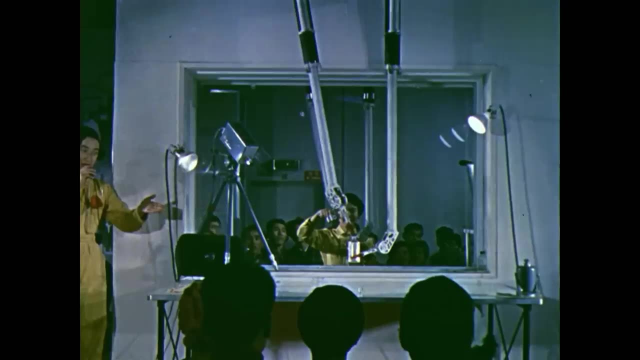 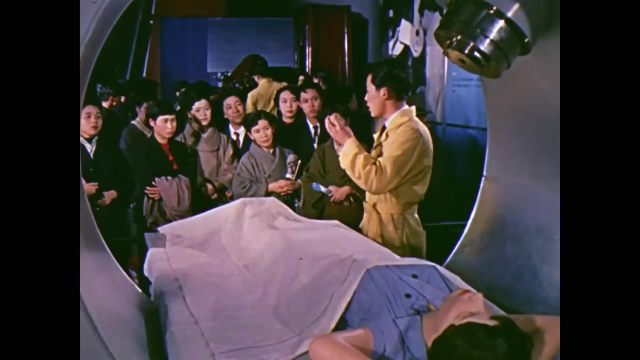 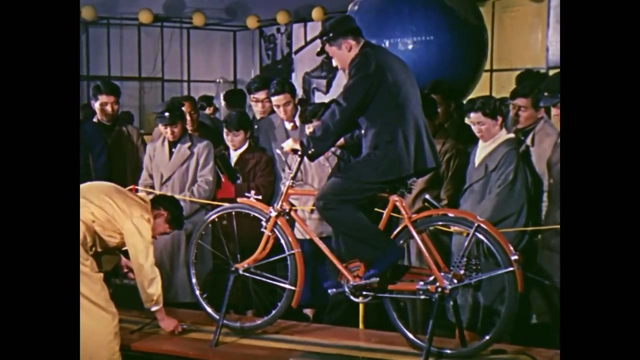 important to the American government than Japan. On the first day of November 1955, the United States Atoms for Peace exhibition opened in Hibiya Park, Tokyo. The United States sent exhibits to Japan. It promoted the work of Japanese scientists in atomic energy work. Atoms for Peace helped sort of send this message that hey, we're the good guys. It sort of helped whitewash the bad odor created by Hiroshima and Nagasaki. The general public was being encouraged to look on the bright side, so to speak. 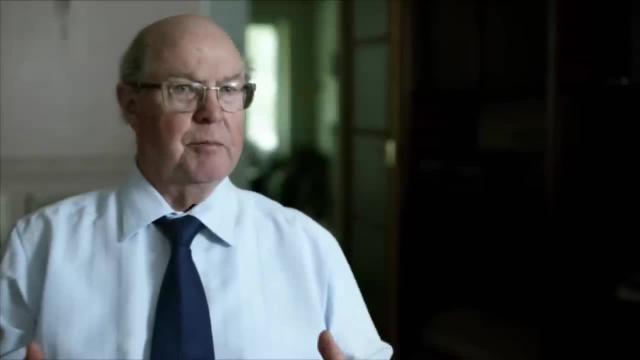 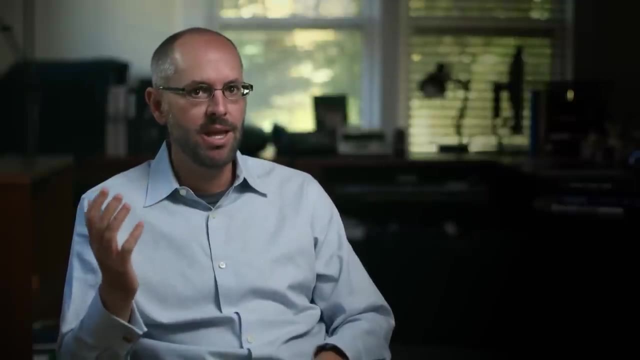 by demonstrating that there was this enthusiasm burgeoning all over the world. Was it propaganda or was it policy? The answer is it was both. It was, at the same time, an effort to influence public perceptions, to change the way people talked about nuclear energy. 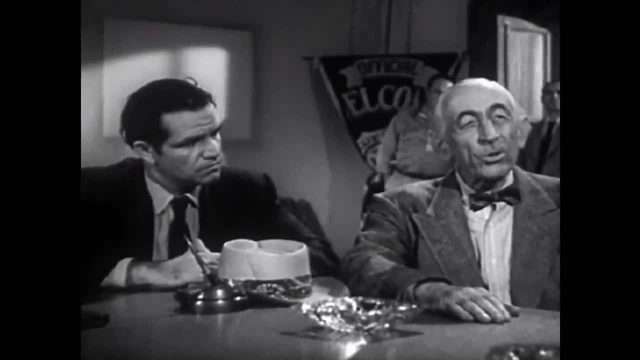 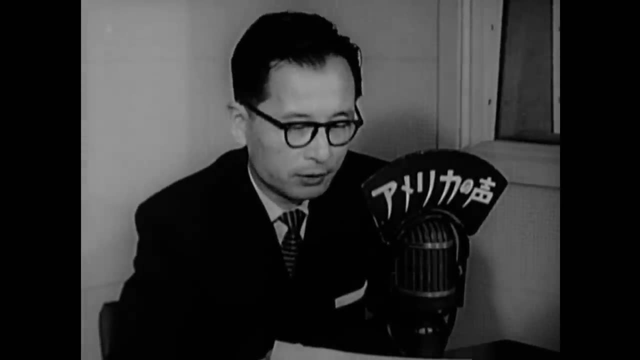 I voted against atomic energy because I thought it was the work of the devil- Now I know I was wrong- And, on the other hand, it was a serious, genuine initiative to spread what they saw as the benefits of atomic power throughout the world. 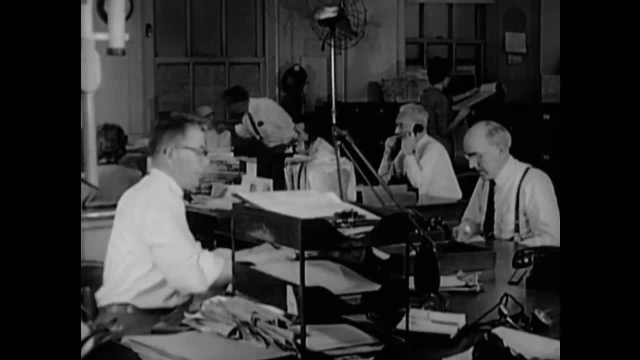 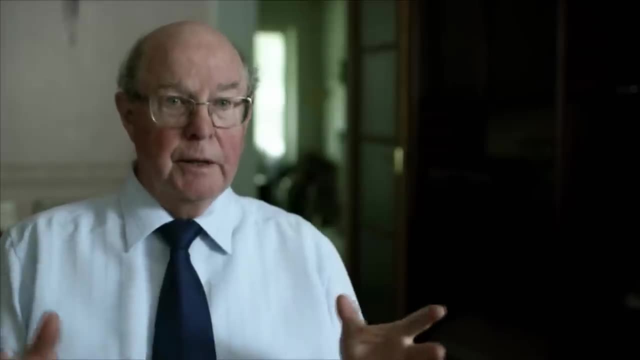 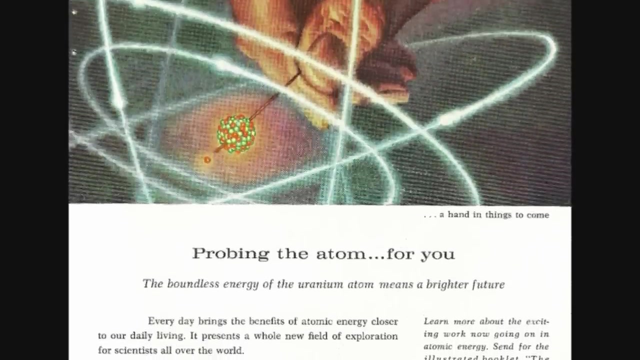 The voice of America was beginning to give the world translations of the president's words in 43 languages. The potential of civil nuclear power suddenly was seen as a global beacon of progress. Every country involved wanted to take part in the development of this new, gleaming future of atomic energy. 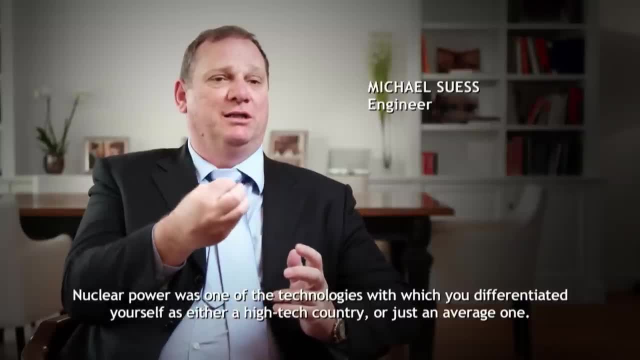 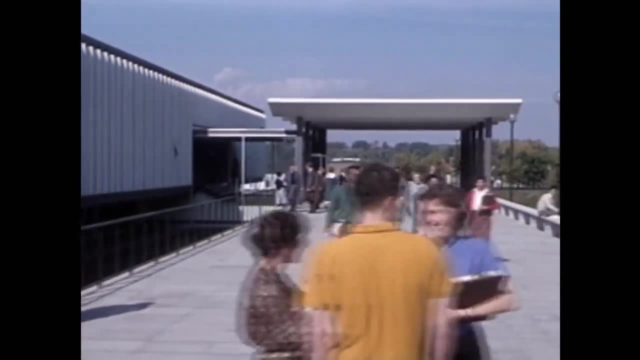 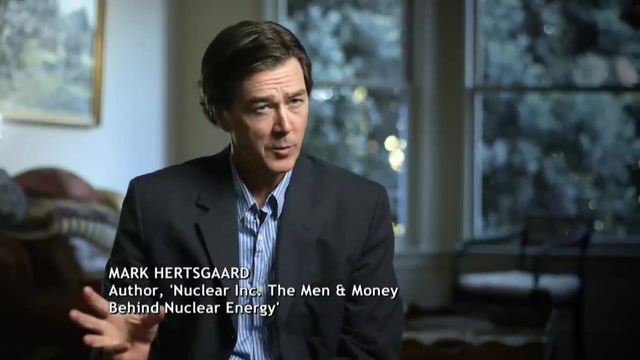 Nuclear power was one of the technologies with which people differed. Whether you were a high-tech country or if you were a young scientist or engineer graduating college in the 1950s in the United States of America, you were in a pretty sweet place. 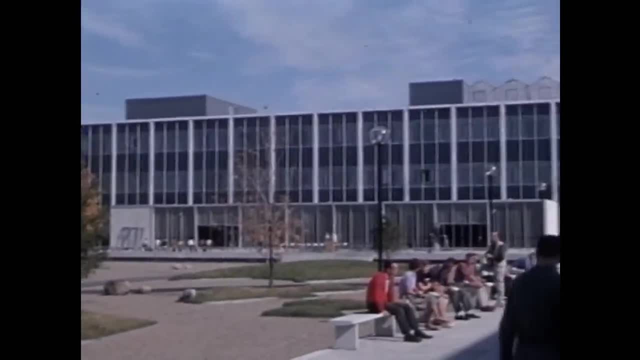 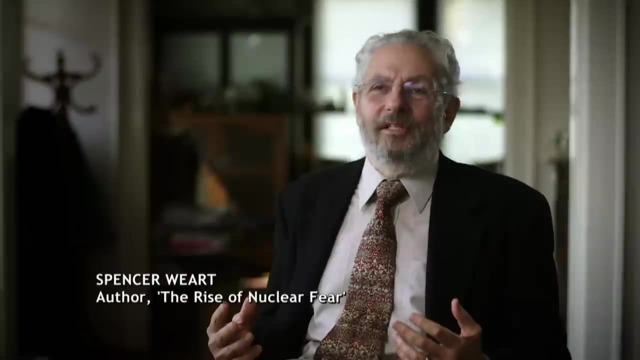 Possibly you could make an analogy to the dot-com boom in the 90s, but it's bigger than that. It's huge. The scientists had stepped forward as the new wizards, the warlocks, the magicians who were going to bring all these wonderful things to the future. 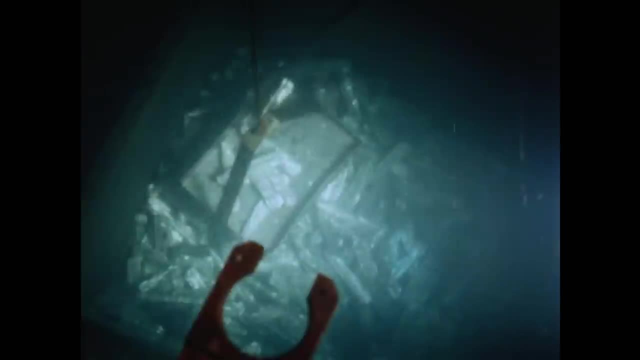 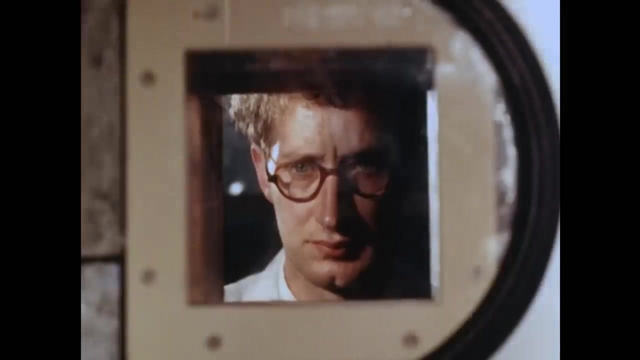 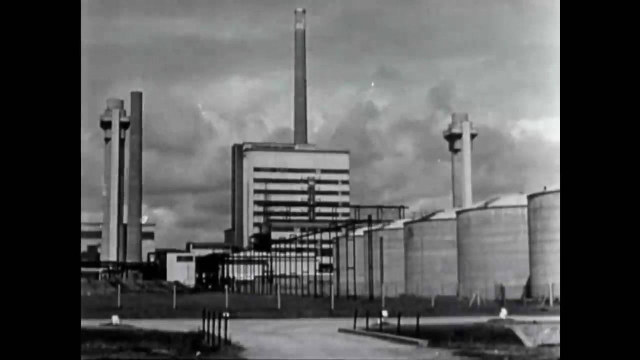 They were like inside the shell of this magical world. You know, the scientists that studied this were really fascinating people and they were part of this very, very elite group of special people. The British set up the first civil nuclear plant at Calder Hall in the UK. 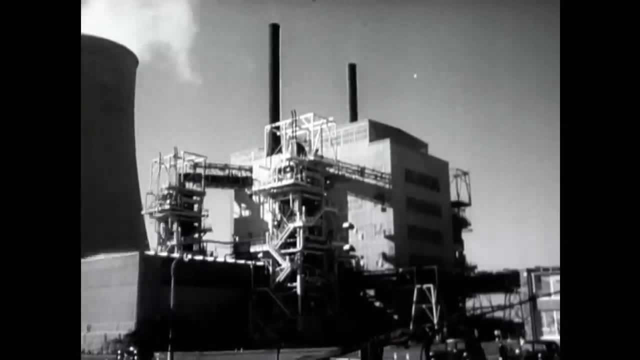 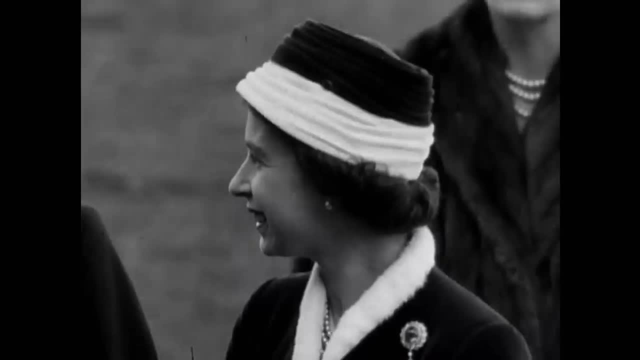 Appropriately for such a very important event, the Queen came to perform the ceremony of the big switch-on. A definite lead in the second industrial revolution has been taken by Britain. The British government was triumphant at being the first nation to launch a nuclear power programme. 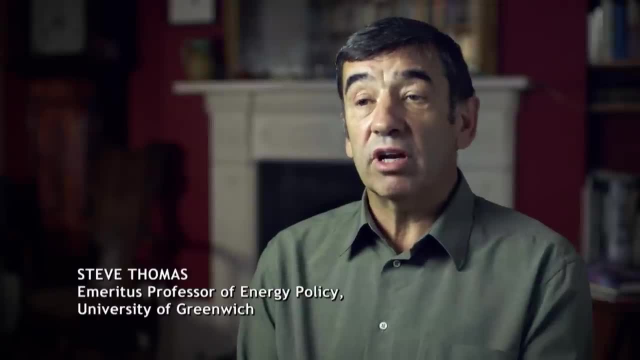 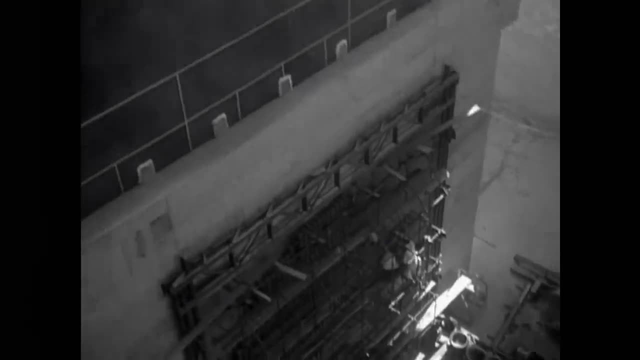 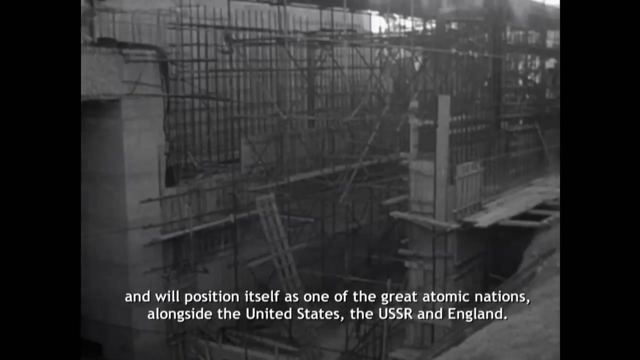 Britain saw itself as the pioneer of nuclear power. We were the first with a nuclear power station and our technology led the world, But others weren't far behind them. France will enter the nuclear production of electricity and will place itself in the ranks of the great atomic nations. with the United States, the USSR and England. When De Gaulle came to power after the Second World War, his concern was to restore the glory of France, the position of France as a power. And so, from October 1945, General De Gaulle by order. 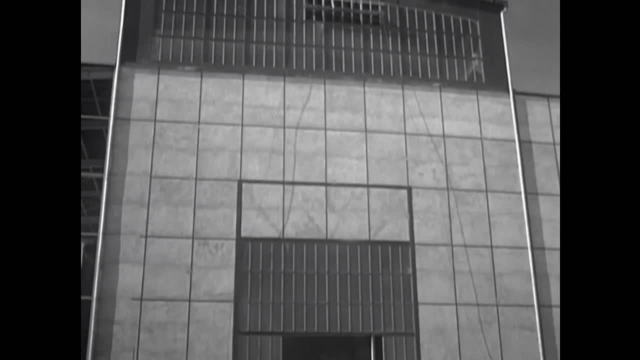 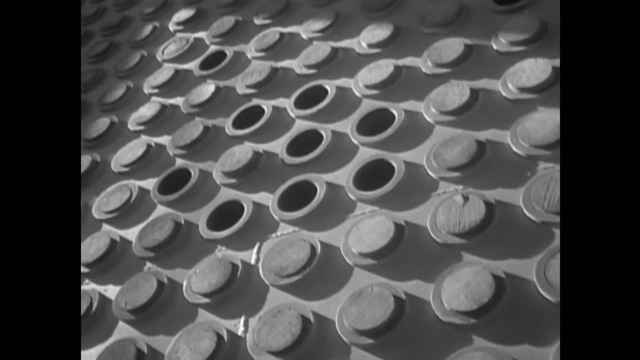 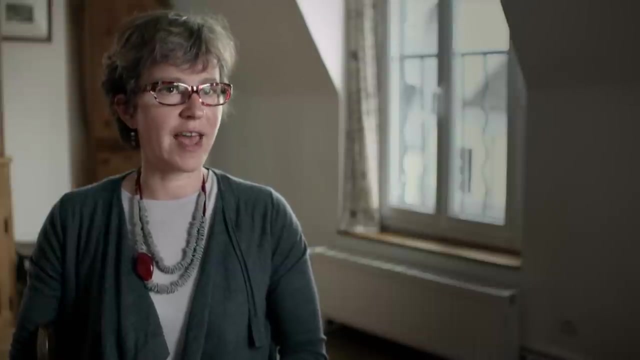 created the Atomic Energy Commission, Even if some slight deception was involved in explaining what these shiny new reactors were actually for. The first nuclear power site in France was presented as a prototype for electricity generation, and that was what all the fanfare was about. In reality, and from the very beginning, the Mark 2 reactors were designed to optimise the production of weapons-grade plutonium. Gold Hall wasn't a power reactor. Its purpose was to produce weapons-grade plutonium material. The electricity was a useful by-product. 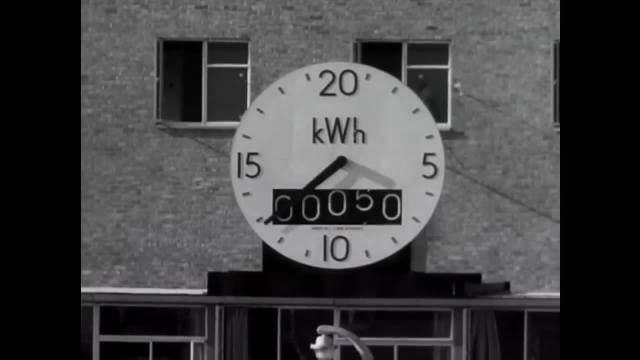 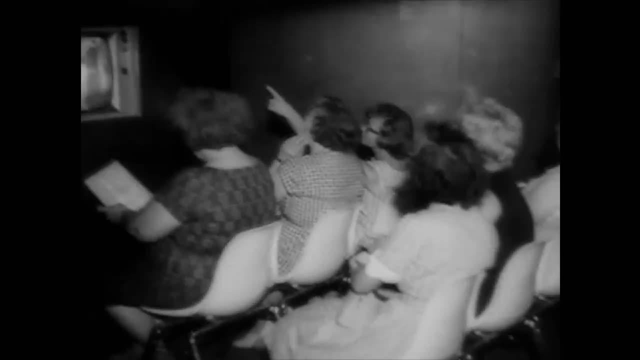 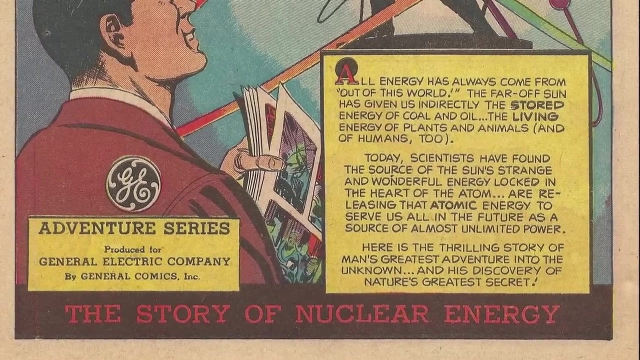 And in fact that dial was not connected to the reactor at all. Governments weren't the only ones spinning a positive atomic message. Private nuclear companies were getting in on the act too. General Electric was really instrumental in this. They did a lot of work. 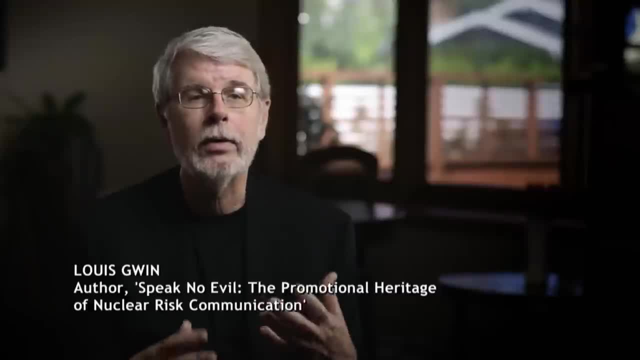 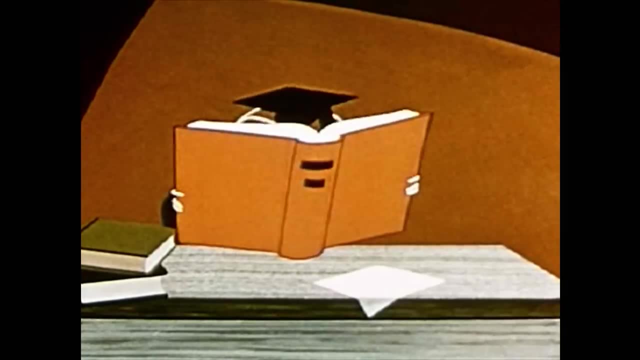 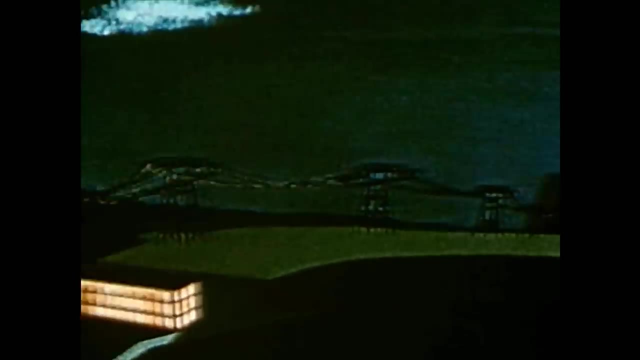 They had a comic book, they had film strips and it was all done with bright colours, with exciting little characters. Let's start by meeting a leading authority on the subject, Dr Atom. The public's mood was galvanised by the new atomic power stations springing up around them. 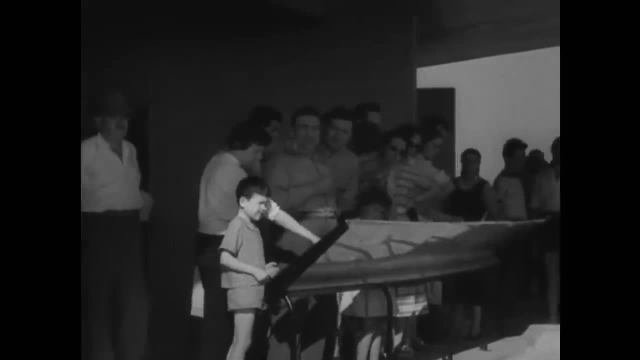 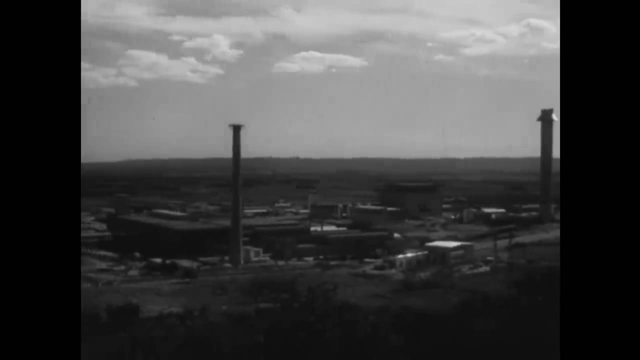 The reactors actually became tourist attractions in and of themselves. At Marcoule there was a lookout point where tourists could go and view models of the reactor and see the whole site Growing up in Essex and going for days out on the River Blackwater. 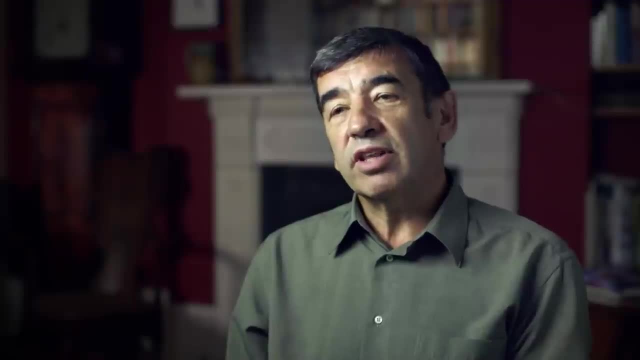 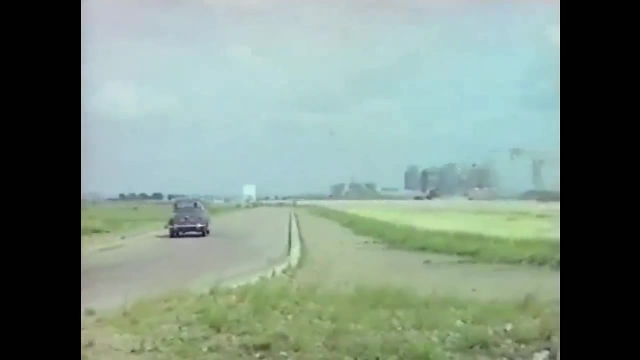 I remember very well driving there along small country roads, But as I got close to Bradwell the roads suddenly became very large and very impressive and you could look along towards the mouth of the river and see this very clean, very efficient nuclear power station. 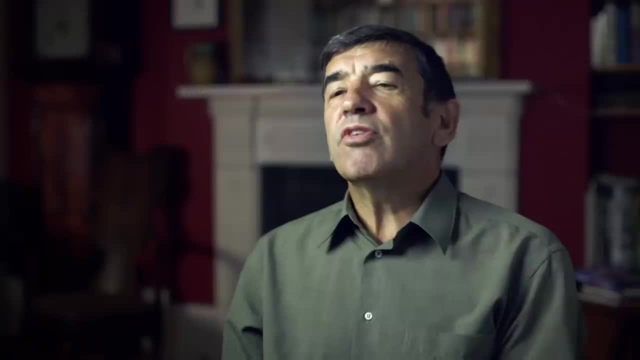 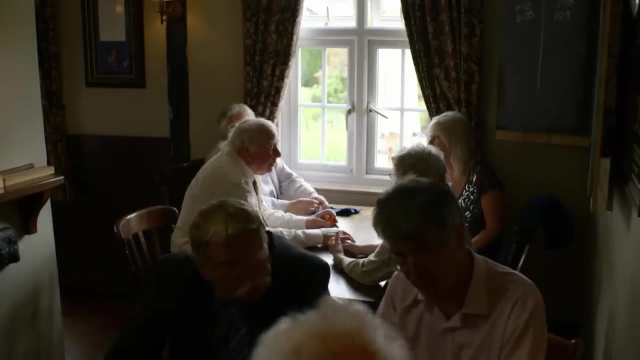 It looked very modern, It looked the future, But no-one felt the thrill quite so much as those on the inside. I felt proud to work at Bradwell. When I look back I think, yeah, I was there, I did that. 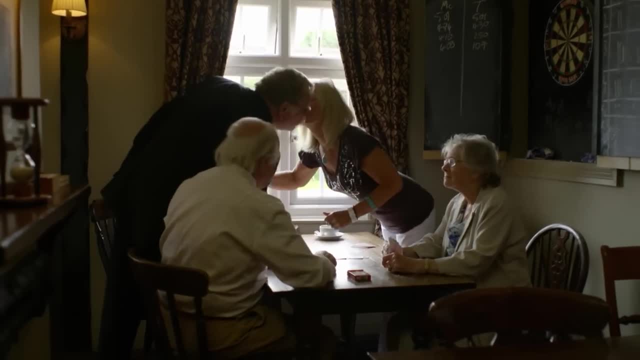 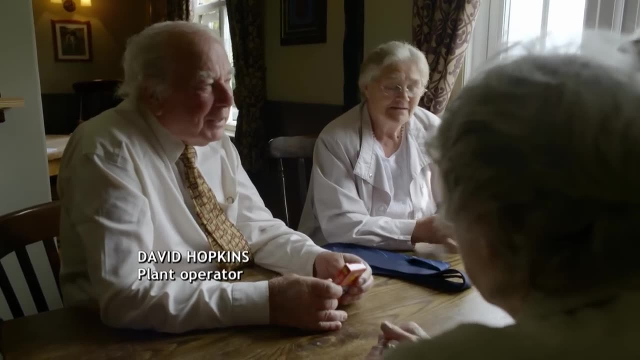 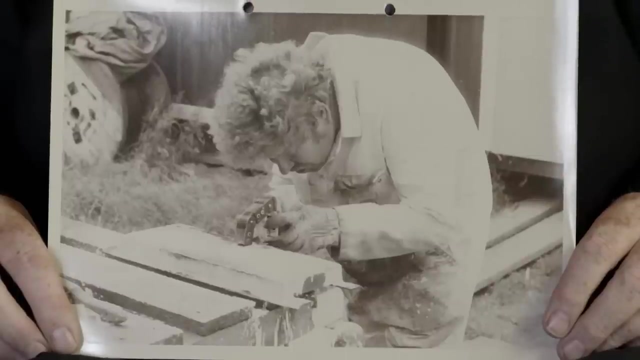 Hello, Hello. We felt we were at the forefront of technology. It wasn't only Bradwell, The country as a whole was raising their head up and saying we can make it. 50 years has gone by since then. I even had a lot of hair. 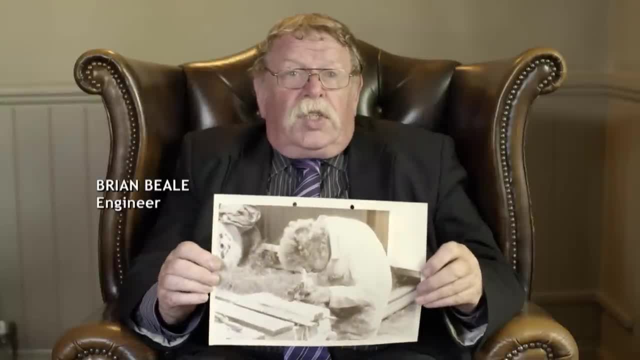 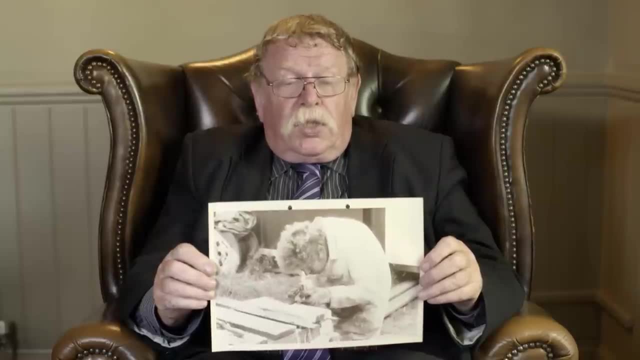 And one of my jobs was to test materials for faults, defects and used to climb inside the reactor building main structure, inside the ducts and everything, and test all of the welds. Looking rather like a super version of a plastic Macintosh. 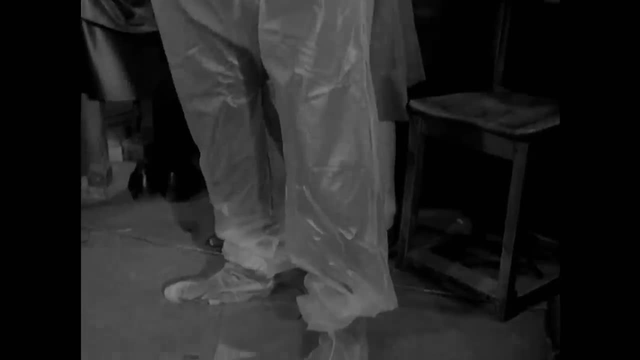 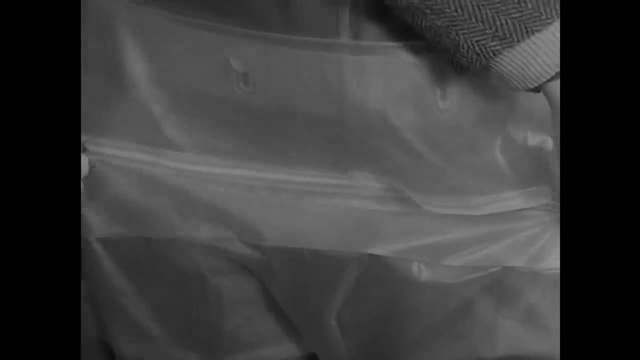 is a new suit designed for workers at Britain's atomic plants. Once you're inside and the zip's been fastened, all that remains is to pump in compressed air so that the wearer can breathe easily. I used to be dressed up like a Michelin man. 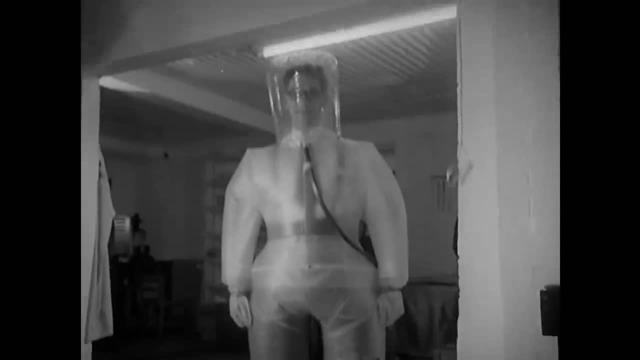 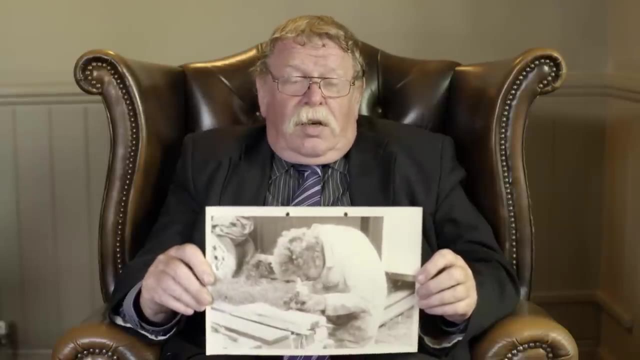 with special clothing, with an umbilical cord supplying air to my body, sort of thing, and for breathing and also throat microphones, and then climbed through every part of the reactor, In the boilers et cetera. We were looked up to because people from coal plants 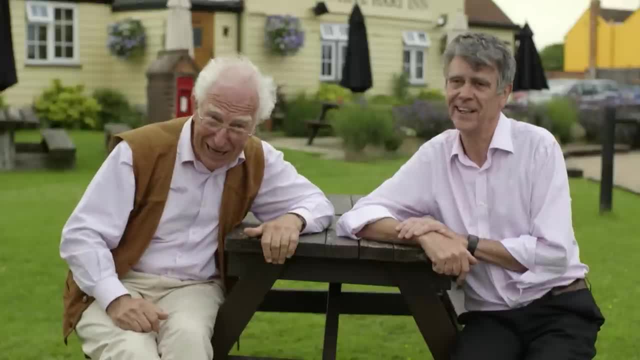 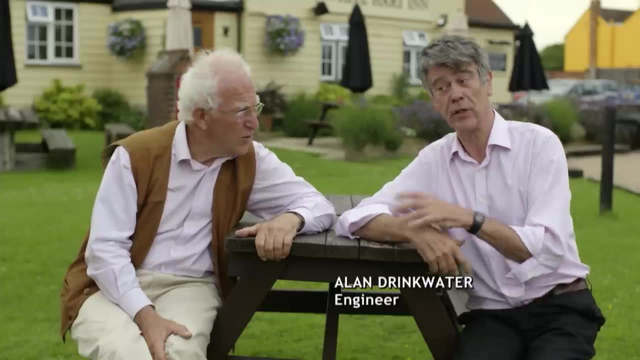 used to come to us and say, my, isn't it clean, Isn't it wonderful, this clean environment you live in? I could take you to an old coal-fired power station. We're doing exactly what Tony and I used to do. 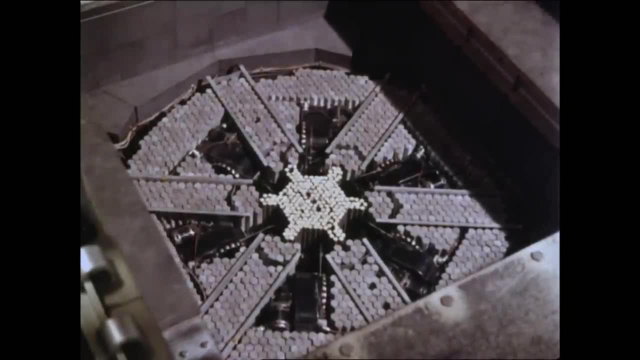 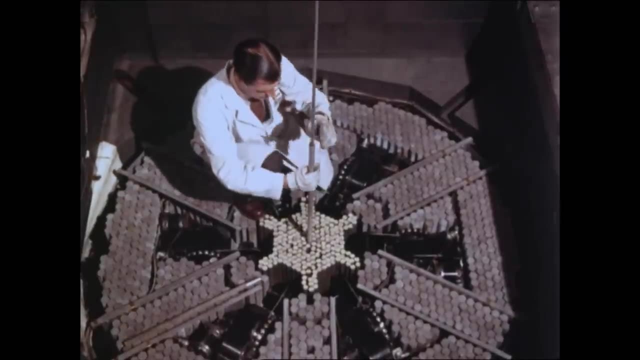 You'd come out black Across the pond. America's engineering giants were so enamoured with nuclear power they were ready to bet their wallets on it. What they did was to offer a fixed price or turnkey contract. All the utility had to do was to go to the reactor. 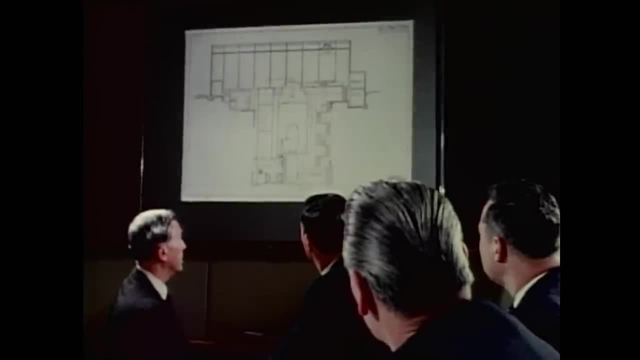 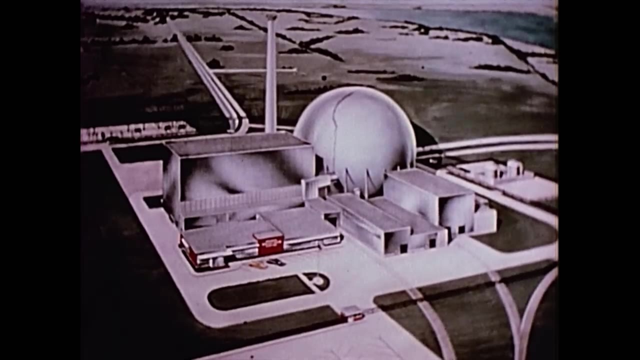 when it was built and turn the key and turn on the reactor, It seemed like there was no risk in building a nuclear power plant because the price was low and the vendors, Westinghouse and General Electric, guaranteed that price. And then comes the gold rush. 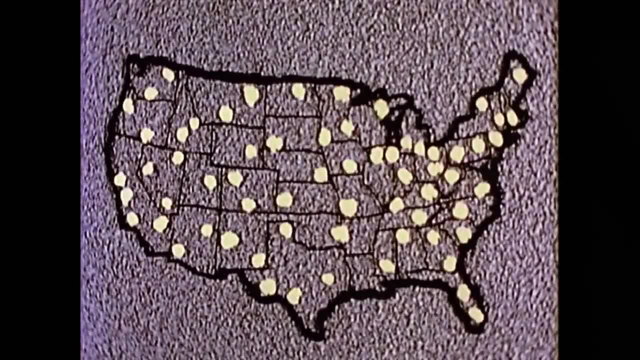 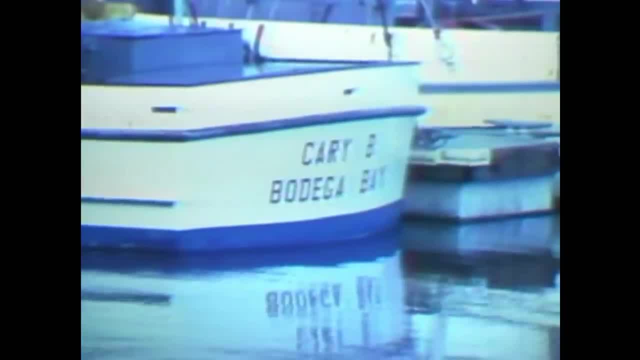 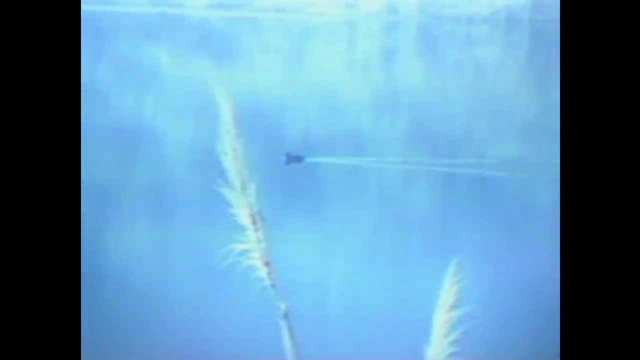 where everybody in the electric utility business is suddenly deciding, wow, we need nuclear power too. But not everyone is. But everyone was so enthusiastic I went down to Bodega- Bodega by the sea. There was a plan to build a reactor. 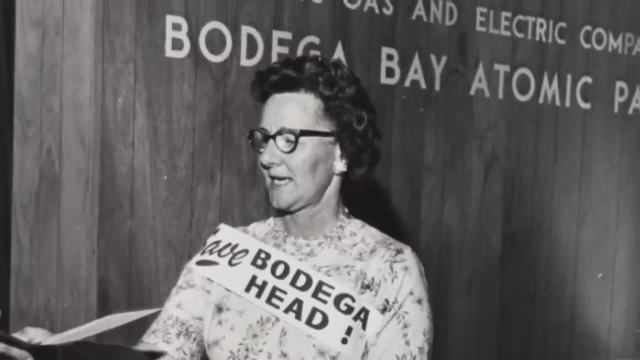 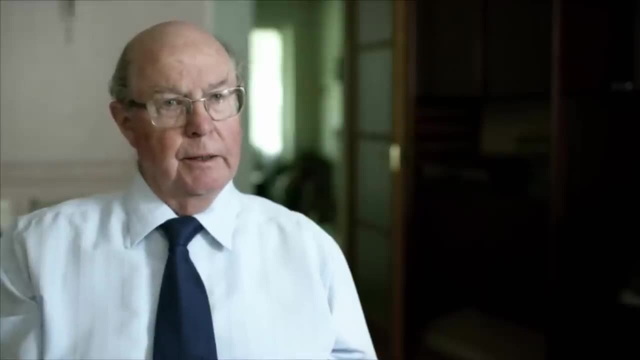 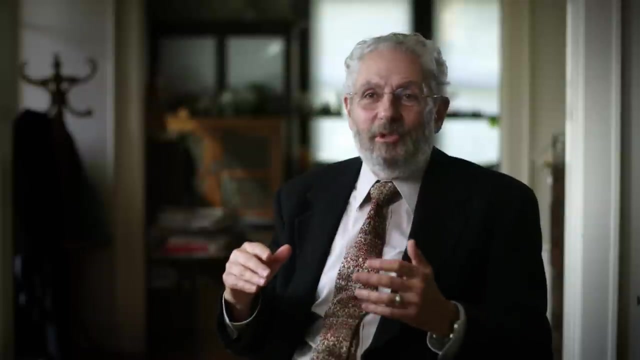 at Bodega Bay, California. Protests first started from local people who were just concerned about the view, But then people began to do a certain amount of homework and they began to get concerned by radioactivity released from the plant in normal operation. The local fishermen were worried. 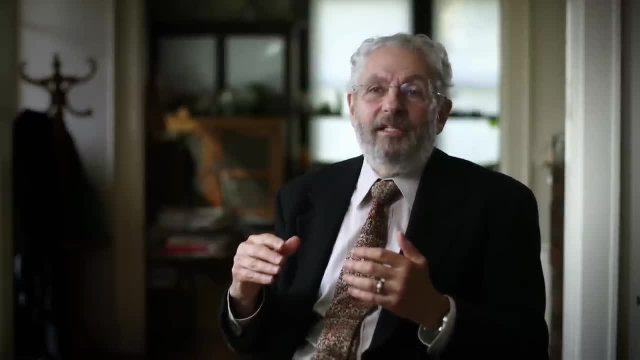 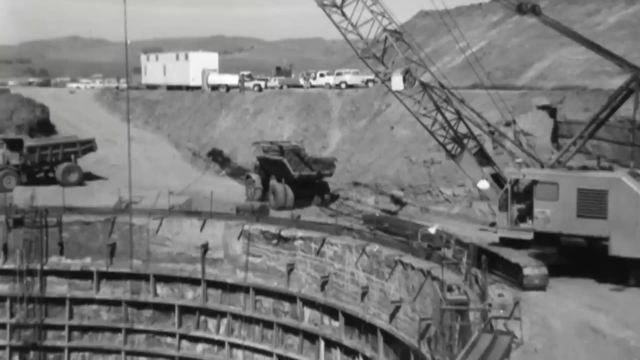 would we be able to sell our fish? Will people be worried about the radioactivity of it? There was also, more particularly, the possibility of an accident involving a nuclear plant, which might release a lot more radioactivity. I think that's an interesting thing. 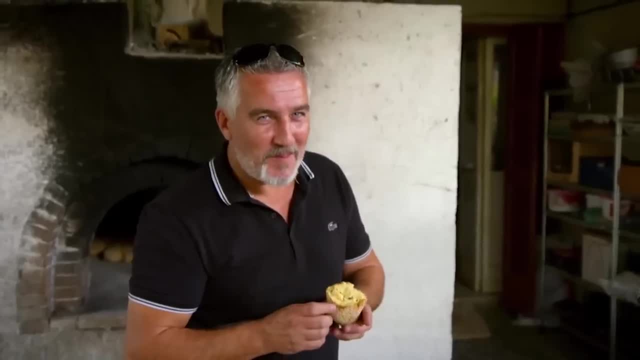 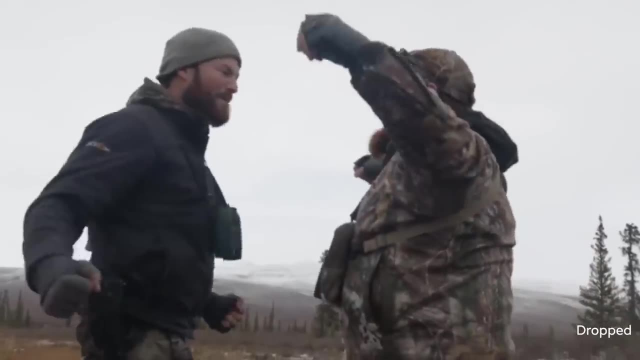 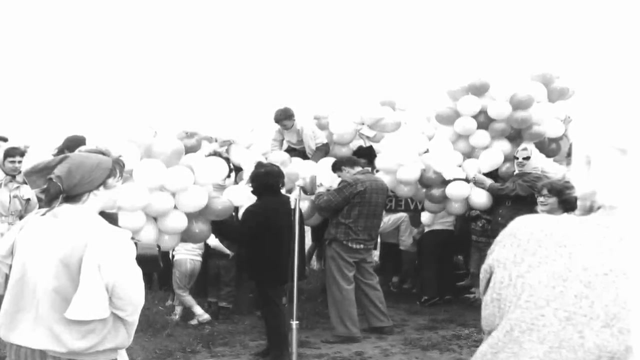 This one piece will make 52 layers Watch on mobile devices or the big screen. All for free, No subscription required. The most interesting stunt was they released a whole lot of balloons and when they came down they would have little messages on it saying. 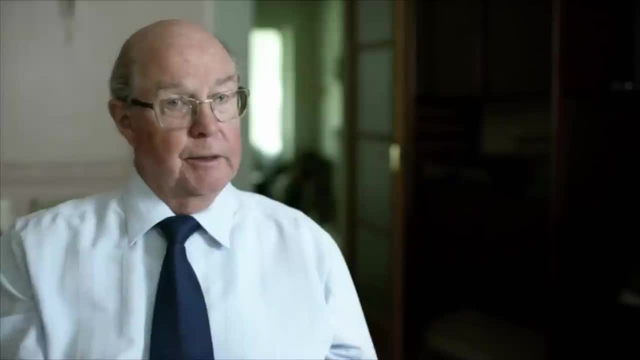 this could be radioactivity from the reactors. The public didn't in fact really know that there had already been a number of significant industrial accidents in nuclear installations in Canada, in Switzerland, in the US and in the UK. There was a very big fire at Windscale. 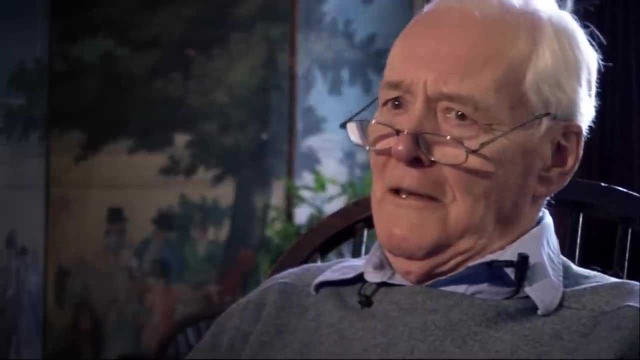 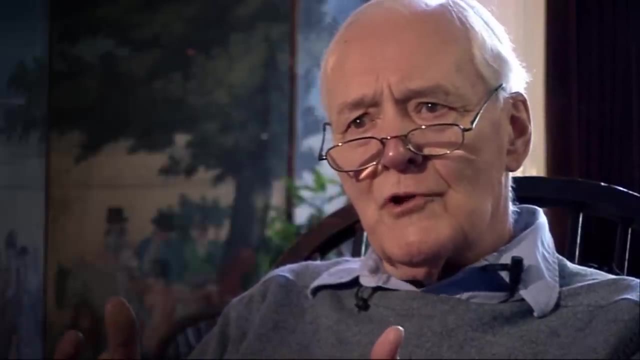 I was never told. I discovered when I went to Japan. I was talking to the Japanese minister and he said to me: how did? how are you getting on with dealing with the consequences of the fire? And I said to my officials: what fire? 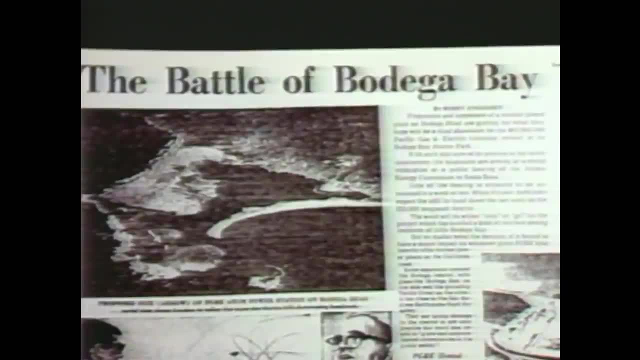 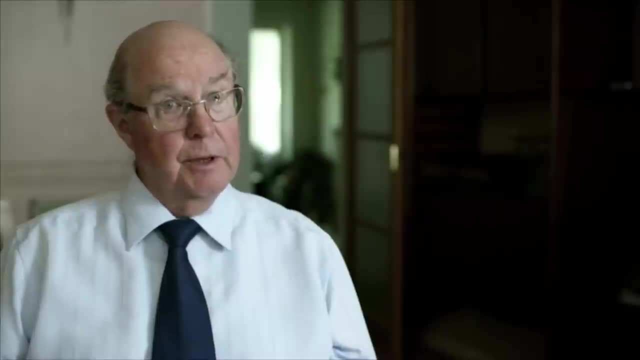 Oh, we didn't want to bother you, minister Bodega Bay actually persuaded the local electricity company to abandon the plant, And this was the first time that a nuclear proposal of this kind had actually failed because of opposition by the public, And it was going to be the first of many. 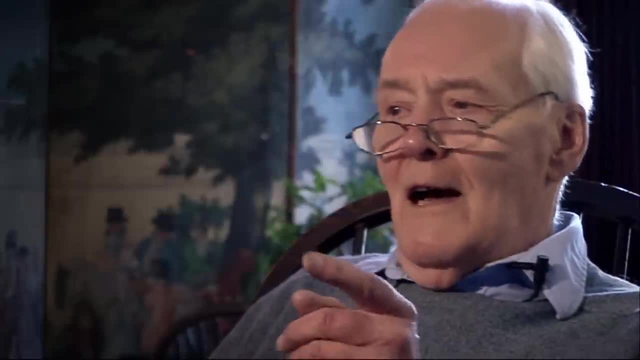 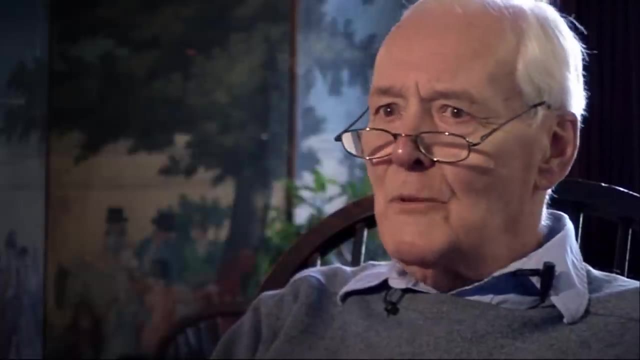 I remember when I first went to the States as a minister I was told that they had a policy of 2000-2000.. 2000 nuclear power stations by the year 2000.. But the local opposition was so strong that they couldn't build them. 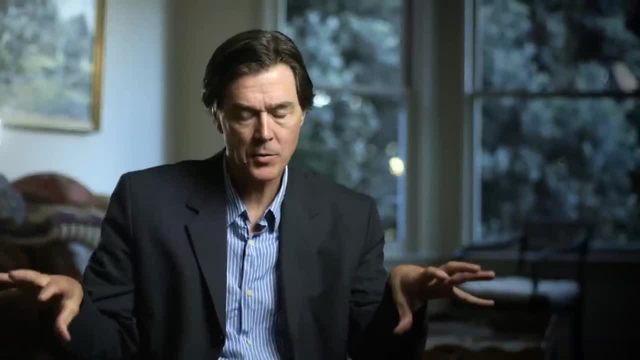 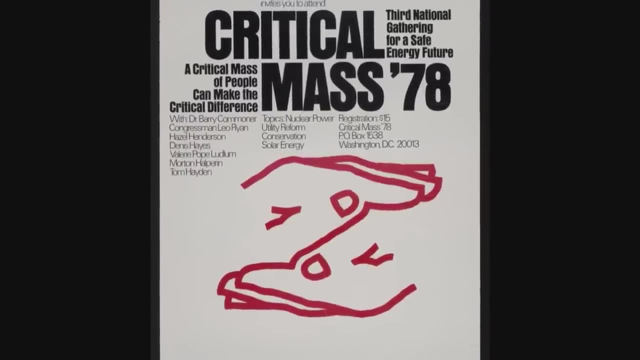 There were individual activists who were fighting individual plants around the country And then Ralph Nader called a conference, the so-called Critical Mass Conference, that brought together four people, 1,400 of these activists, and kind of gave them a way to see. 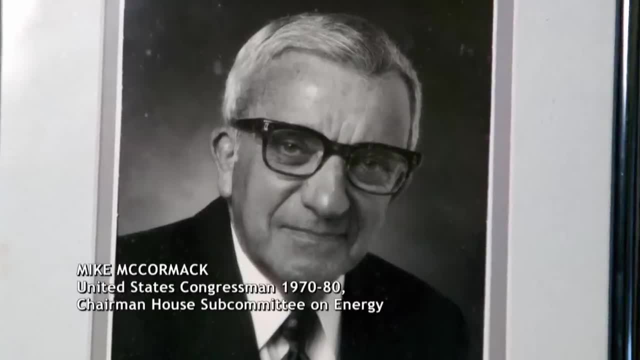 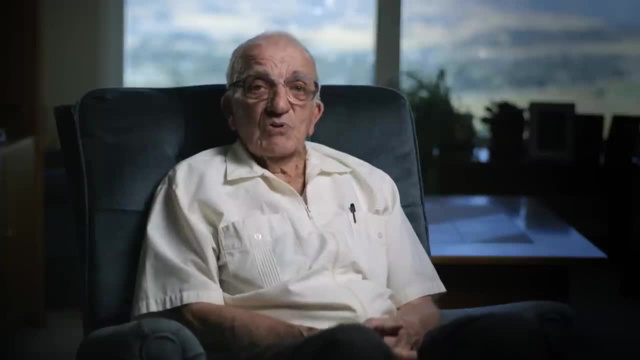 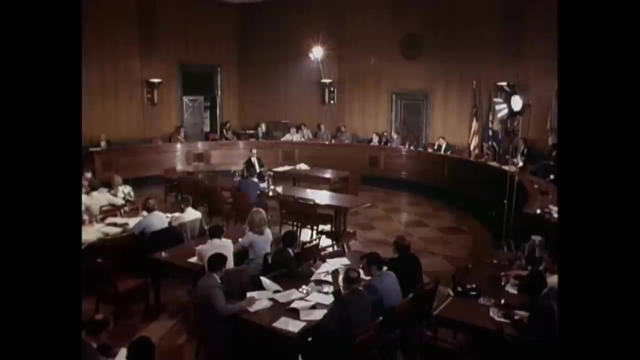 wow, we're not alone. It was frustrating to deal with what I had sometimes thought of as organized ignorance, And it was frustrating to deal with professionals like Ralph Nader who kept stimulating this sort of thing. The credible accident of one nuclear power plant catastrophe. 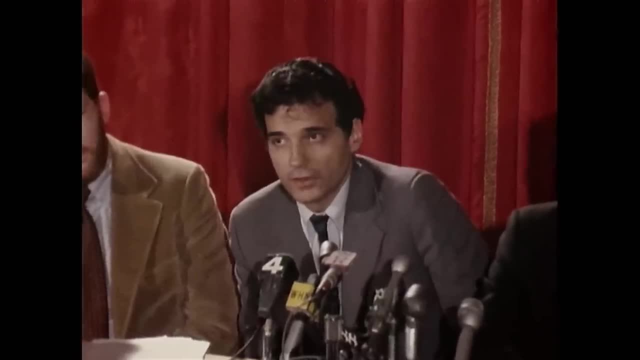 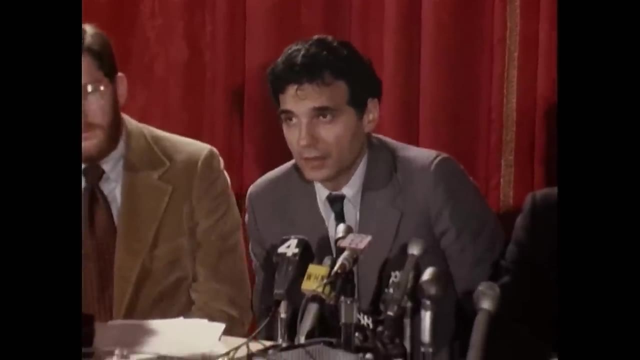 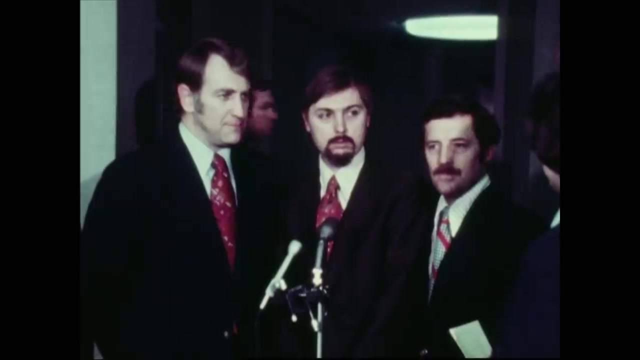 would be 45,000 dead and well over 100,000 seriously injured, $17 billion worth of property damage and an area the size of Pennsylvania contaminated. There were some nuclear scientists and engineers who helped this opposition. We had two marvelous general electric engineers. 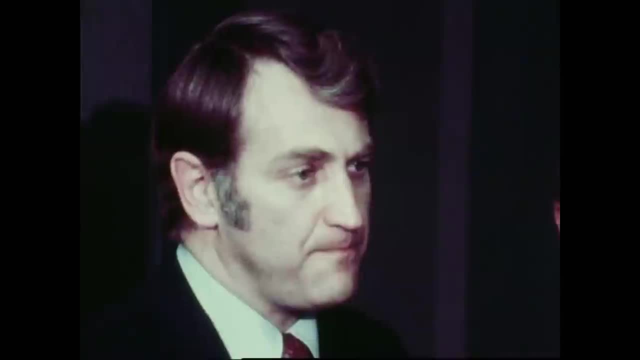 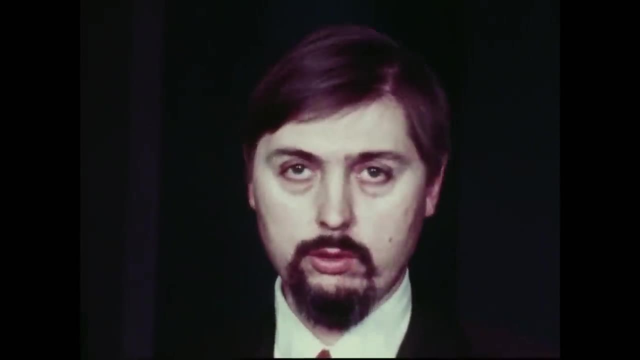 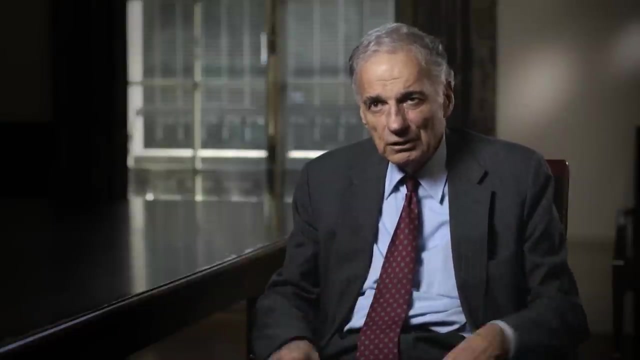 who quit and became whistleblowers. I testified on the NRC's quality assurance program that the quality assurance on a toaster is greater than that for the instruments that control a nuclear power plant. On the other hand, there was inadvertent support. The very pro-nuclear director 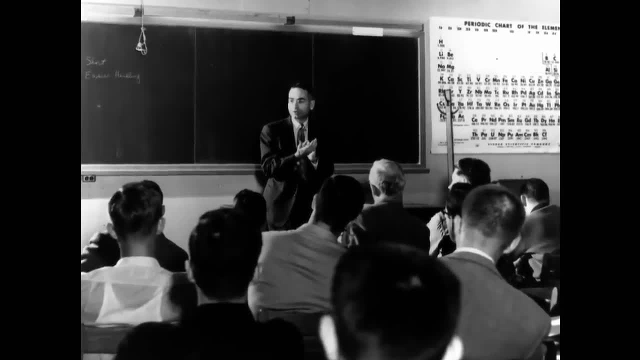 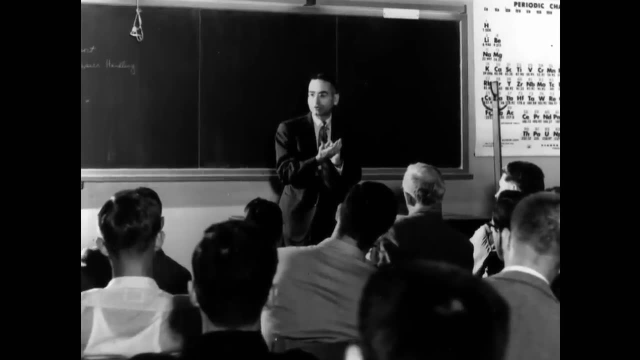 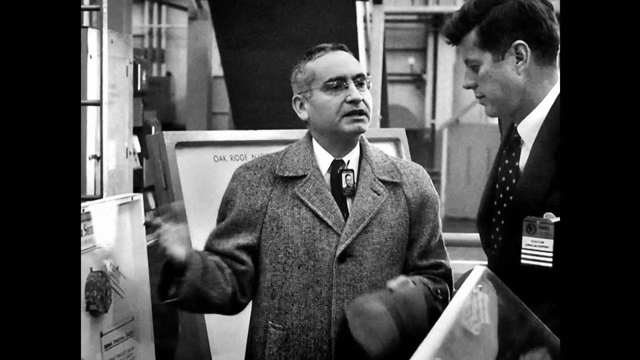 of the Oak Ridge National Lab, Alvin Weinberg, always harbored concerns. He thought that there shouldn't be one nuclear plant here and one nuclear plant there, that it would be better if we had six in one nuclear reservation, so that you could use what he called. 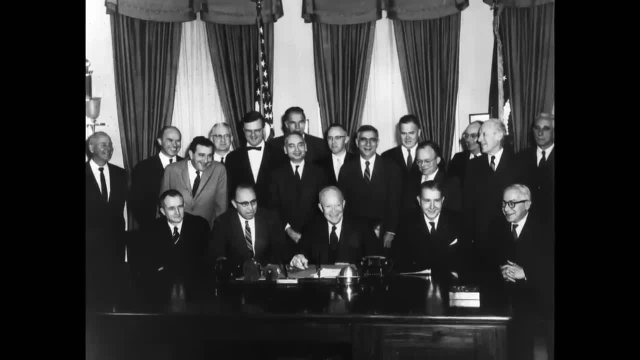 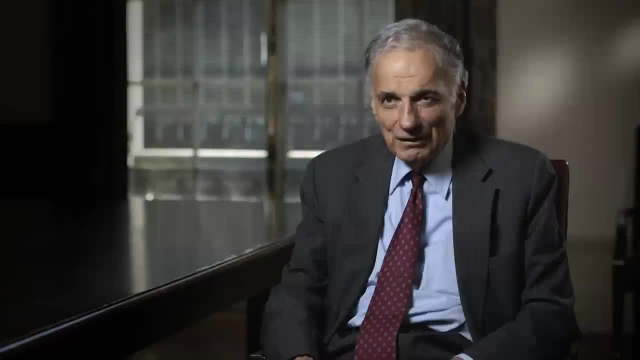 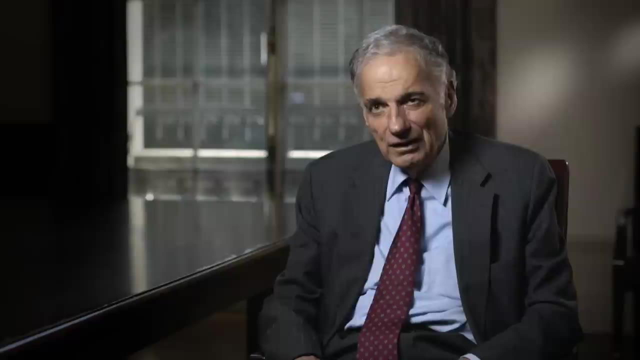 the small number of very competent scientists and engineers to manage it. He knew what the risks were. But at one time he said to me: you know, you're asking all of us nuclear scientists and engineers to do Ralph. And I said what? 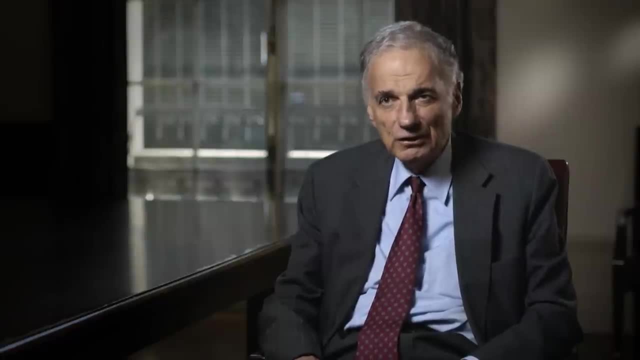 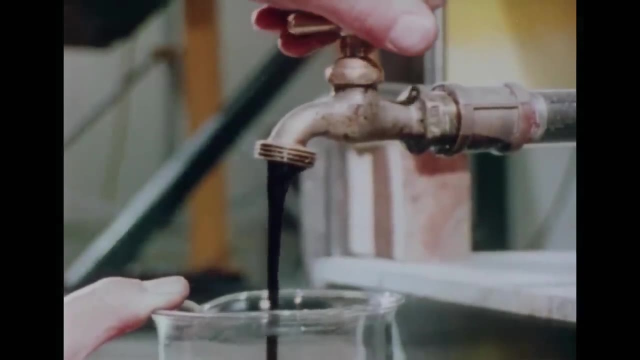 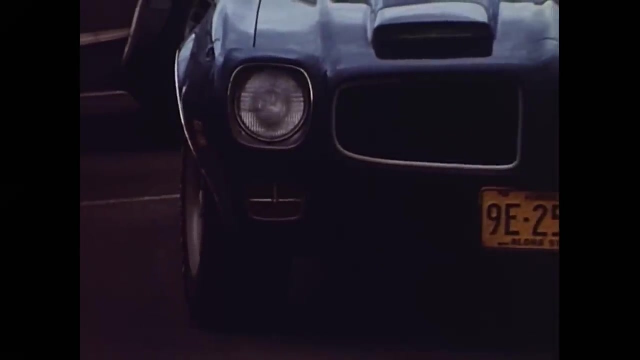 He said, to give up a lifetime of knowledge and their career, and that's very hard to do. But just as the opposition was growing in confidence, global events suddenly made nuclear power look a whole lot more appealing. In 1973, the big Middle East producers 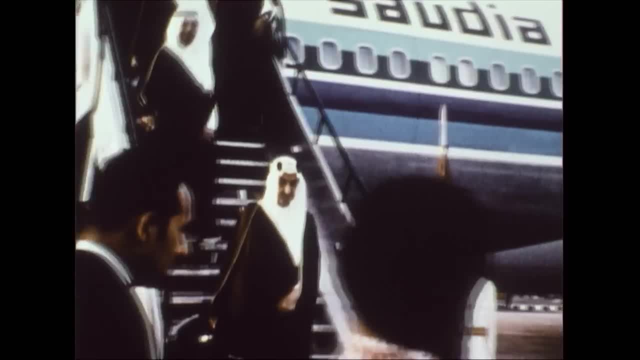 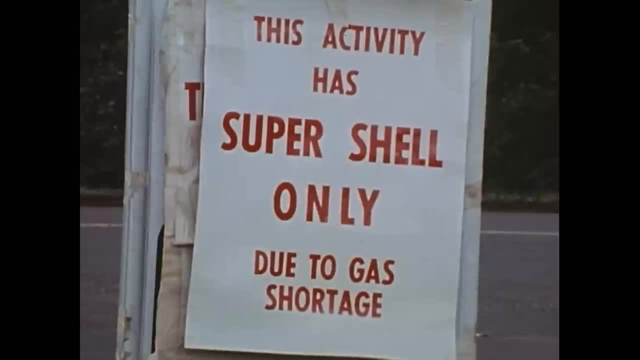 cut off oil shipments to major consuming countries. When the embargo was lifted, the price of foreign oil had jumped from $3 to $12 a barrel, four times higher than before. This nation- in 1980, can have all the energy we need. 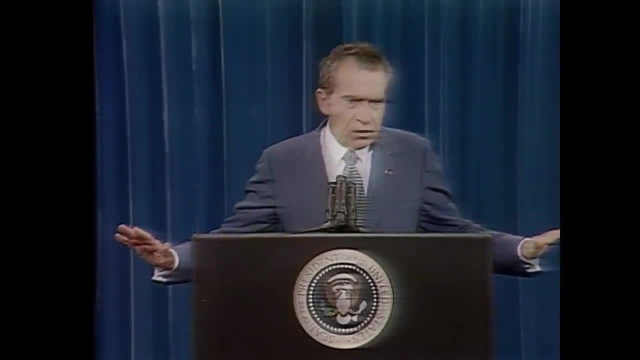 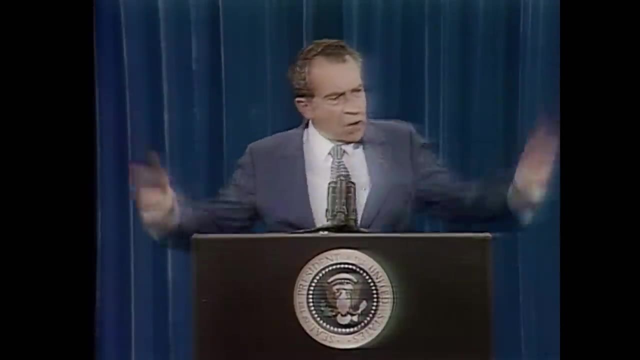 Now, don't write an editorial on this. You're really going to catch it from your readers if you do, because it scares people. Nuclear power: They think of the bomb, They think of the possibility that one of them is going to blow up. My house in San Clemente is just 12 miles from the Southern California Edison Company's nuclear power plant. It's safe, It produces good power, It's clean power, And the United States, which first found the secret of the atom, is behind, where it ought to be. 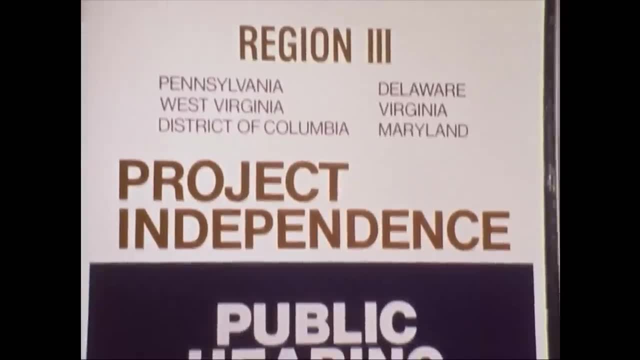 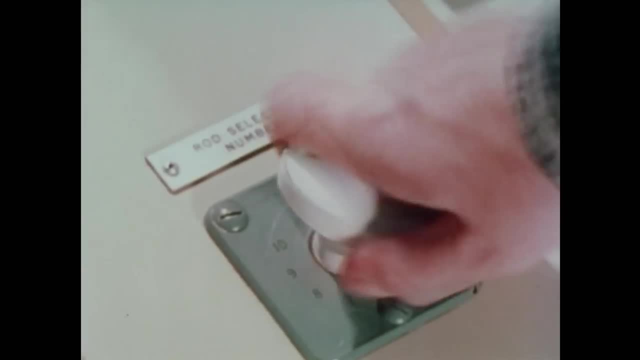 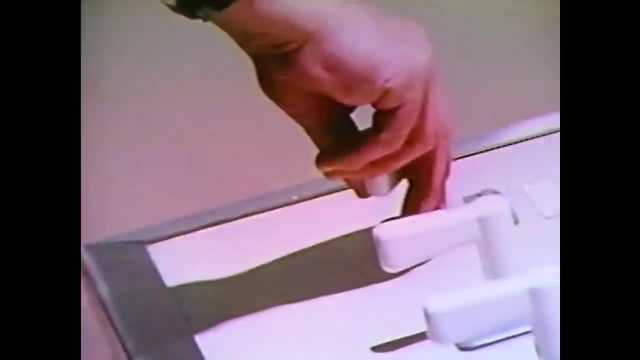 in the development of nuclear power. Nixon proposed a huge expansion of nuclear power In the name of getting America out from under the boot of OPEC. But even Nixon's support couldn't disguise one rather pressing problem. It became clear very quickly that the turnkey orders were horribly underpriced. The cost of every reactor and the nuclear power plant surrounding it. those costs were doubling every two years, Doubled and then it doubled again As the cost increased, as the cost of building reactors went up and up and up. they just couldn't afford it. It became untenable. The Americans may have been wondering if they could afford to expand their nuclear power program, But across the Atlantic the French couldn't afford not to. When there was the multiplication by four of the price of oil, the shock was quite considerable. 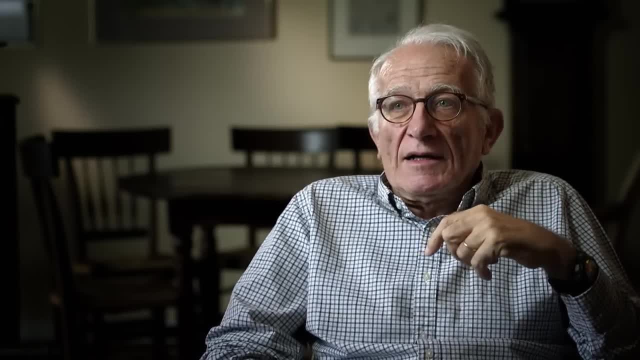 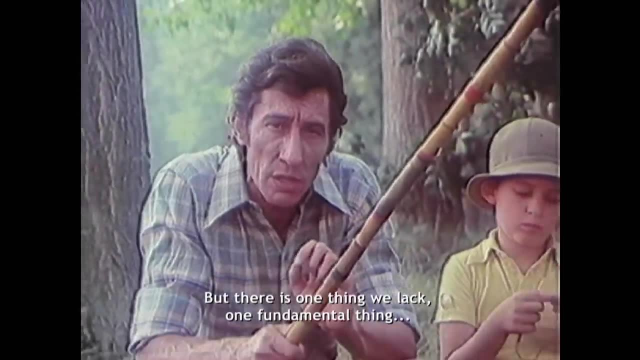 because 68% of our electricity was oil. There were very, very few countries that were at that point. In France, we have all kinds of things, Yet one thing is missing, One essential thing: Oil, Oil. we have to buy it from others. 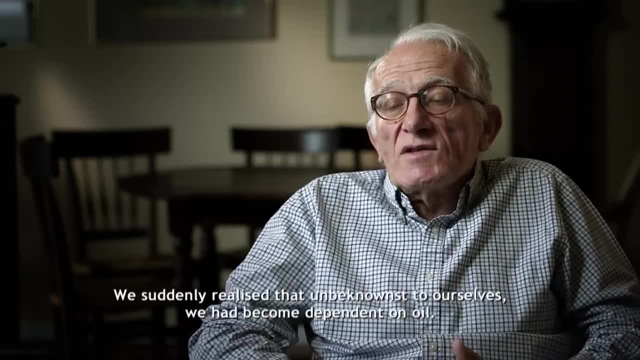 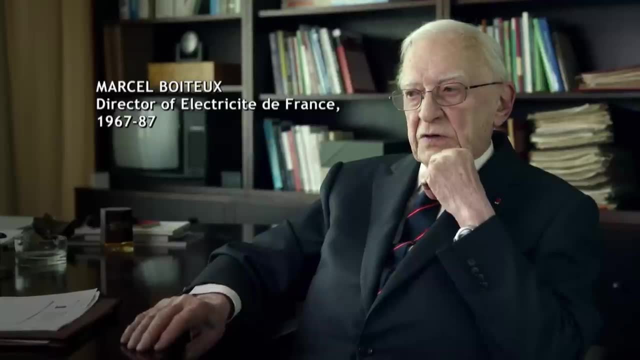 Expensive, Too expensive. All of a sudden, we realized that we had been addicted to oil without realizing it. But now it became unbearable. Yes, indeed, when the oil crisis came, it was clear to France that its salvation was nuclear. 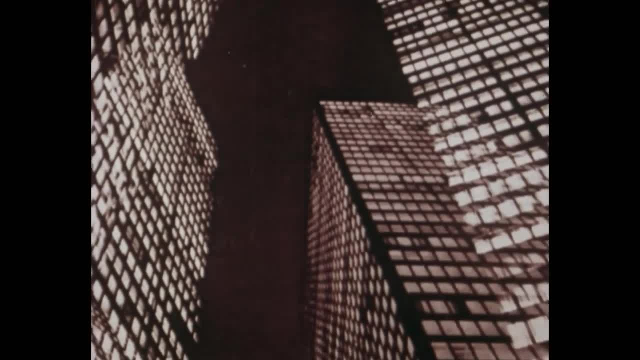 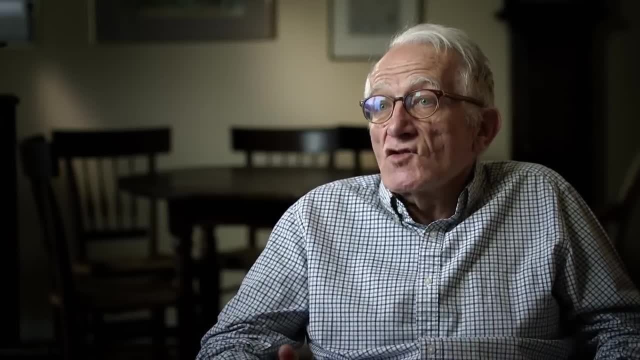 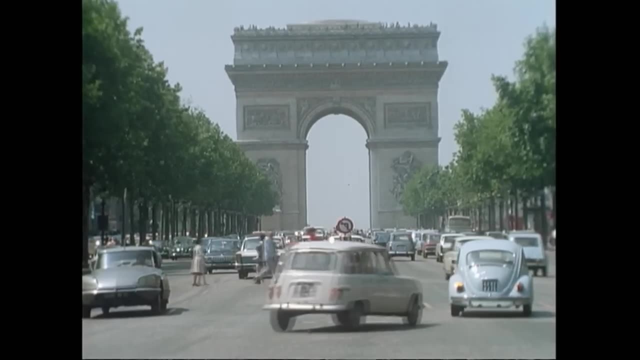 Why? Why nuclear energy? Because of electricity. The only place where we could easily replace oil was electricity. because in 1973, we already had a first generation of nuclear reactors. Spurred on by the oil crisis, the French government moved quickly. 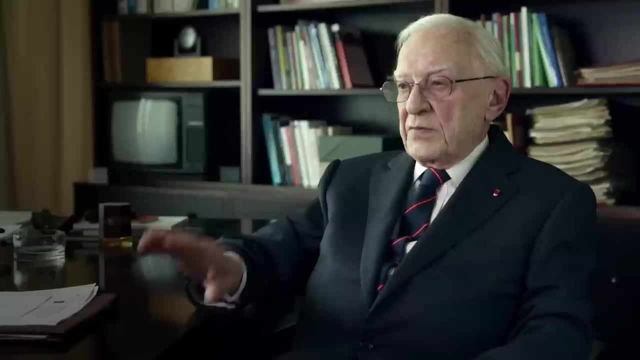 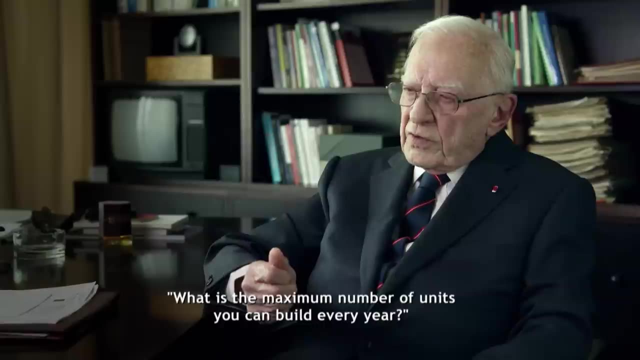 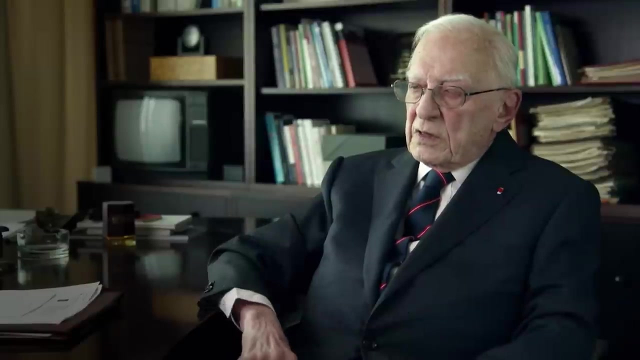 to ramp up the number of nuclear power plants in the country. On Saturday morning the energy delegate called me and said: how many centers, how many centers, how many sections? how many sections could be made at maximum in a manual rhythm? Three, four, five, six. 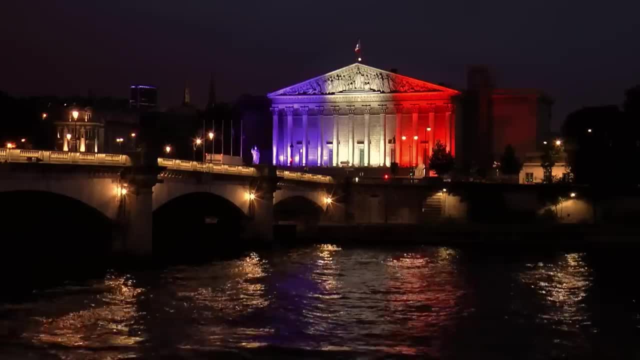 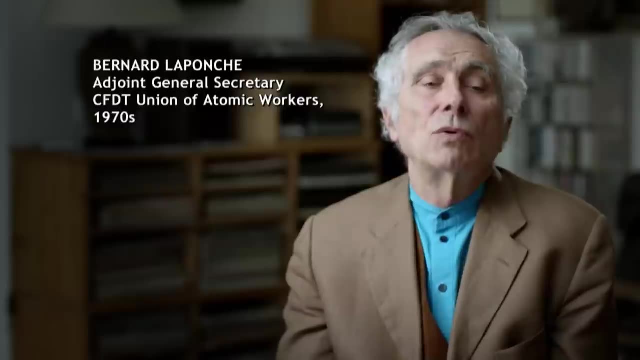 We did a whole camp to find out what we thought about it And finally we confirmed that it was six to seven And they didn't have to worry about what the public thought. Listen, from the point of view of decisions, it's a small group of people. 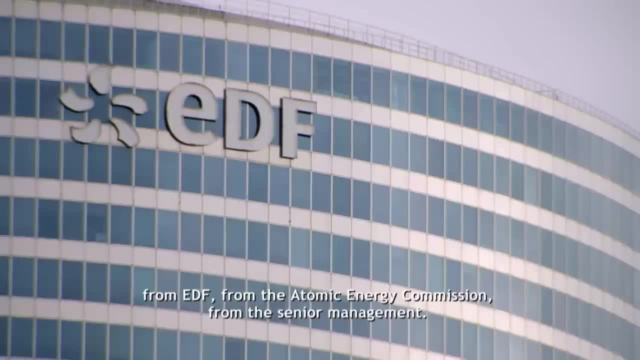 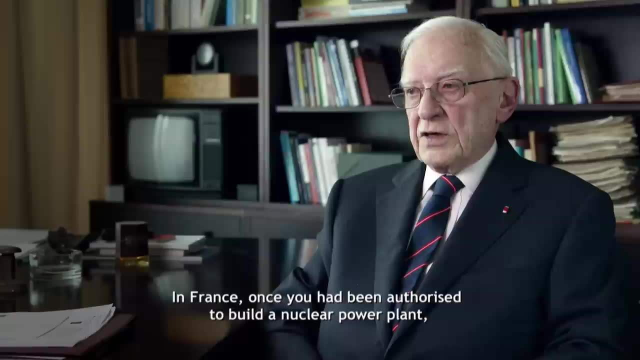 who are mainly dealing with the FDF, the CEA, the high administration, And it's the state that represents the people. It's very strong. In France, when we had received the authorization to make a power plant, it was over. 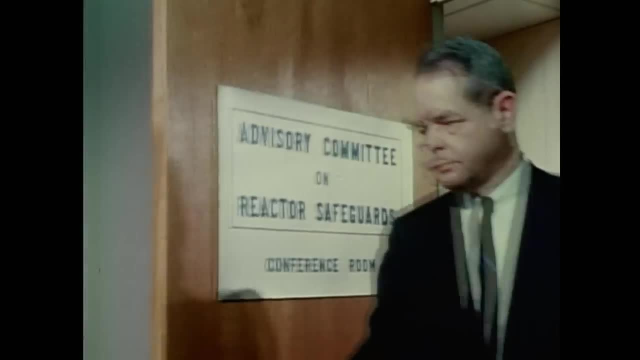 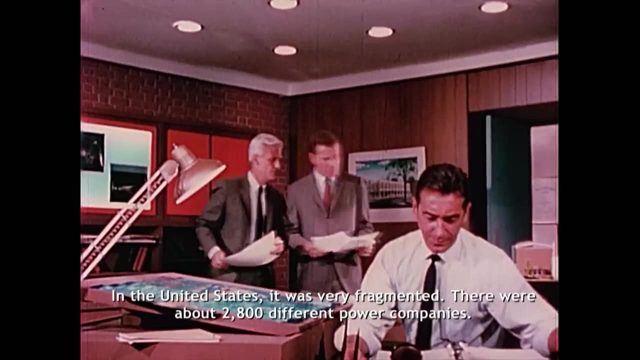 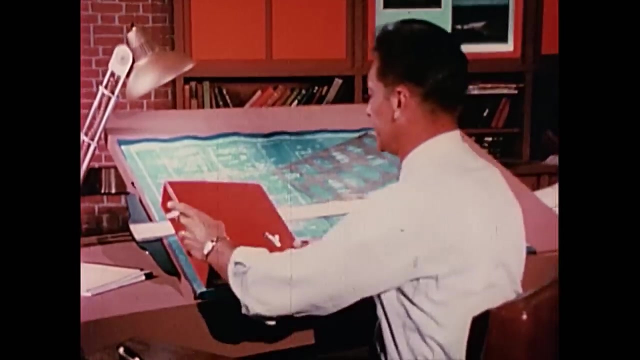 we didn't touch it anymore In America. things were more complicated. The United States was very fragmented. There were about 2,800 different electricity companies Out of 108 reactors. you had three identical ones And 101, all different from each other. They kept changing the designs in a competitive frenzy to try and get ahead of the other guy, And that meant that the construction times for nuclear plants just ballooned. Over the next two decades, the French would successfully embark on the most ambitious nuclear program anywhere in the world. The Americans could only look on and wonder. While the French were building 58 reactors, the Americans canceled 200 of them, And that's the difference. Meanwhile, France's next-door neighbors had their own problems to contend with In the 1970s. 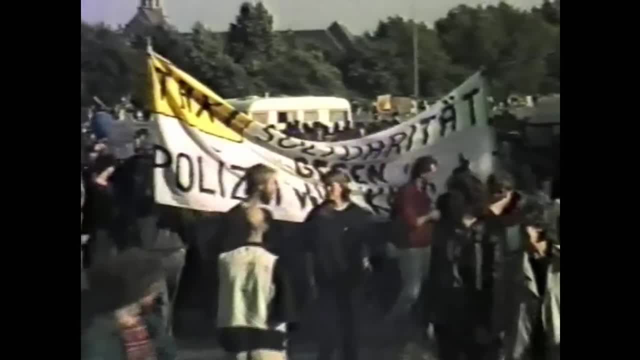 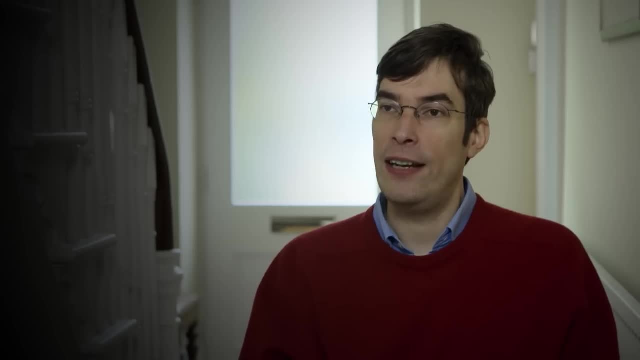 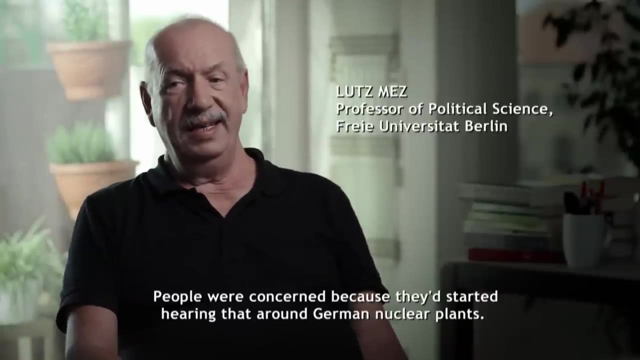 West Germany saw the growth of one of the largest movements against nuclear energy in Western Europe, possibly the world, And it was the first nuclear power plant in the world to be built in the United States. The concern was that one had already heard that there were inexplicable 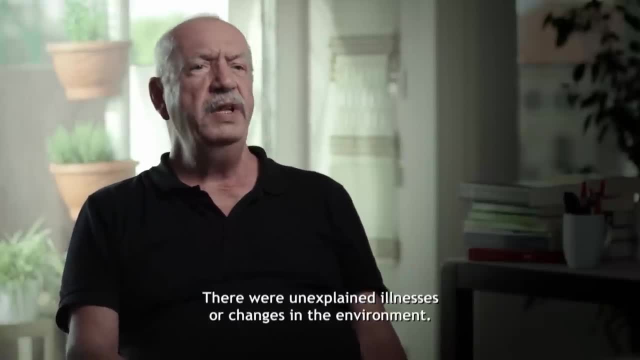 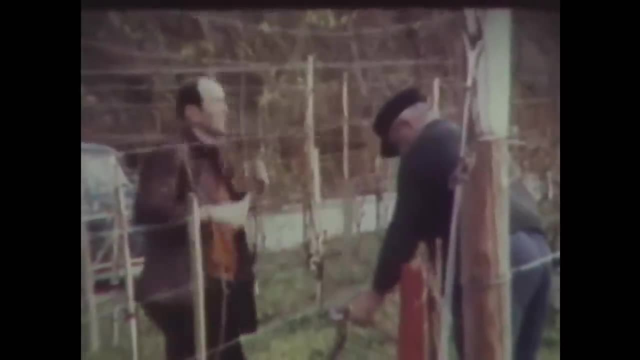 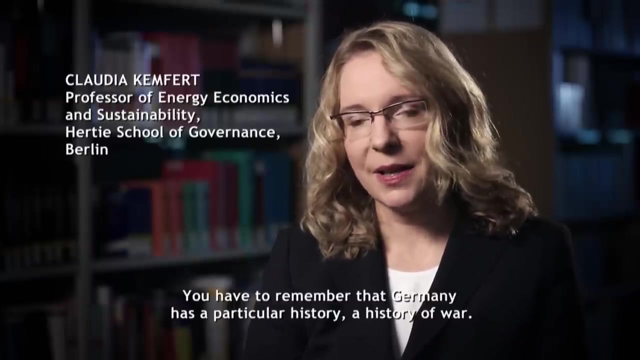 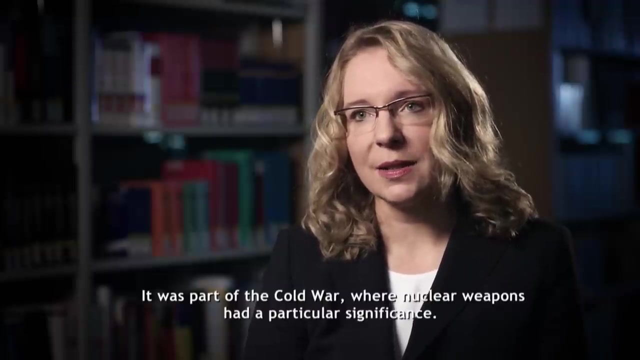 cases of disease or changes in the environment around German plants. You have to see, Germany has a history, also a war history, And it was part of the Cold War where nuclear weapons had an important meaning And we have major insecurity factors here. 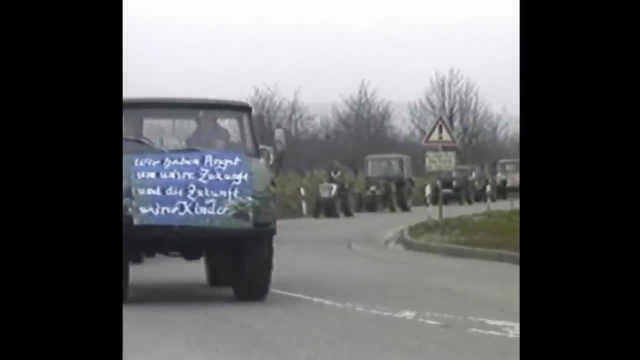 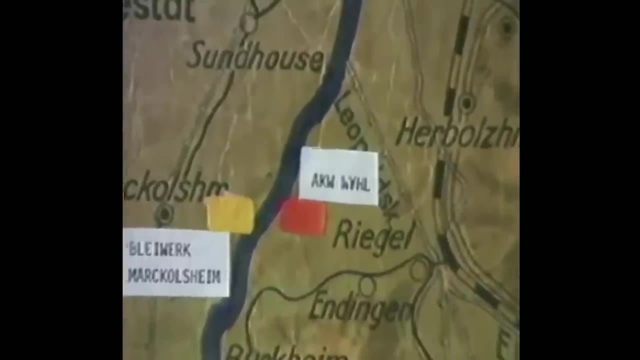 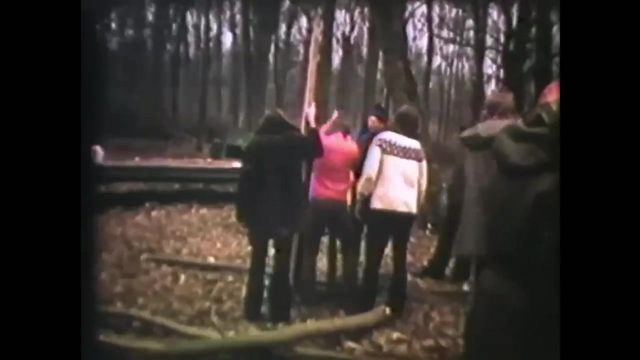 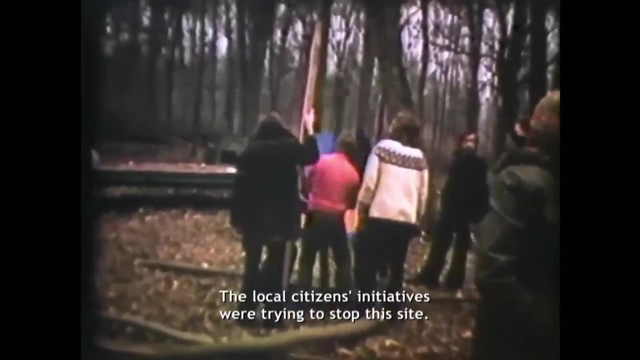 and they were reinforced by nuclear energy. The real point of origin: the protests in a very small South German village of Wiel, where a new power station was supposed to be built, And the local citizens' initiatives try to make this location as safe as possible. 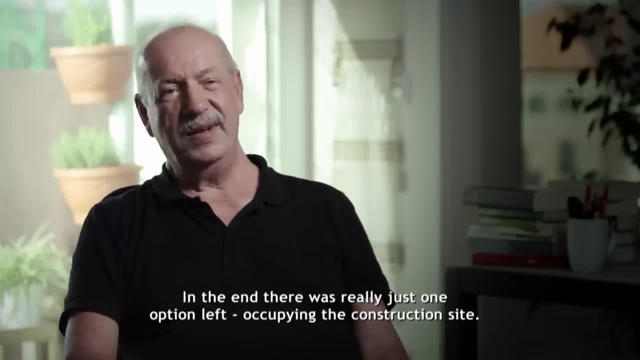 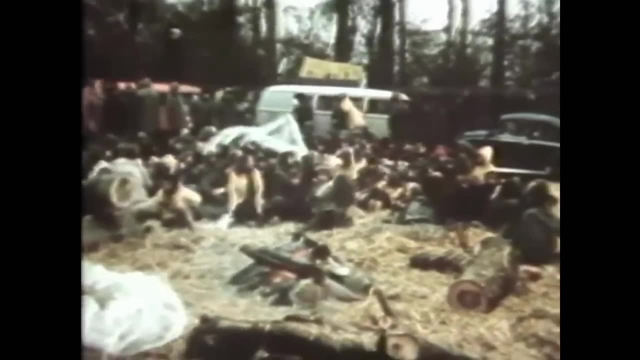 In the end, all that was left for them was to put the building down. They mobbed the site, They brought in tens of thousands of people- too many, really, for the police to handle- and set up a camp with a lot of guitar singing. 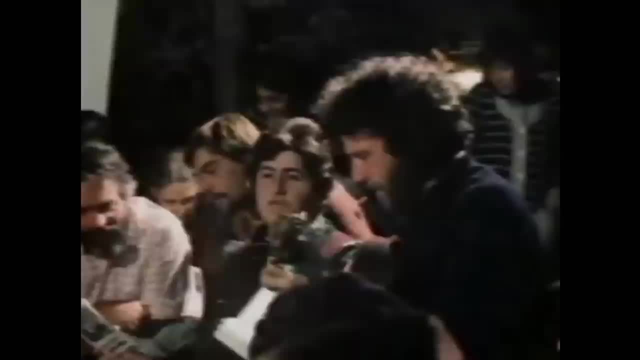 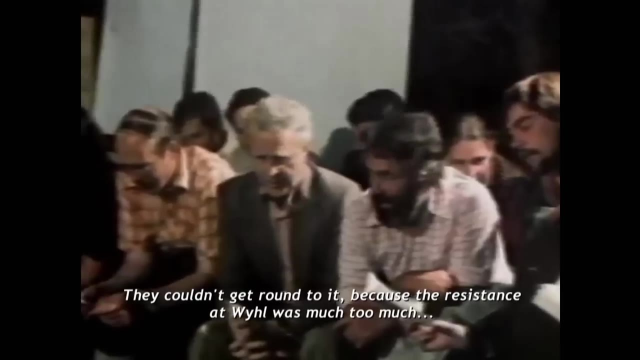 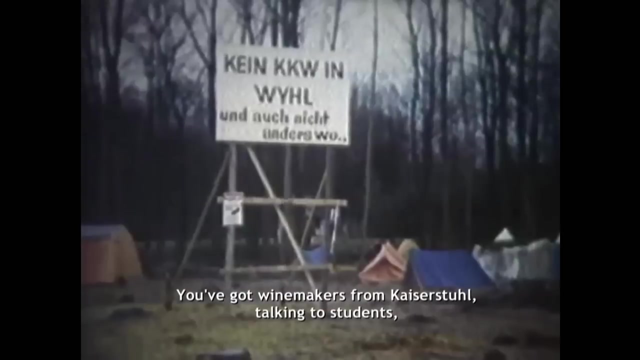 and public classes and free love and all that sort of a thing. They talk about how they wanted to put the building down, And what they really meant by this was to put a camp that it's not only for the police to hold the case for which the onlookers 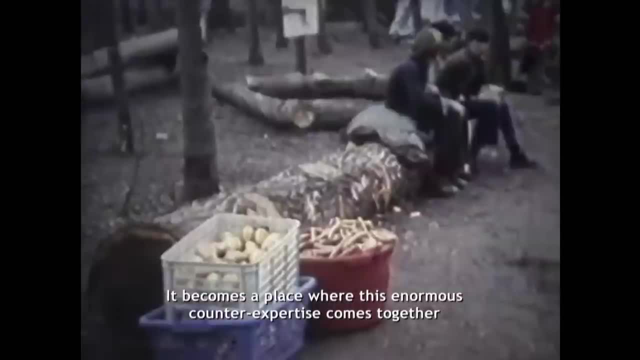 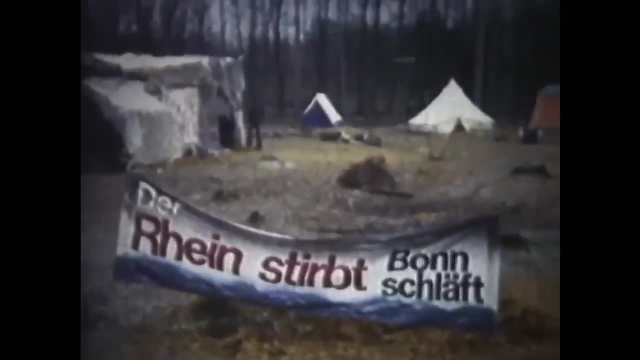 want them to put all the police to stand up and say, look, we need to stop the killing of the people of the city on the street. But Wiel's peaceful teachings soon gave way to far uglier scenes Wherever there were plans. 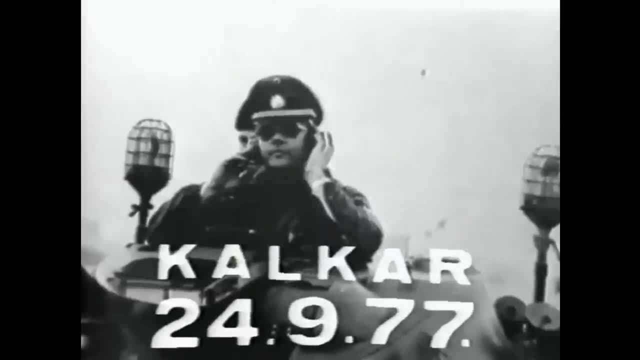 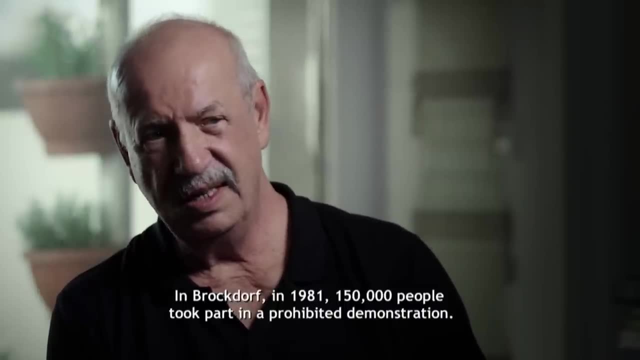 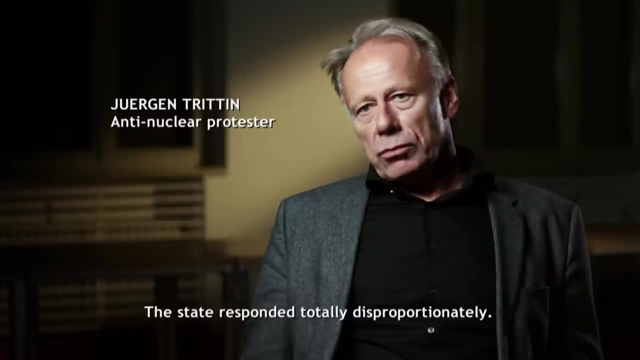 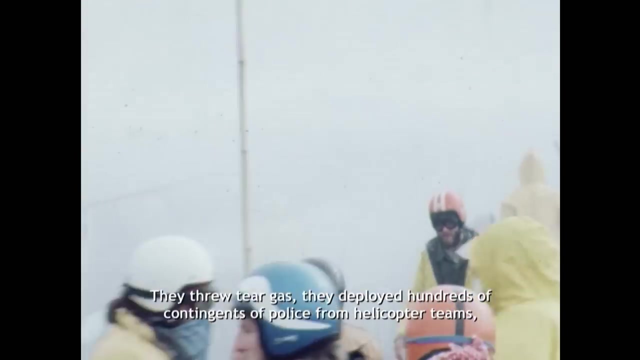 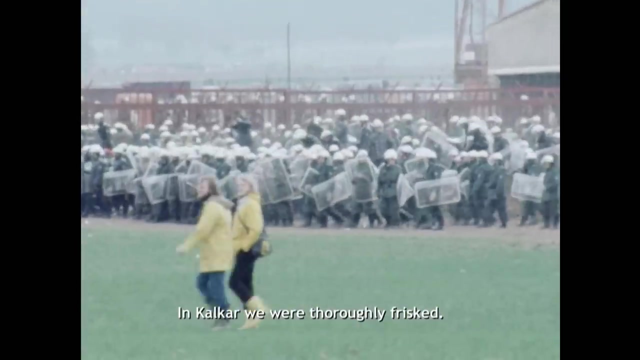 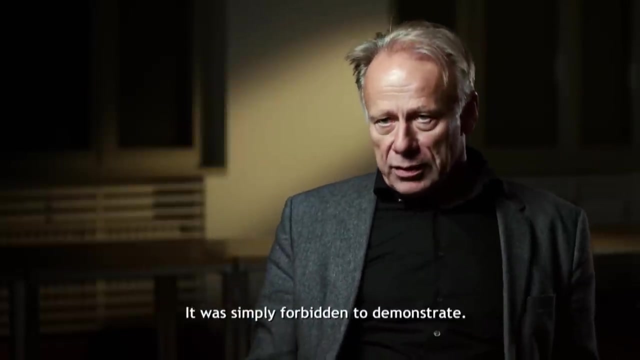 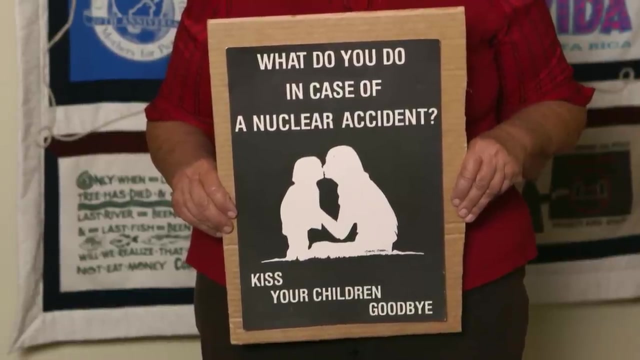 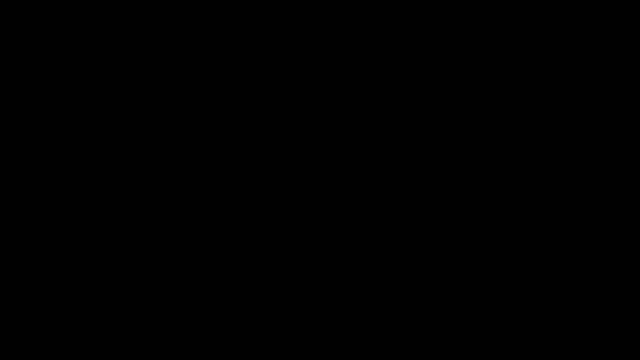 to build a reactor. there were huge protests and they often led to clashes with the police. Protesters on both sides of the Atlantic had been sounding the alarm about the prospect of an accident at a nuclear plant. fears the industry always dismissed Until one morning in March 1979.. 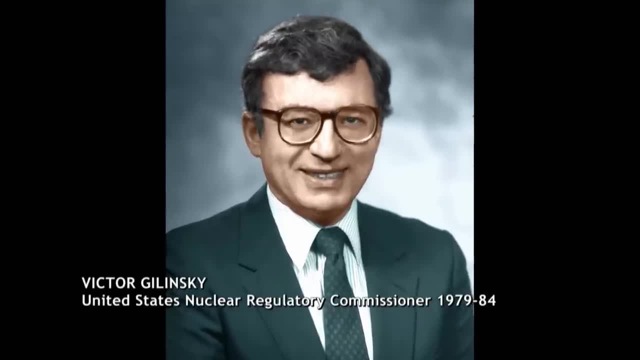 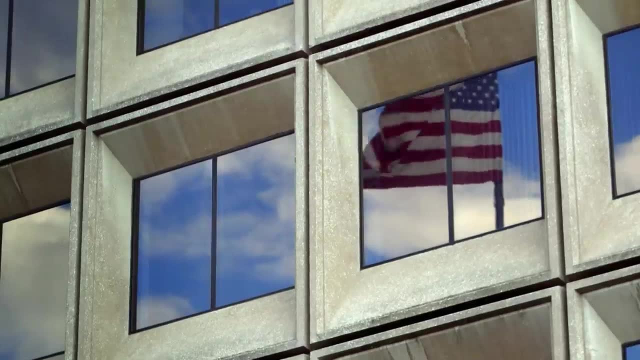 I came in to work and a commissioner went running by me, John Ahern, and he said: can I use your car? I said, sure I get upstairs. I discover that you know we've got a problem: Harrisburg, Pennsylvania, an accident at a nuclear power plant. 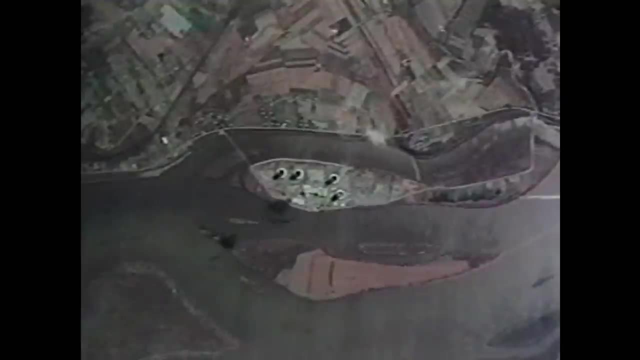 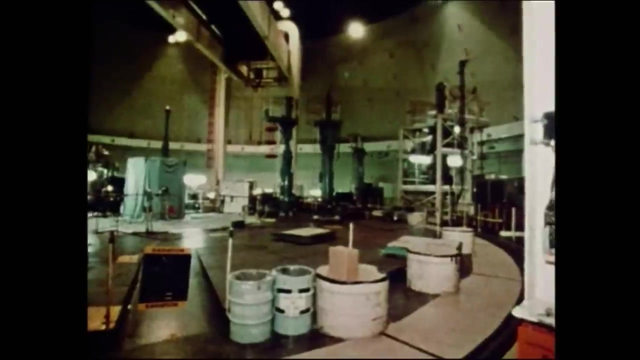 A spokesman said that a feedwater pump broke down this morning, automatically shutting down the three-mile nuclear power plant. People think that in an emergency everybody starts running around like in an operating room, you know. In fact, everything kind of got slowed down. 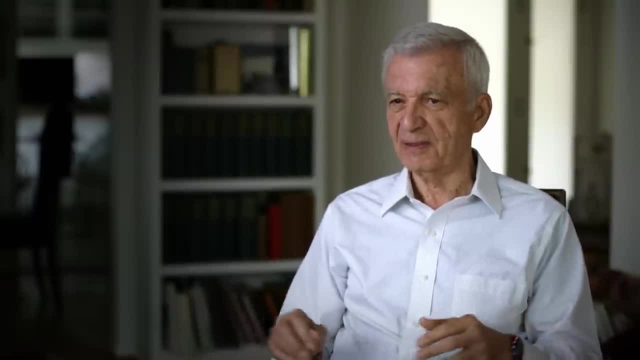 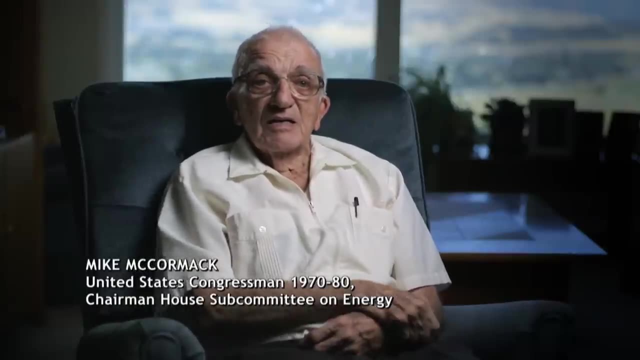 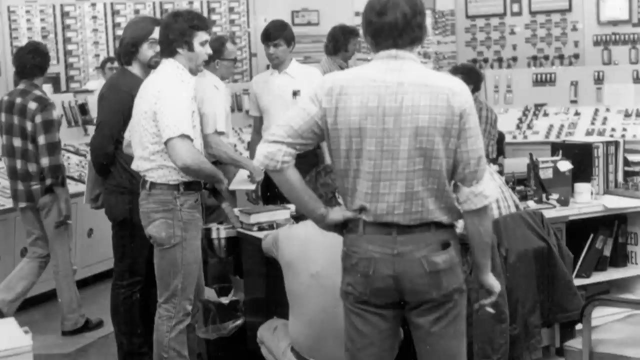 because you have tremendous uncertainty about the facts. I got a, a radiation monitor and I walked all around the entire plant reading the radiation levels And I found that the management in charge of the plant and the operators who were operating it were simply ill-prepared. 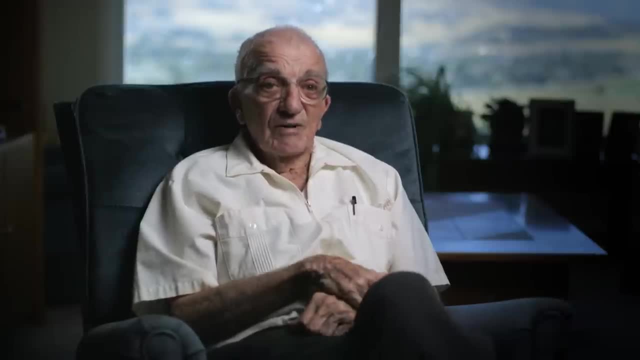 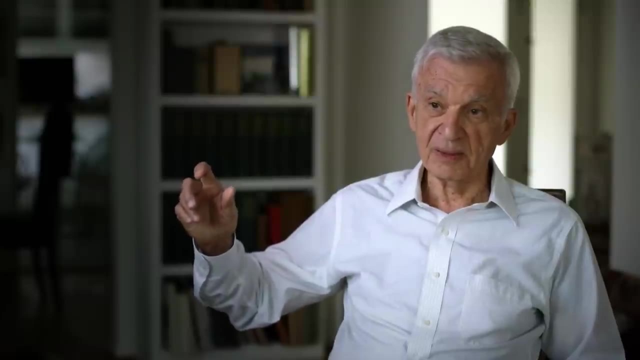 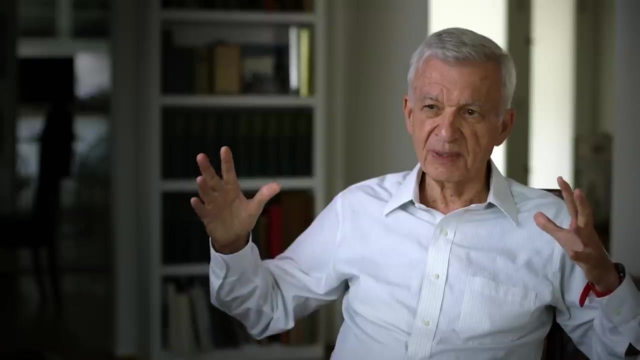 either to operate the plant or to talk to the public about it. The information was contradictory. Meters were reading very high, high radiation. Experts were saying these meters must be wrong. The overwhelming feeling is just the fog of information. you know, information fog. 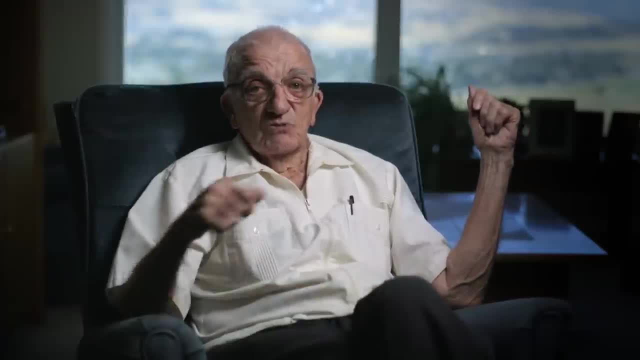 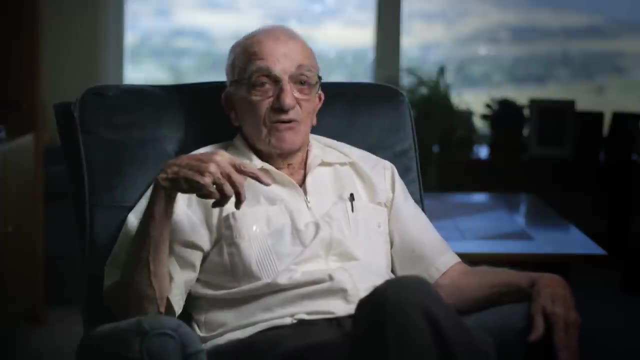 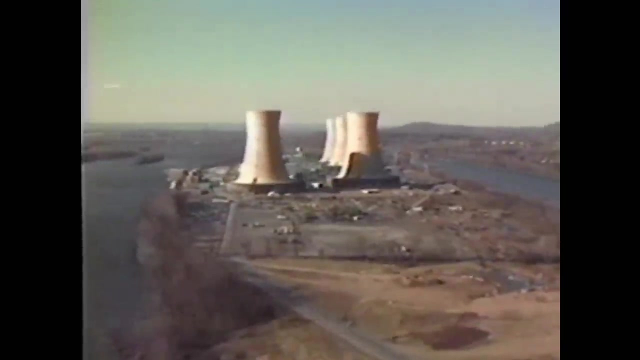 I remember Walter Cronkite closing off his news program that evening showing an aerial view of a cooling tower, saying I'm scared, There's absolutely no radiation about it at all. But that's what they were showing. I was on the set of Saturday Night Live. 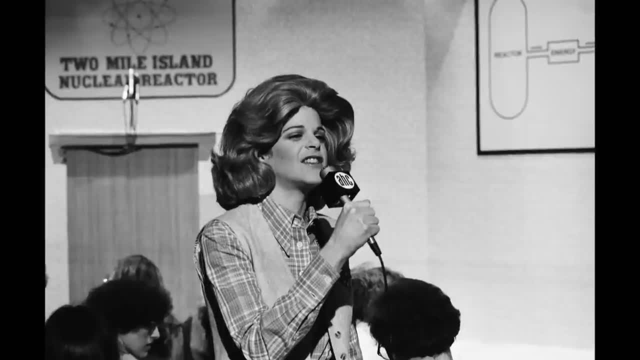 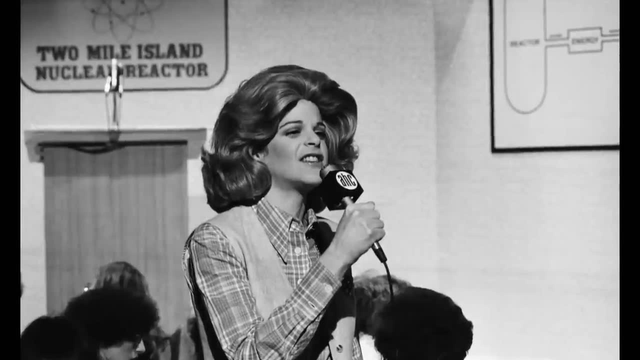 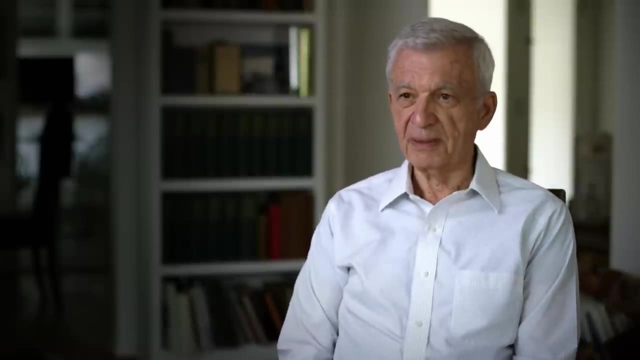 And Gilda Ratner, who's very famous, a very famous comedian, was very frightened and she asked her colleagues whether they were all going to die. But it scared the wits out of people in the eastern coast of the United States. It was very much unexpected and it was a feeling as if this was much worse than anything that one could have imagined. 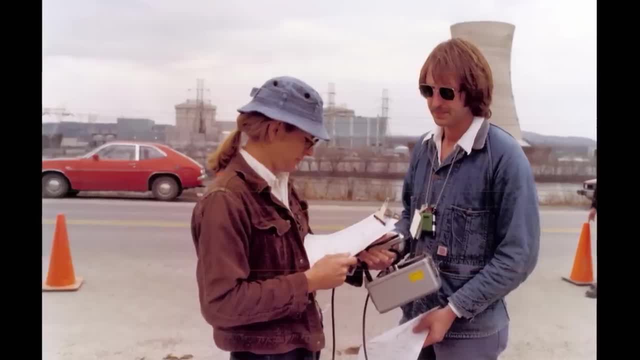 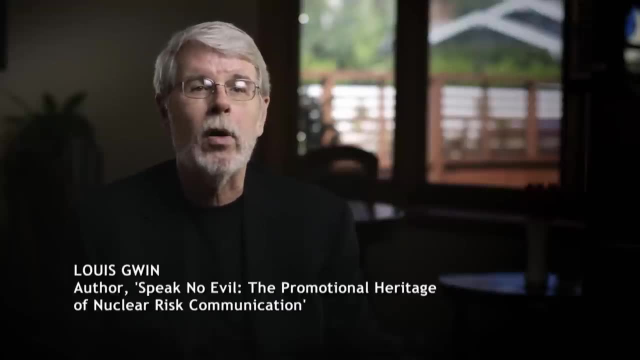 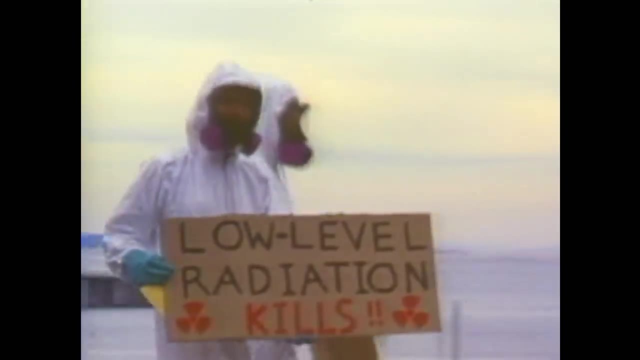 There'd been some near-serious accidents, but not one like Three Mile Island, And when that happened, I think the whole, the whole framework fell apart. It could no longer claim that nuclear plants were safe. That was a very defining moment. 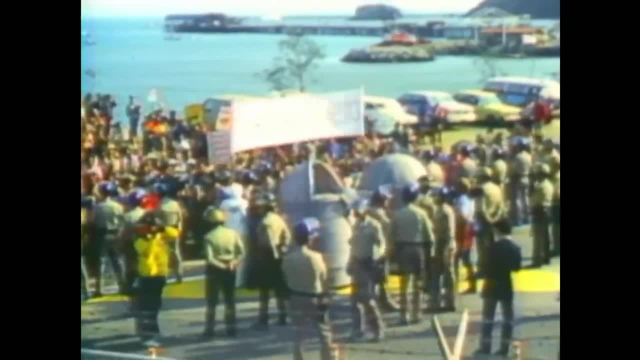 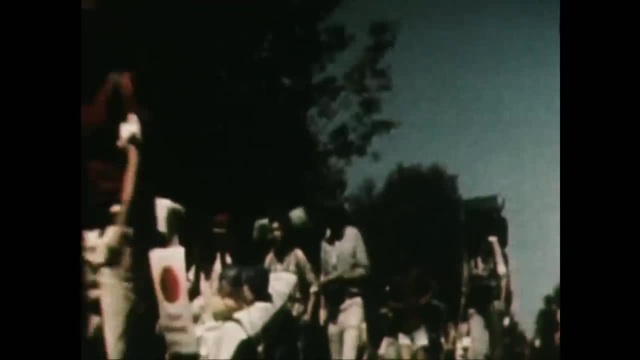 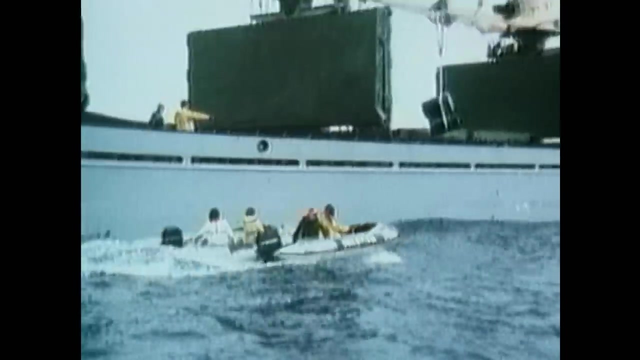 They're going to build them, even though we say no, They are the rulers. They say which way to go. We are the people, They are nuclear madness. Ha Ha Ha. Three miles Was only the start Of something bigger. 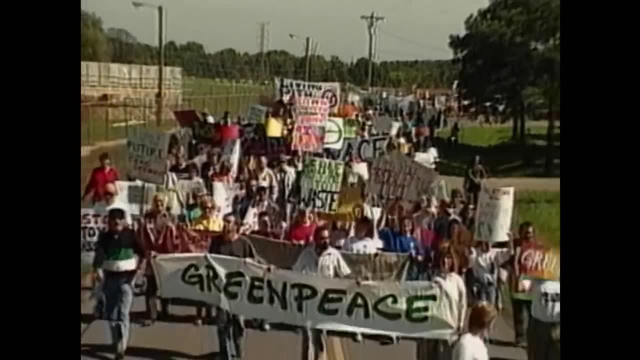 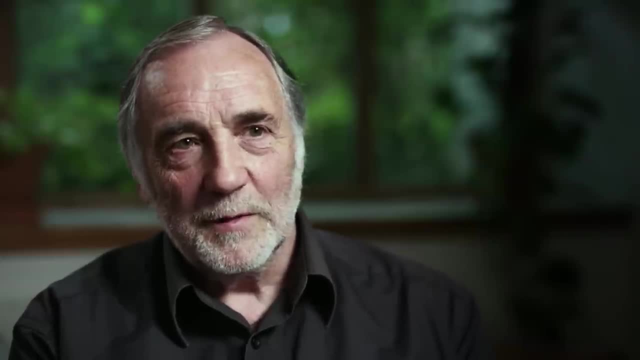 They're going to blow us apart. We are the people. I think that period of time left us with a scorecard of about 4-0 in favor of Greenpeace. to be quite honest with you, Greenpeace were activists, true activists, and that was a new problem to deal with. 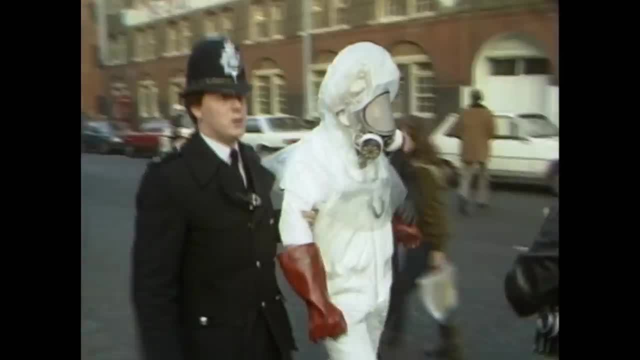 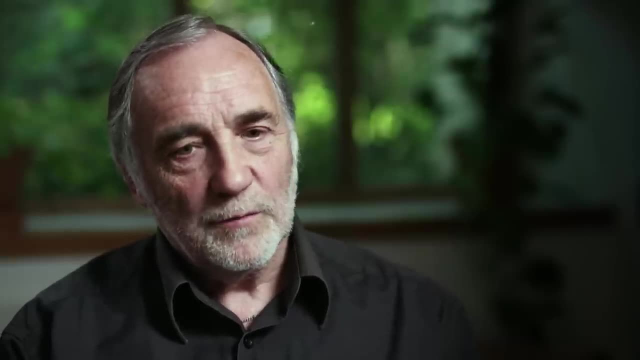 In the 80s we had this sort of this inevitable march towards a nuclear future and at the same time, we were looking forward to the future at the situation where there was this wheezing puffing plant at windscale and which was pumping. 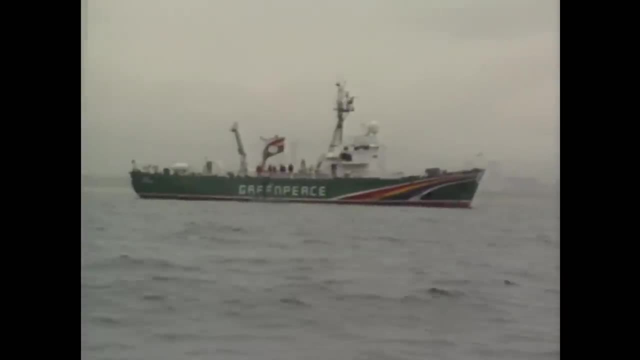 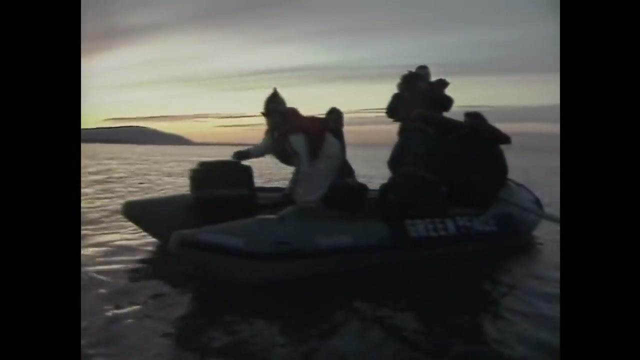 out two million gallons of contaminated material into the irish sea every day. i mean the whole thing was just a joke. i mean it really was and we had to address it in some way. at first light greenpeace were already up and about. their plan was simple: to block the one and a half. 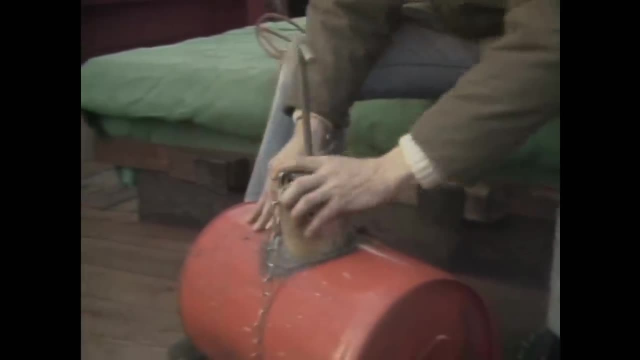 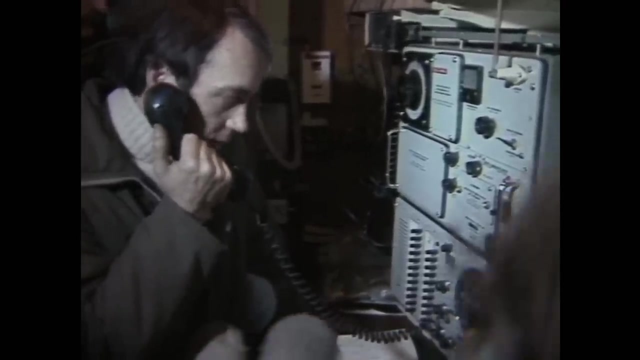 mile long discharge pipe with stoppers like this one. i held a confidential briefing with the press and i said: you know, we're going to bung the pipe up. we have bungs ready. we are going to stop the discharges. and somehow that got leaked and bnfl then knew that we were going to do it. 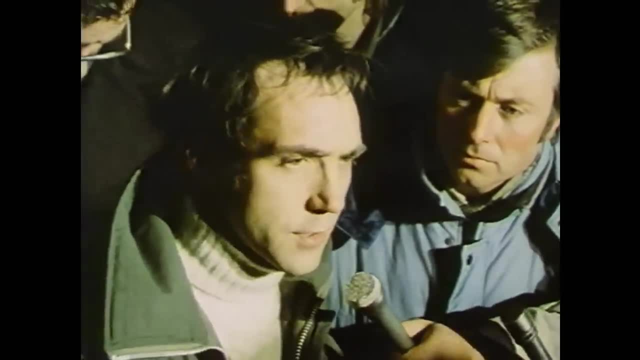 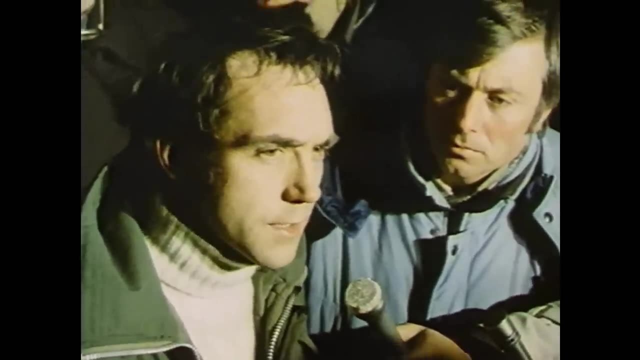 right at this moment. british nuclear fuels have beaten us to the punch. they've obviously known precisely what we've been going to do. for the last week or so they've worked very heavily on this pipe and it's impossible for us, with the material we've got at the moment, to block the pipe. it was. 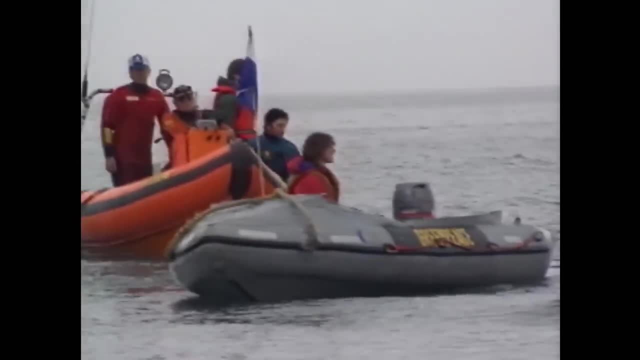 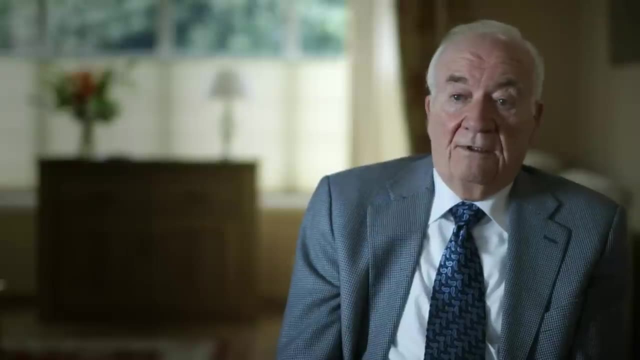 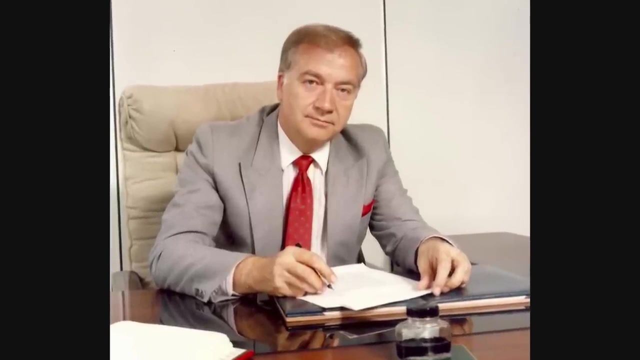 a balancing act, always to try to deal with them sensibly, but in the end, to use the law if necessary to stop them doing things which i felt were dangerous. they needed to be told they were not beyond the law any more than we were, and so i was a baddie at times. public confidence was at an all-time low. 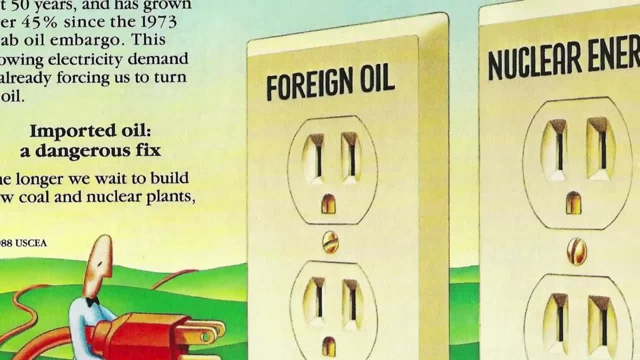 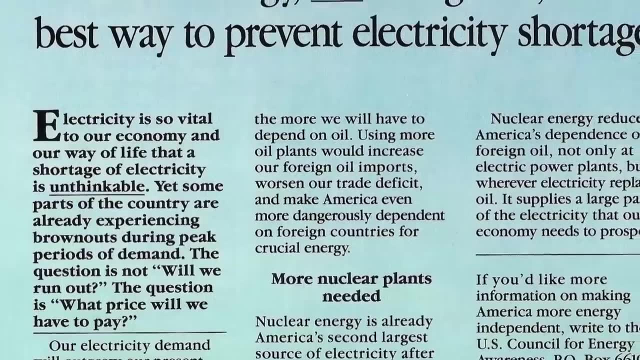 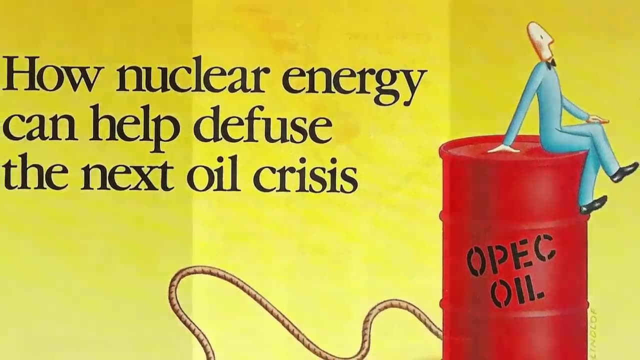 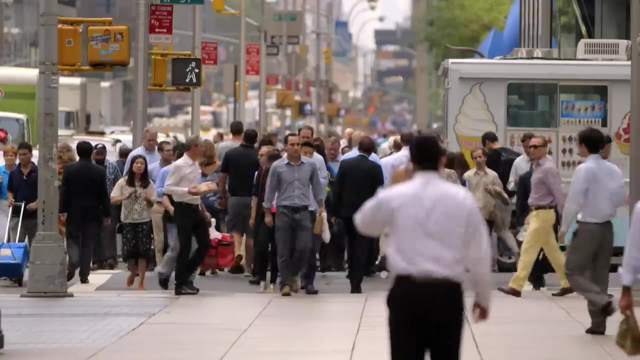 and yet the industry did not give up. they created an organization called the committee on energy awareness that was out there saying we need to stop our dependence on foreign oil, and nuclear power can do this. they deeply- and, i think, genuinely- believed in the nuclear enterprise. how could anybody turn against this technology? this is a miracle technology. 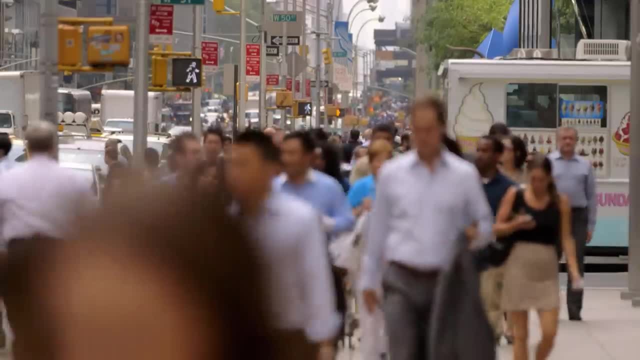 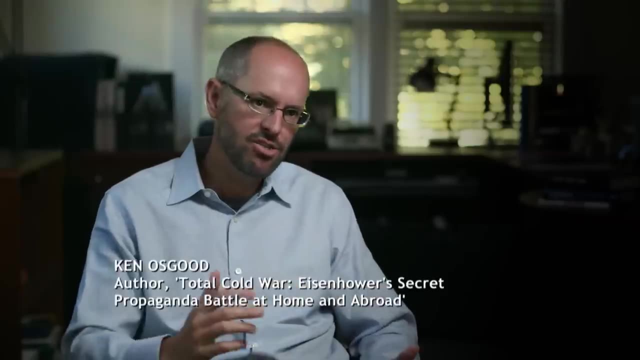 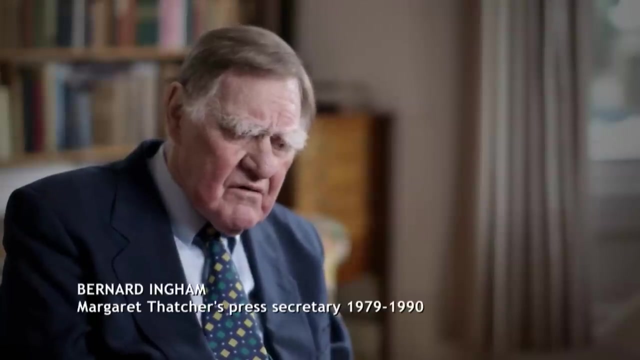 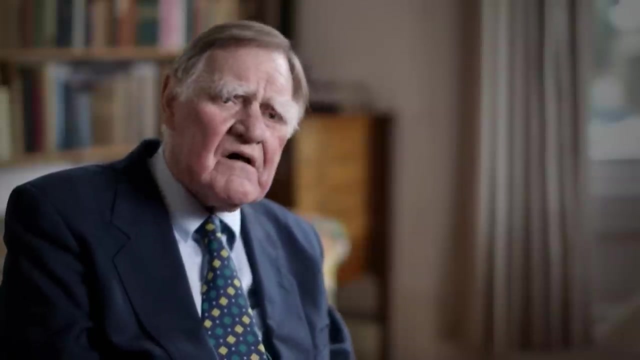 why don't you love us anymore? advocates of nuclear power and opponents of nuclear power just didn't speak the same language. it wasn't that one of them had a monopoly of facts is that they interpreted the evidence differently. they saw the range of concerns differently. the 1980s were a period of difficulty, but there was at least an element of the nuclear 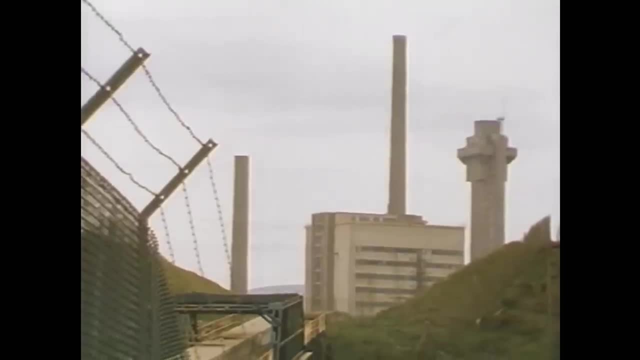 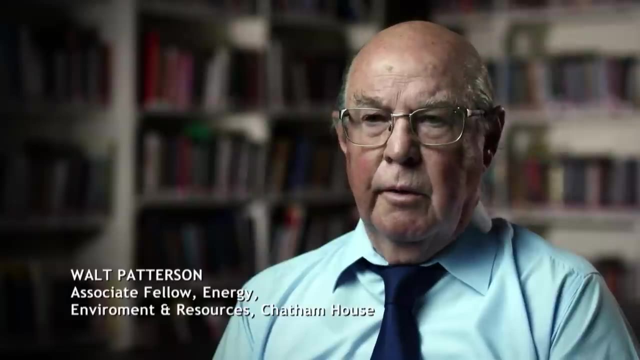 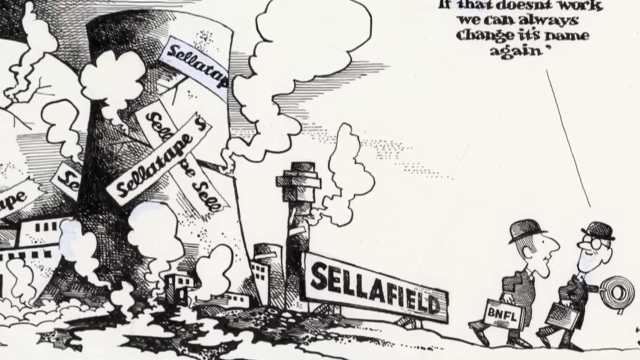 industry that was trying to deal with the public relations, the explanation, the reassurance. bnfl had decided that they would no longer use the name windscale for the facility. they would call it sellafield, which is the name of the little village where it had originally been built. 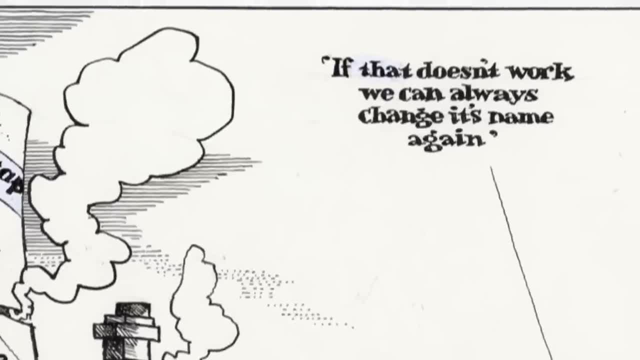 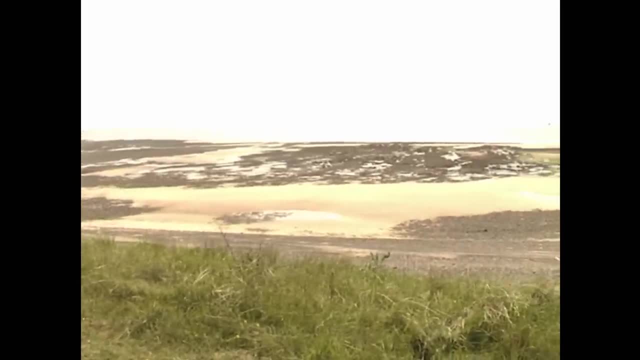 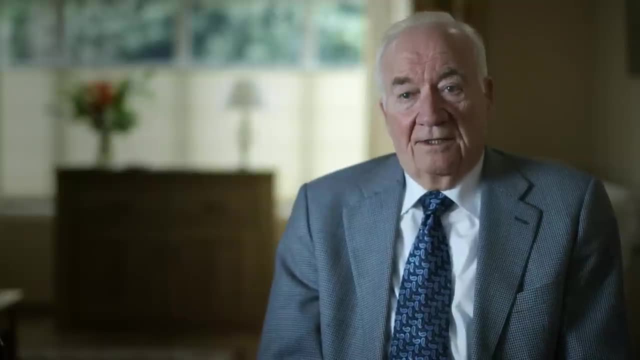 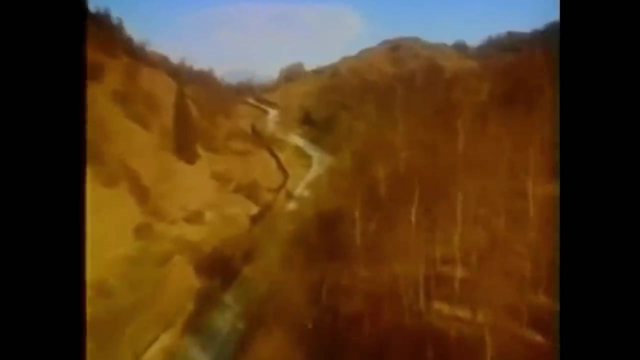 ironically, soon after the name change was announced, bnfl was accused of having radioactivity on the shoreline and leaks in at least two of their facilities. i was tempted to go and tackle the safety issue and then i was told no, be positive about the good things which nuclear will bring. 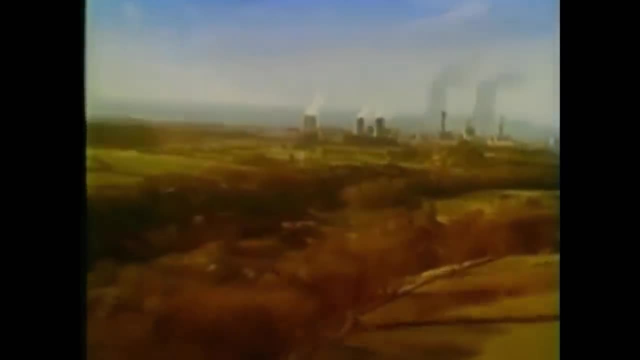 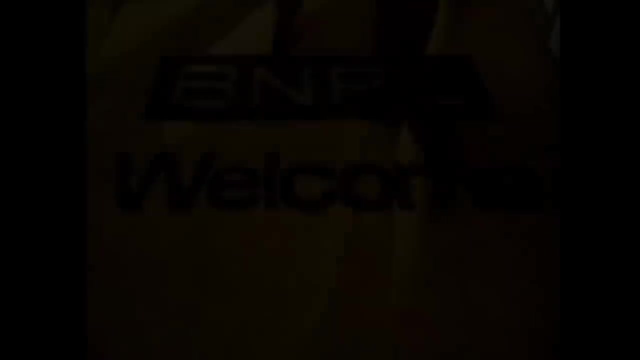 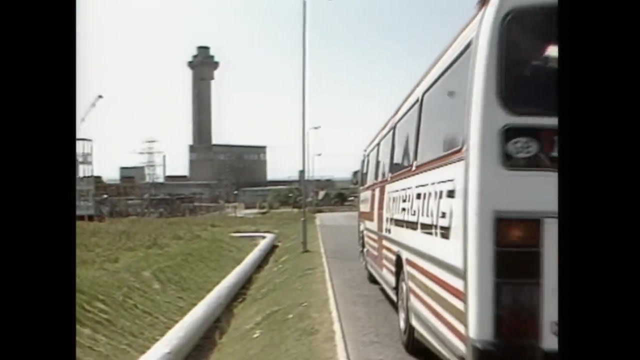 and that was the start of the idea of a visitor center, because the facts at the sellafield exhibition center are there for all to see. welcome to sellafield. ladies and gentlemen, my name is paul wilson and today i'll be showing you around the sellafield plant on a guided bus tour. 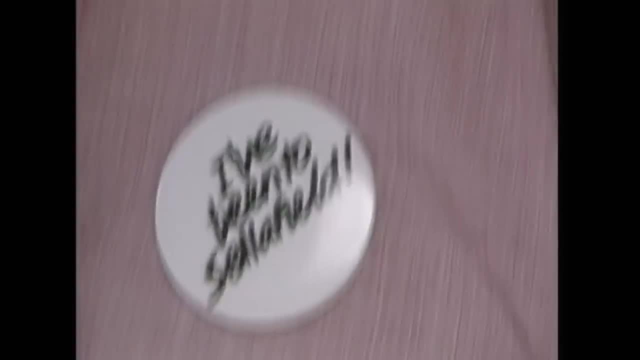 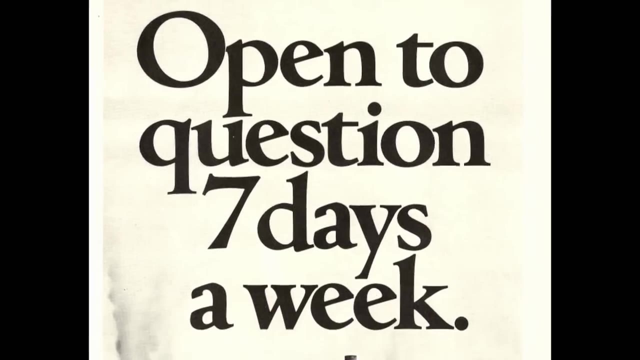 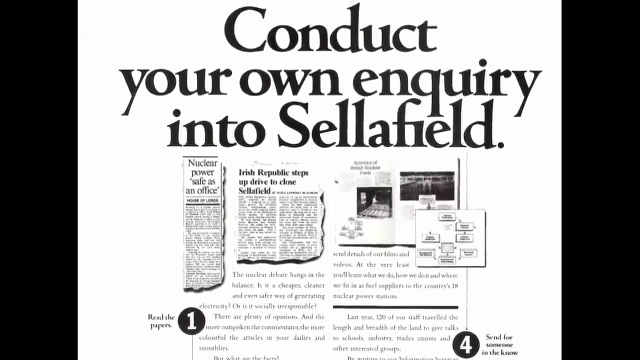 the tour will include a visit to culver hall power station to see the generation of electricity there, on the world's first commercial-sized nuclear power station. subliminal messages got through which we could then build on, mustn't it? because they've invited us to go up, go around, and they are trying. 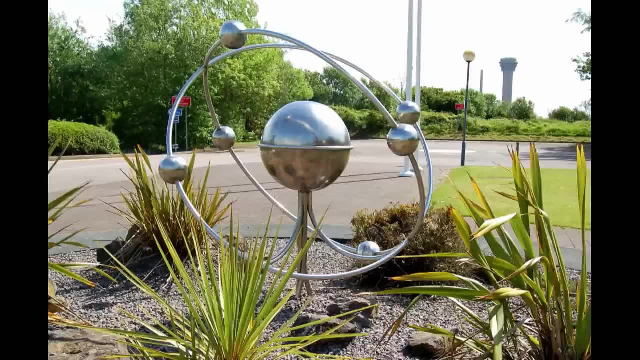 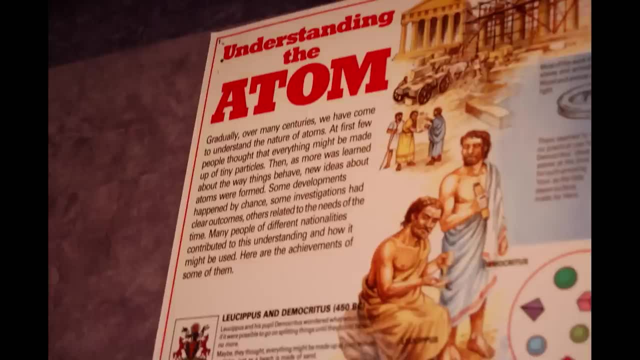 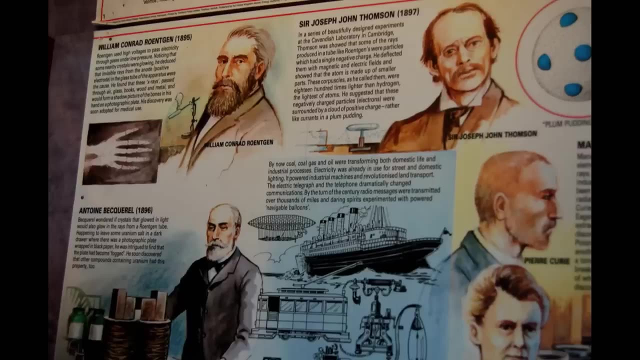 to be open and honest because they're asking us to go there. nuclear had previously been really in in secrecy. the industry had acquired a reputation for just not telling anybody anything, and a result: uh, no one really trusted them. so they went for a kind of- uh kind of- glasnost openness policy and they, they tried to break down the, the suspicion. uh. 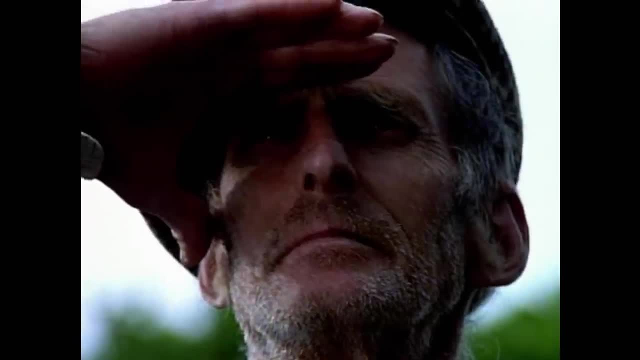 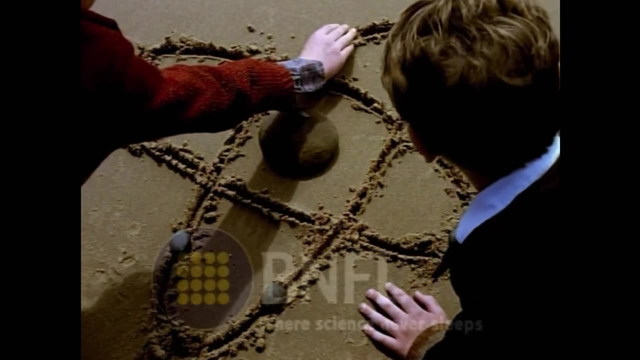 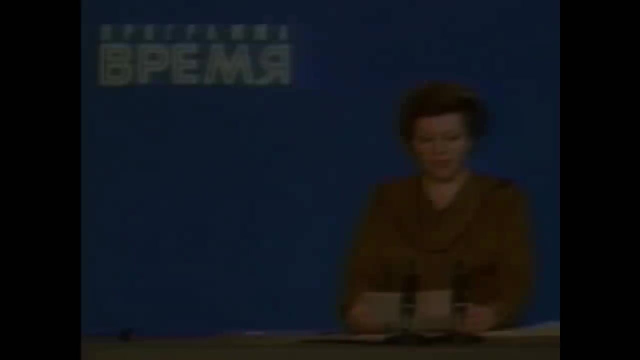 accompanied nuclear over the previous decades. to learn more about what we do and how we do it, come to our new visitor center at centerfield, the nfl. as science never sleeps. and then, just as the charm offensive finally seemed to be working- unless viewers of moscow television were watching, the 9 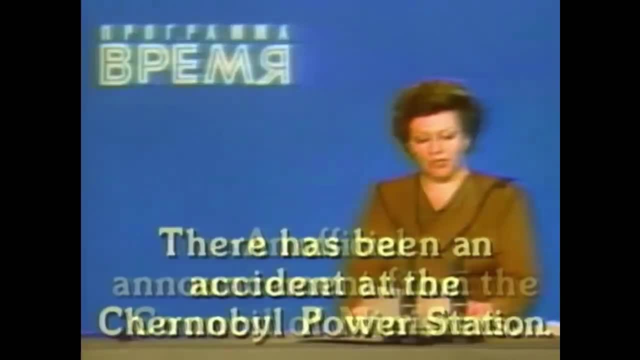 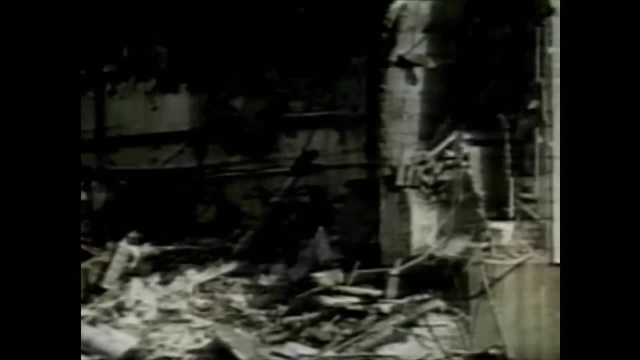 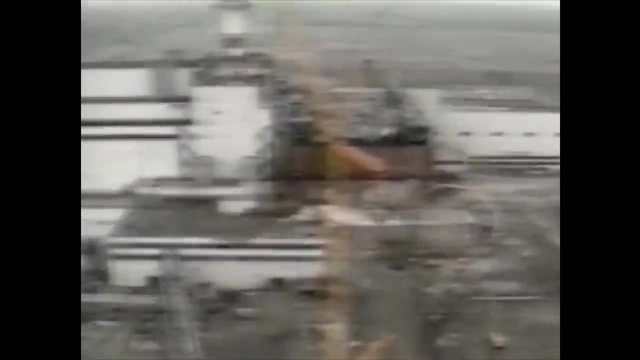 pm news closely on monday, april 28, they would have missed the brief and buried report of the biggest nuclear accident in history, an accident that had occurred at least two days earlier at chernobyl in the ukraine. chernobyl definitively ended the industry's 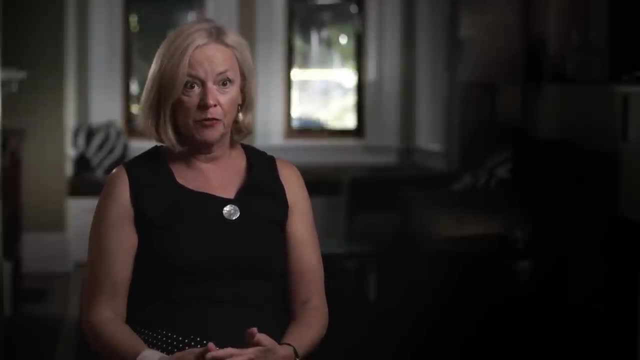 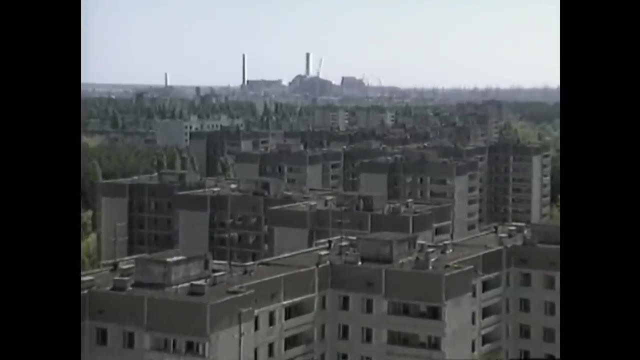 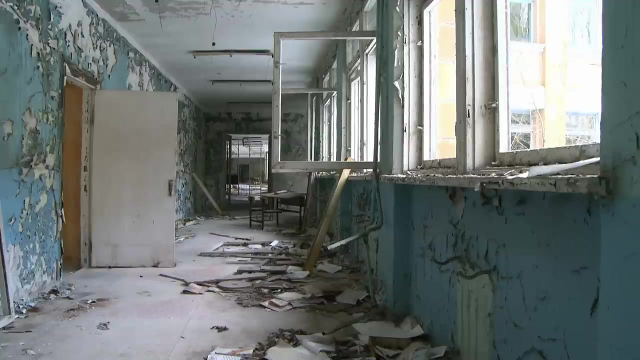 line that there could never be an explosion, that a reactor could never blow up like a bomb. effectively, that's what happened: it blew up. we're talking here about uninhabitability. after chernobyl, there were 12 500 square kilometers all around it in ukraine and belarus- uninhabitable. 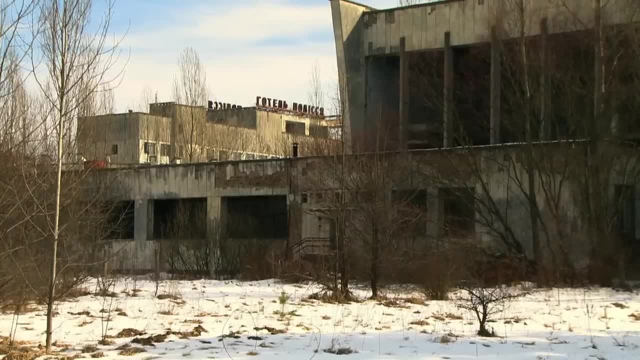 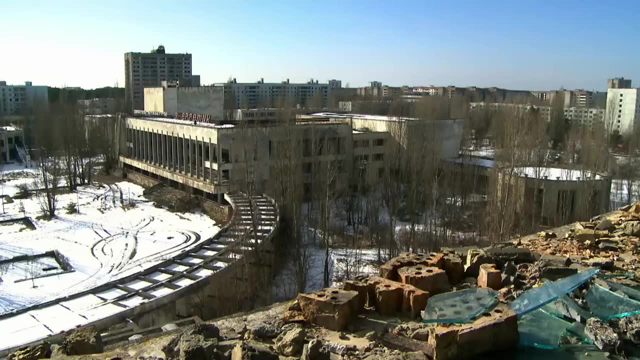 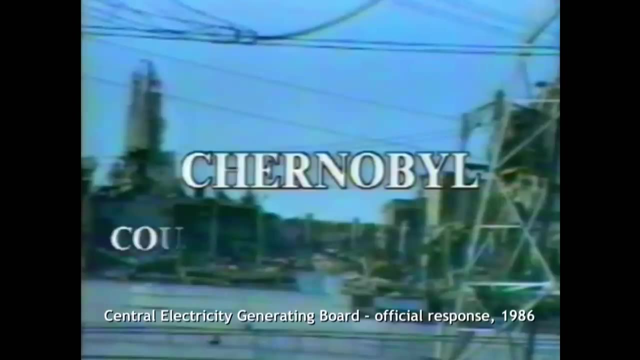 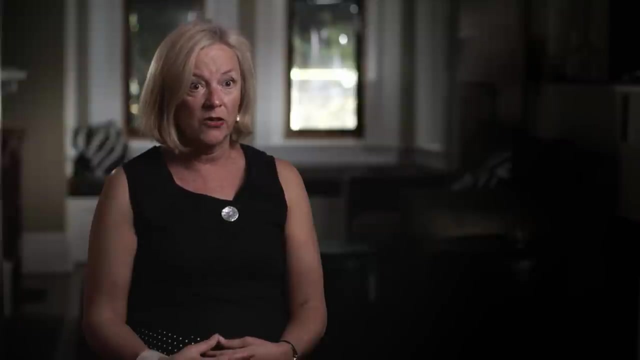 nothing but you know, animals and birds, abandoned villages, abandoned towns, doors swinging open in the wind. it was a dramatic event and, of course, did create widespread doubts about nuclear power. there was a very concerted effort by all the western governments to distance themselves as fast as they could. 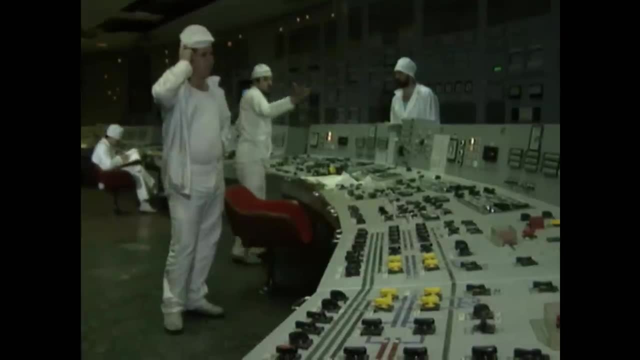 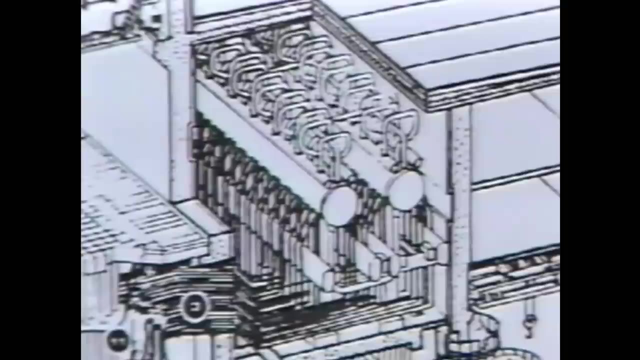 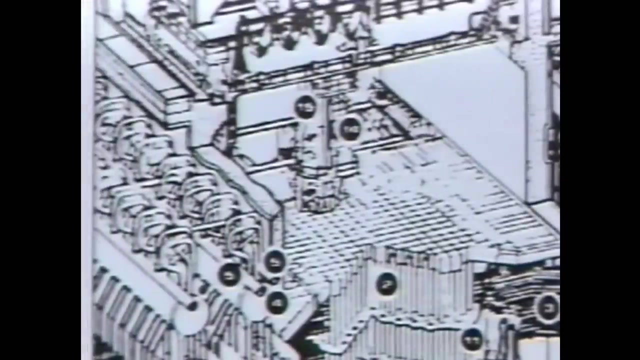 and blame it all on russian technology. it can be stated categorically that an accident similar to that one could not happen in a british nuclear power station. the reactor of the genoble design simply wouldn't have been allowed to operate in britain. it was a very serious incident and i did question whether i wanted to stay in the industry. i came to conclusion that i did well. Chernobyl hasn't changed my opinion at all. I was quite happy before Chernobyl, as I am now. Our safety standards are very high and we've got many backup systems. 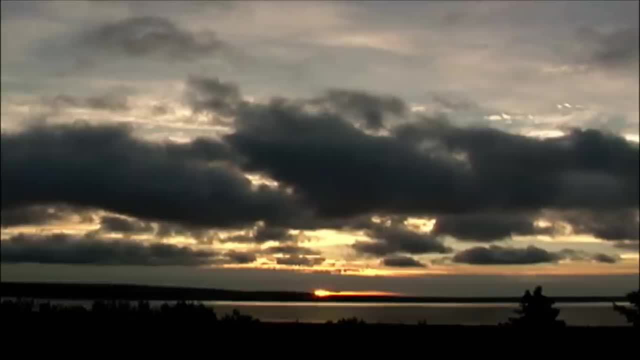 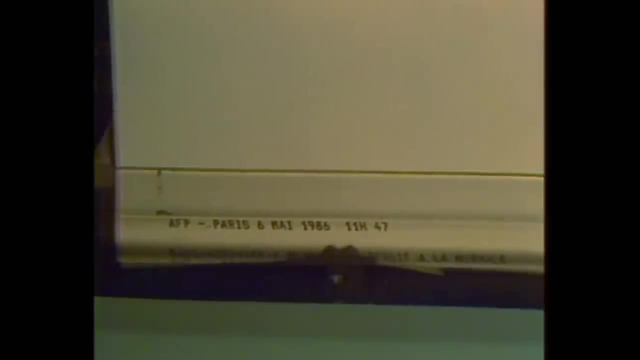 and I feel there's no problem at all. In the days following the disaster, a plume of radioactive fallout drifted west over Europe much to the alarm of those in its path. After Chernobyl in Germany and Italy, it was almost hysteria collective. 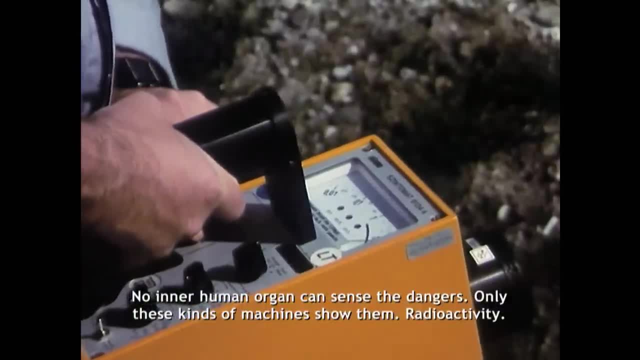 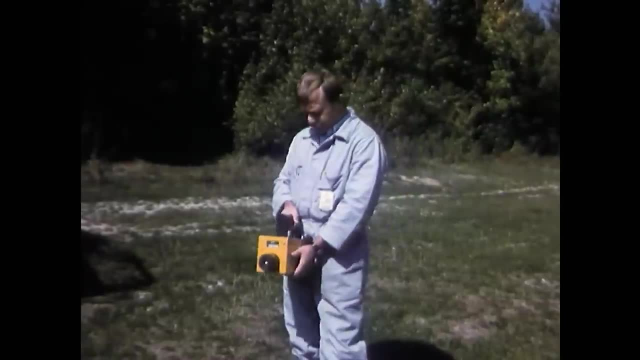 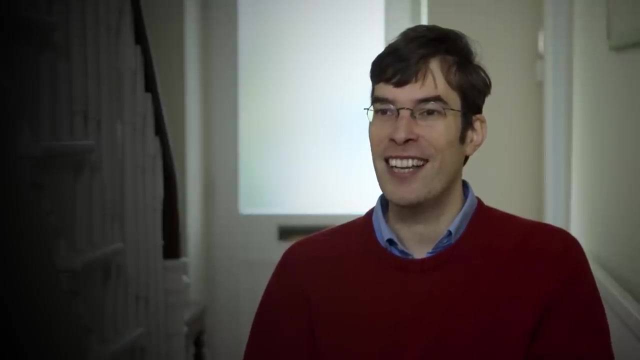 I was there on the school playground with my geography teacher at the time, who had got himself a Geiger counter out of the pharmacy to check whether there was any high radioactivity level. Of course it was useless because we didn't know what the normal level was. 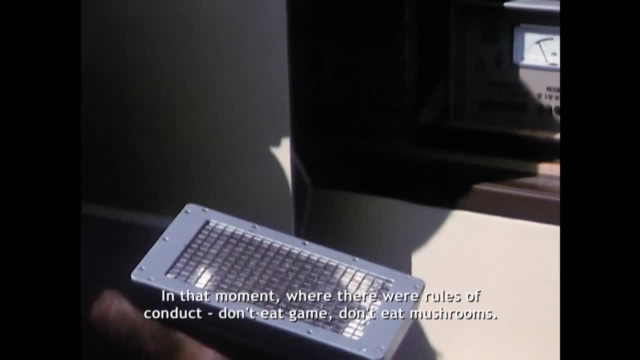 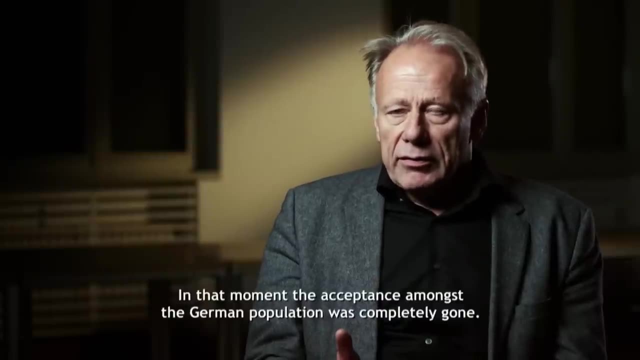 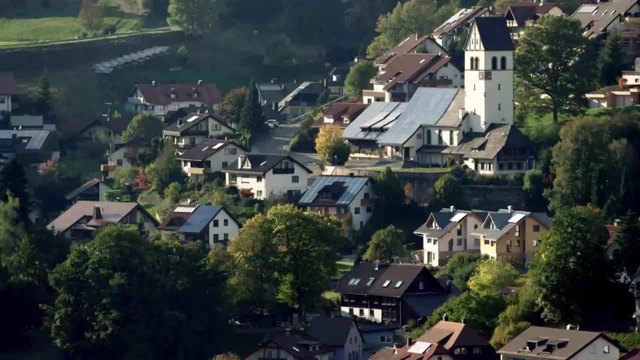 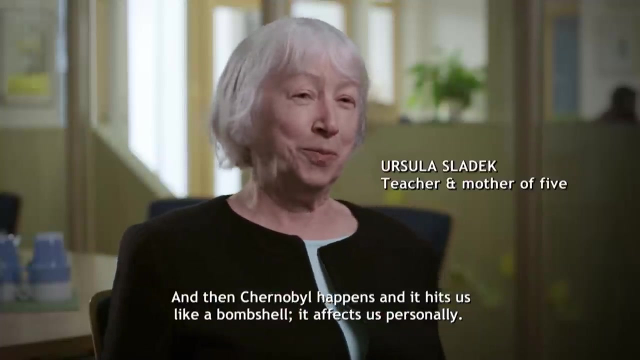 In the moment when there were behavioral measures, there was no wild animals, there were no mushrooms. At that moment the acceptance in the German population was completely gone. Life is quite normal and just goes on like that. And then Chernobyl happens, and that hits us like a bomb. very personally. 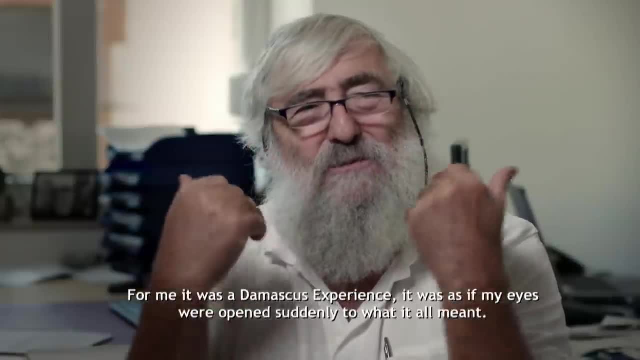 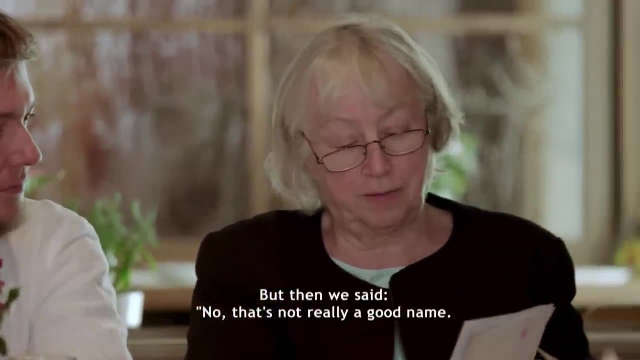 For me, it was an experience in Damascus. For me, it was like a drop of water falling from my eyes. what does that even mean? At first we called ourselves Parents Against Atomic Power, but then we said, no, that's actually not a good name. 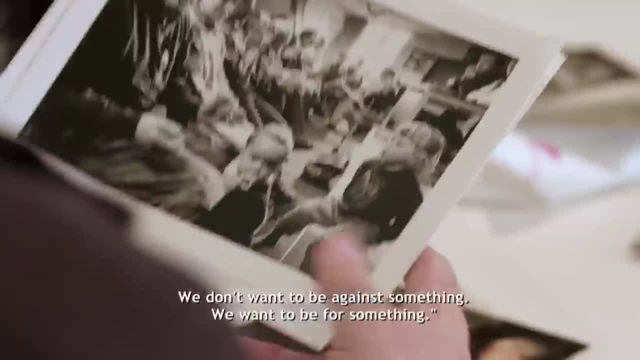 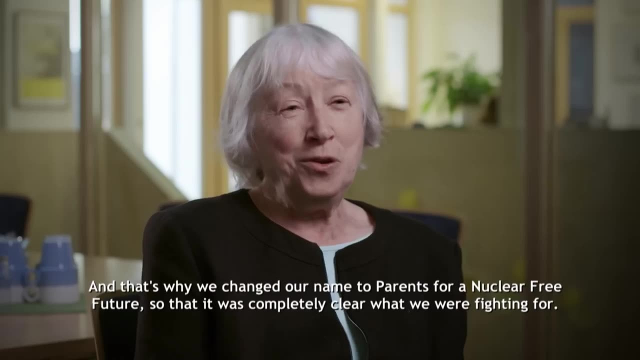 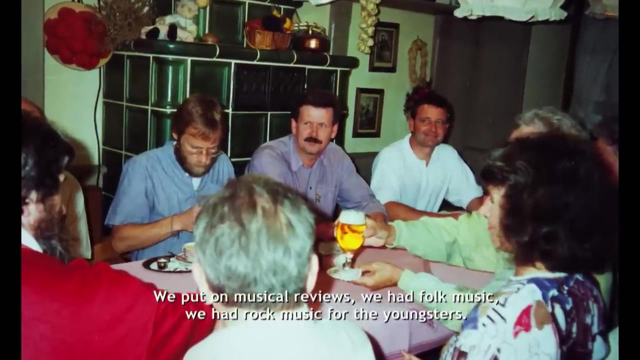 We don't want to be against something, we want to be for something, And that's why we changed our name to Parents for a Nuclear-Free Future, so that it's clear what we're for. We did a lot of musical stories, we did folk music, we did rock music for the youth. 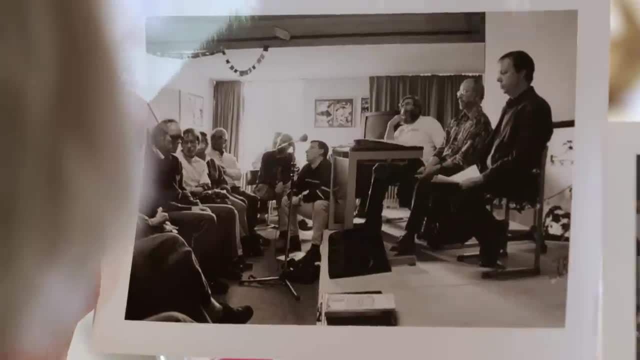 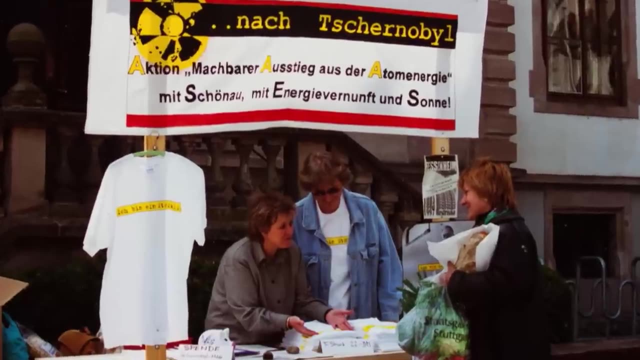 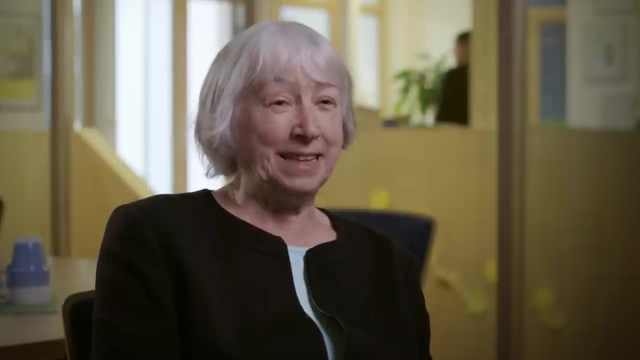 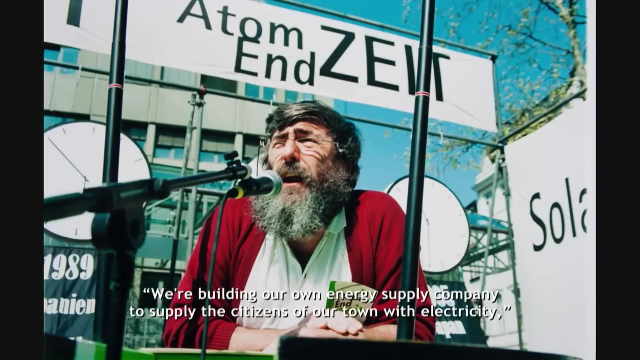 She's Odin. The German-American families were so committed to ridding their village of nuclear power that they made an audacious bid to take control of the local energy grid. Because you can imagine when a citizen initiative says: we're building our own energy supply company to supply the citizens of our city with electricity. 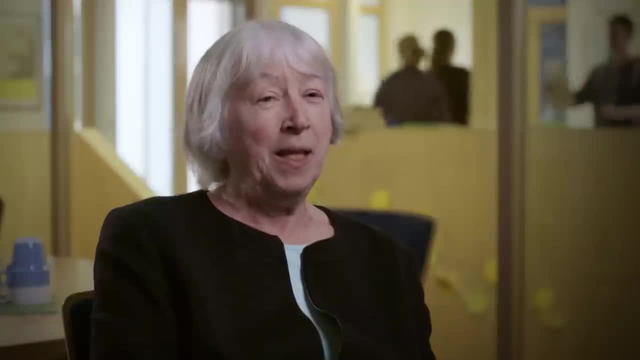 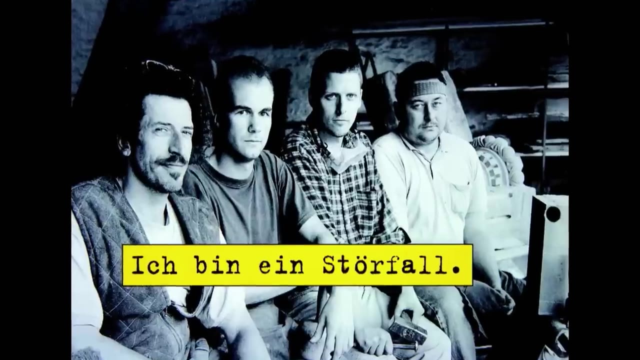 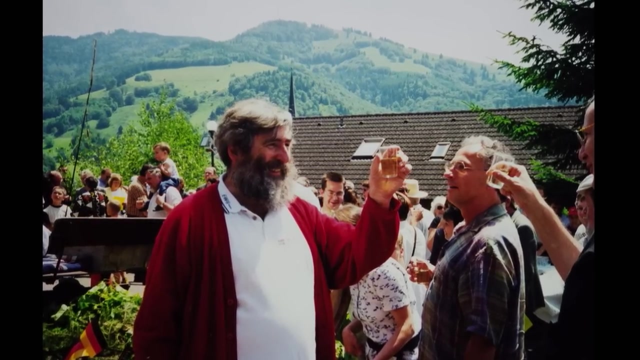 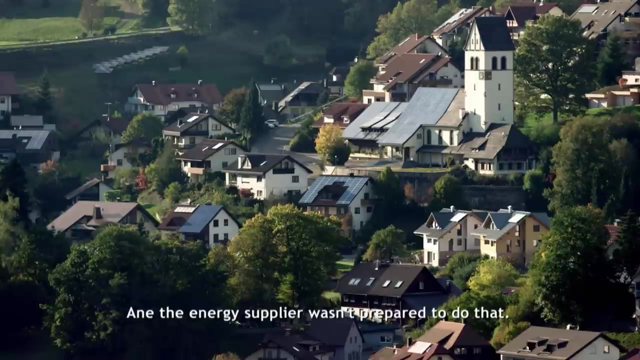 then everyone says, yes, how is that supposed to work? And of course, the energy supply company was the one that did it. But against all the odds, these energy rebels did succeed creating a new citizen-owned energy cooperative Back in Britain. they had other things to worry about. 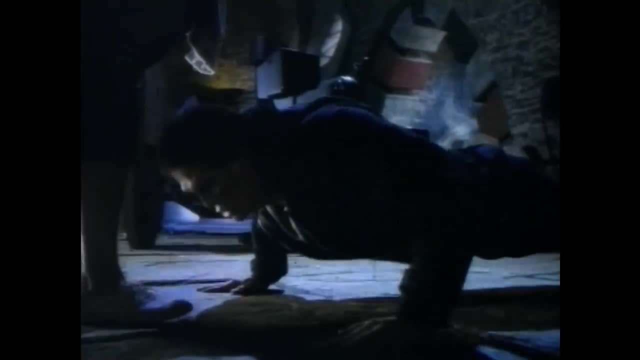 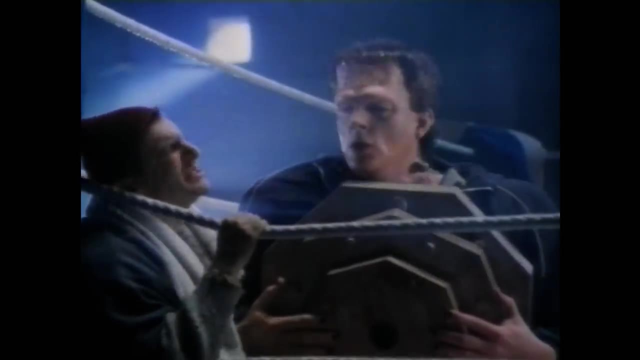 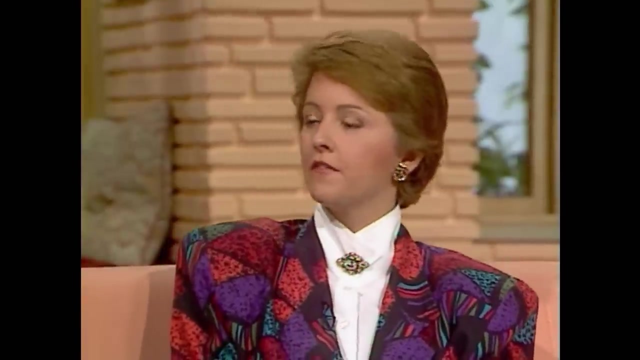 All over the country, ordinary electricity users will be preparing For the 12 regional electricity companies share offers, As nuclear power threatened to sink. one of Margaret Thatcher's flagship policies: The postponement by six months of the privatisation of the electricity industry. 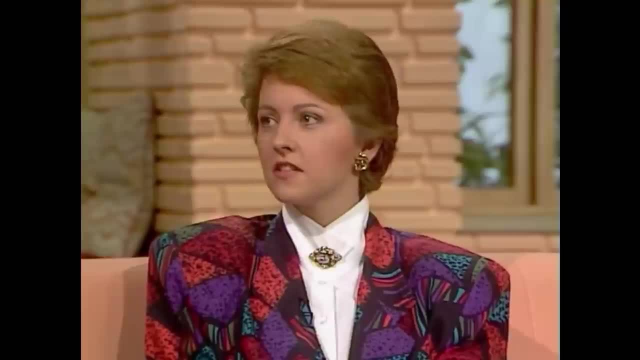 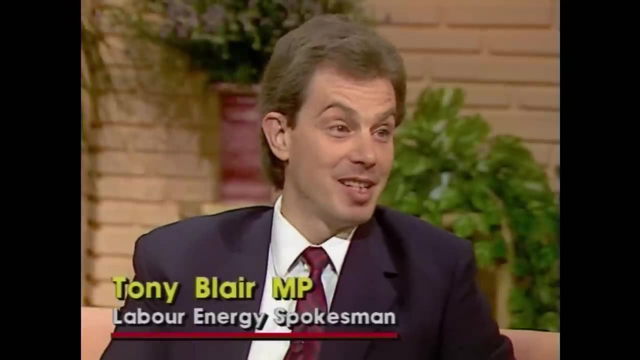 is only six months, I mean, it's still going to happen. Is it really that significant? I think it's significant because what it indicates is that the plans are a complete mess And most people already realise that their bills have gone up in order to pave the way for privatisation. 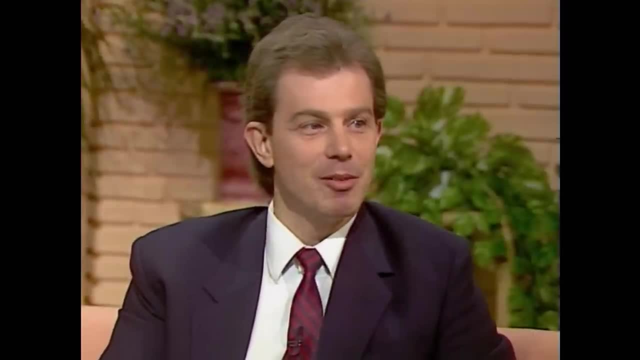 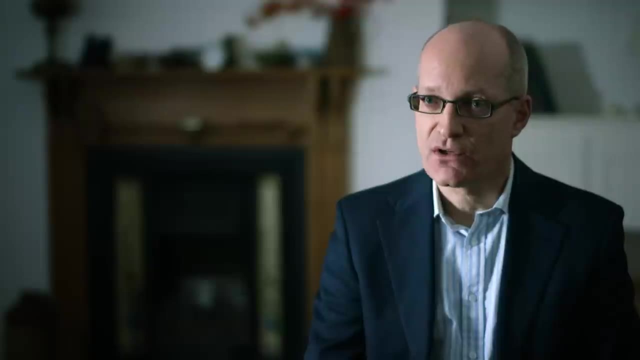 They've got huge. They've got huge problems because they want to sell the nuclear industry, which is going to be very difficult to sell, The cost of ultimately decommissioning the stations, where you return the site to essentially a completely usable, clean status. 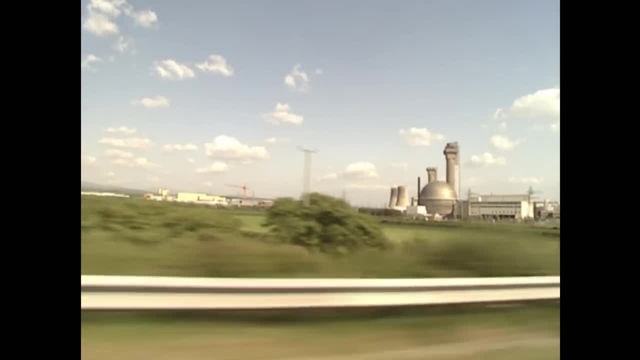 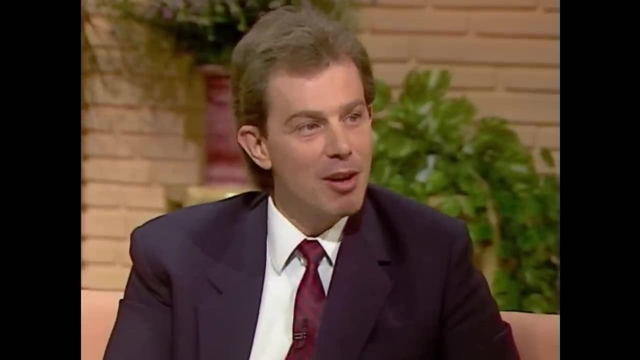 had been underestimated. The costs of future dealing with the spent fuel had been underestimated. I think it's very unwise to embark on a new nuclear programme when we don't even know how to deal with what's left over the legacy of the old nuclear industry. 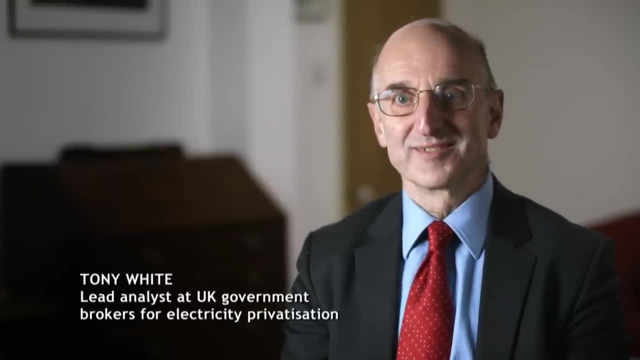 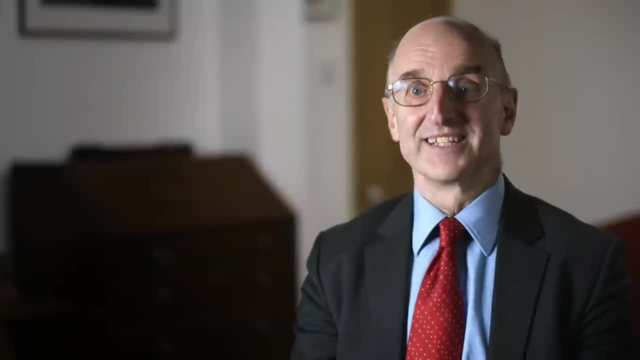 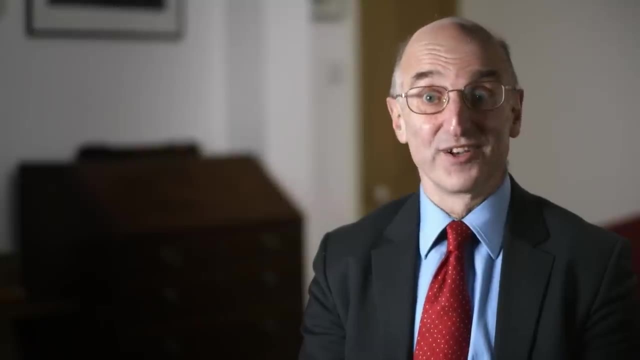 So we went away and we're trying this and we're trying that, But in the end we just said: look, we just really can't do it. And so the government in the end said, OK, you can't do it, therefore we will pull it. 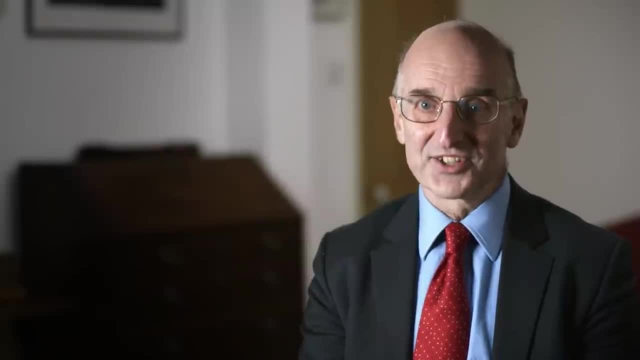 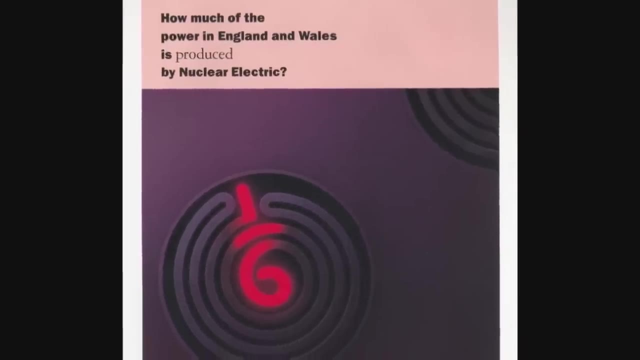 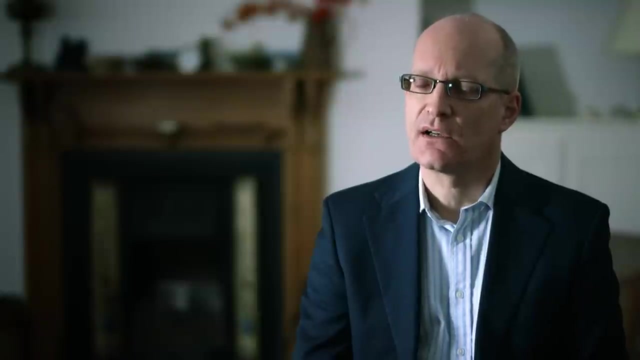 And it was quite a momentous occasion. A few years later the government did finally manage to sell off its nuclear power stations. But it wasn't long before the new private nuclear company also ran into trouble. The company went into steady financial decline from about the year 2000.. And by 2002, it was in effect bankrupt. It had to be rescued by the government, with £340 million initially, And eventually it went up to over £600 million to keep the company alive. The message was a pretty clear one for all of us. 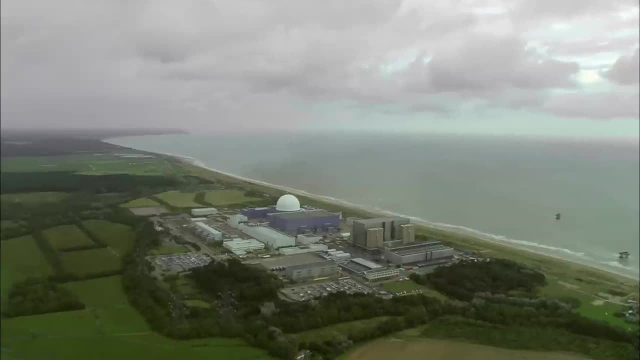 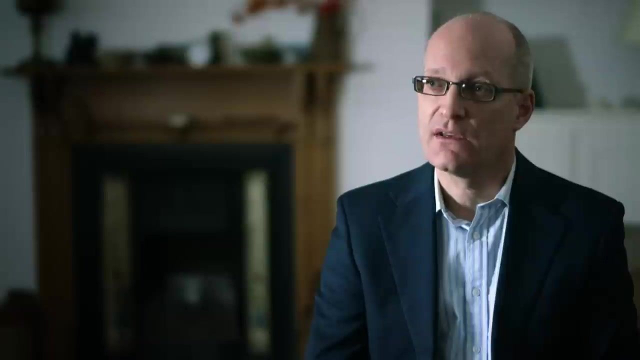 If we're all potential future nuclear investors, this is a very risky business. Nuclear suddenly looked like just a dead end area to work in, And these often very, very well qualified, very smart people felt that they'd made a terrible career choice and that their whole life had, in a sense, been wasted. I remember the 1990s getting to a point where I thought: well, maybe the nuclear dream has died. There really was a global decline In the past where they've been planning hundreds- 300 or so new stations. in the 1990s it was down to below 20.. 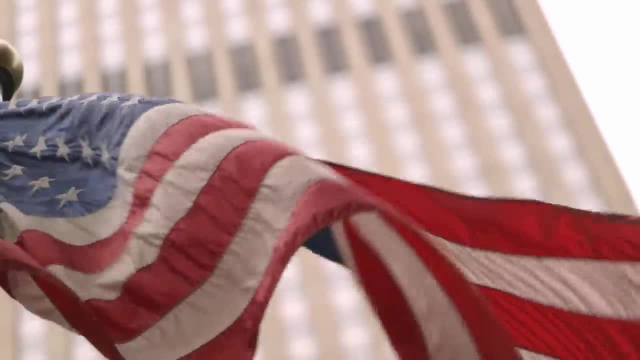 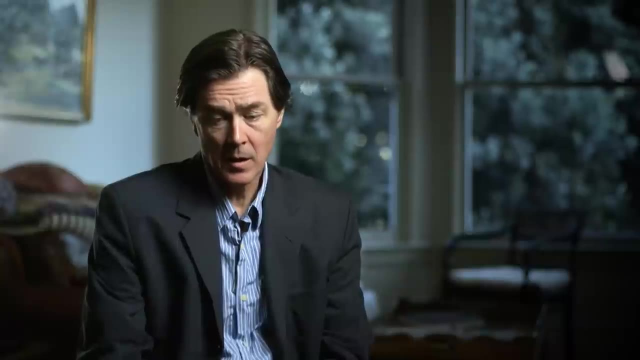 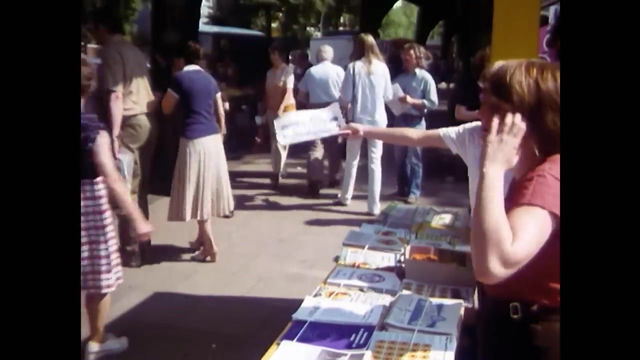 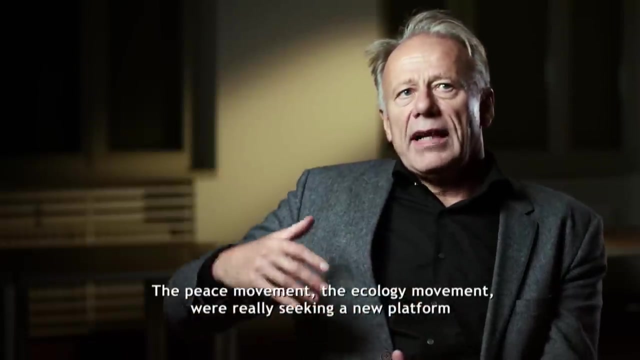 In the United States. nuclear was not growing, They were not selling new reactors, The whole industry stayed essentially in a near-death condition. The atom had never looked so vulnerable, and nowhere more so than in Germany. You feel Germany watched the global climate, the economic movement, the climate movement. 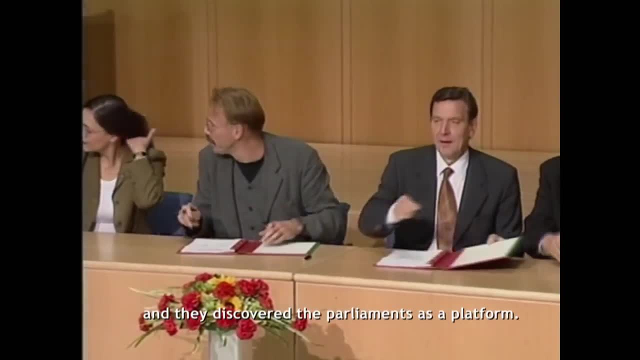 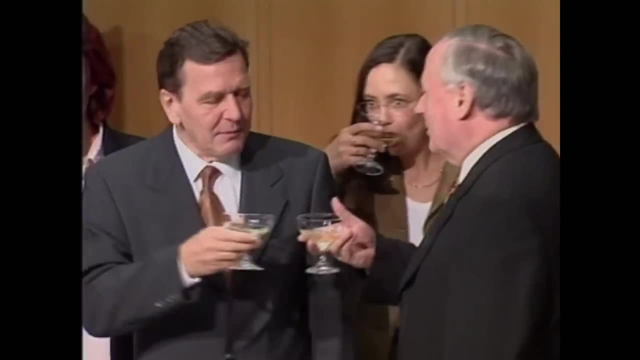 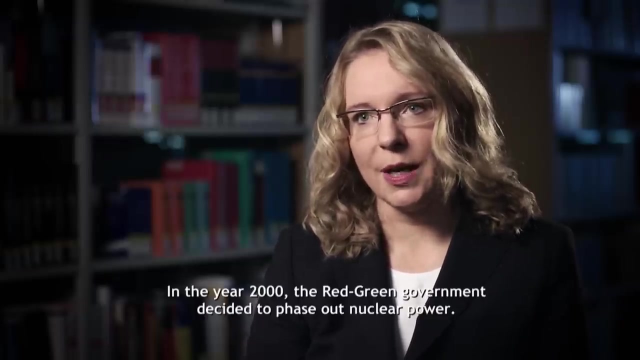 actually looking that they wanted a new platform. They discovered the secretaries as a platform. When the Green Party formed a government with the centre-left Social Democrats in 1998, time was up for nuclear power. In 2000,, the red-green government decided to emancipate from nuclear power. 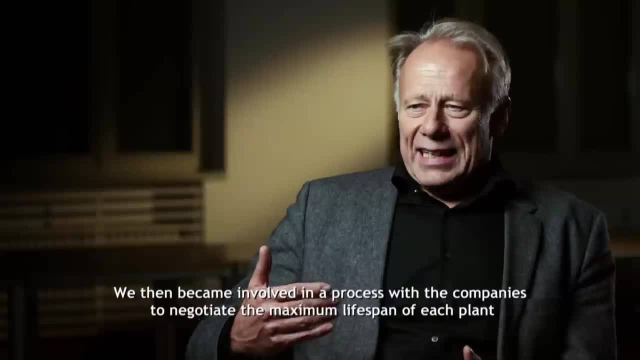 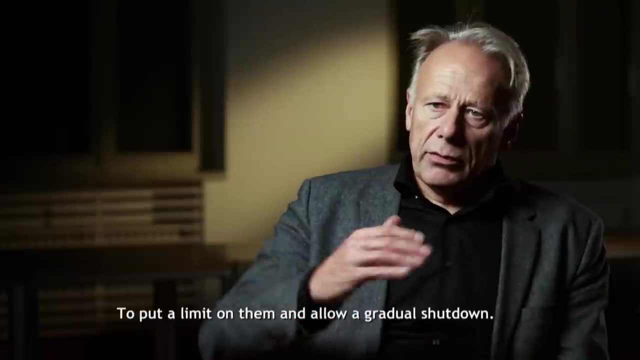 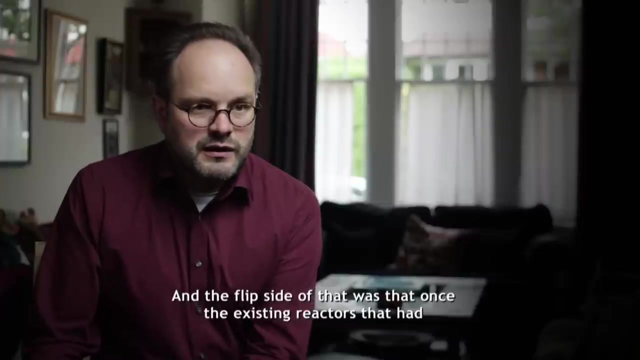 Then we agreed on a process to negotiate with companies on the issue that they limit the running times, which were unlimited until then, so that it can be switched off step by step. What was said at the end of the day, if the existing reaction of the reactors which went into operation in the 70s and 80s 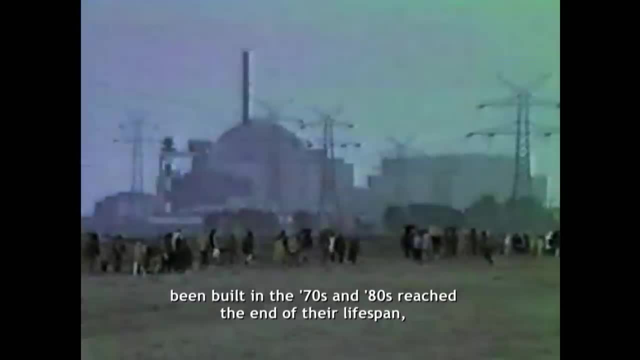 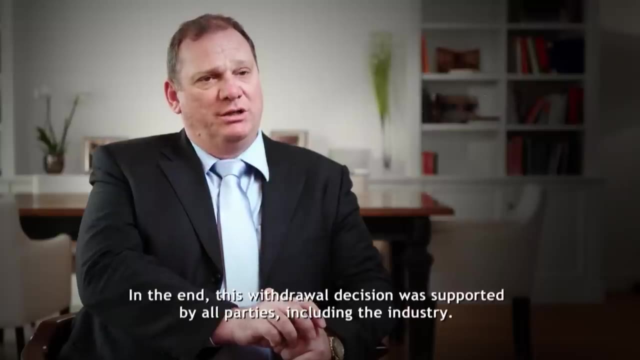 if they come at the end of their running time, then, so to speak, the nuclear exit in Germany would come from itself, At least at the end. this exit decision was carried out by all parties, also by the industrial partners, And this has also been widely accepted. 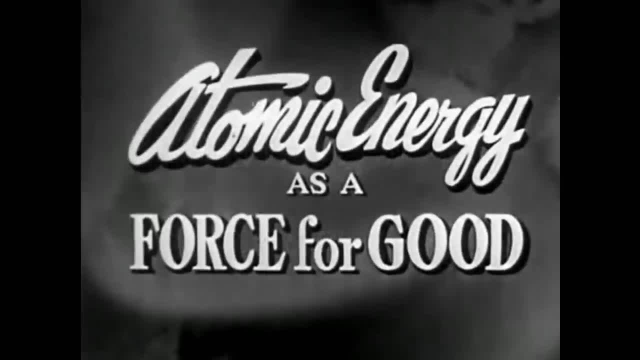 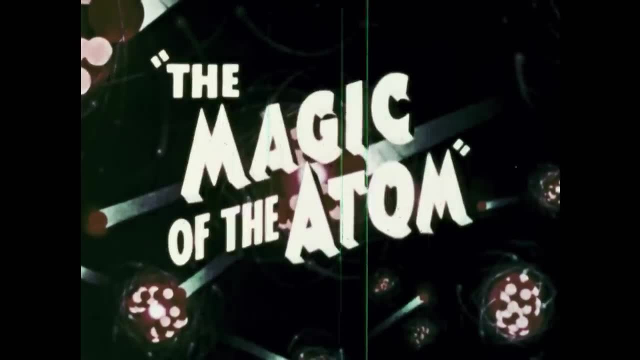 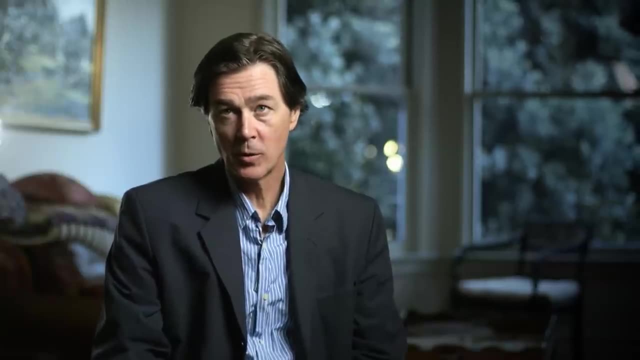 also in the media. the population has supported this. The atom was yesterday's news. It desperately needed to recapture the excitement of those early years. But how? The very first time I heard the term global warming was from a nuclear power industry executive in 1981. 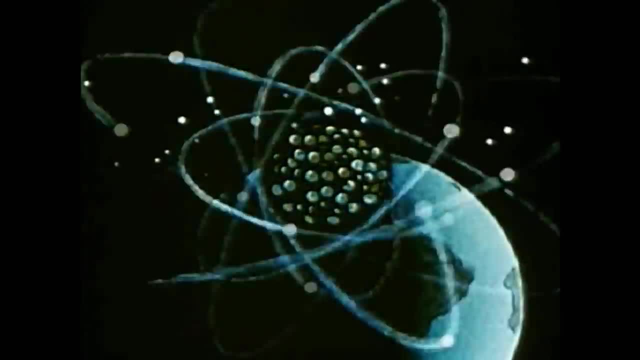 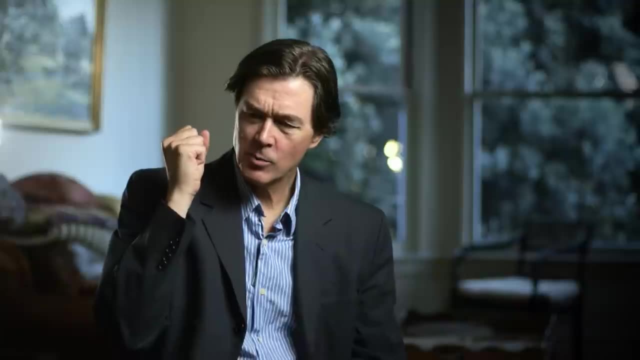 I mean, I said: what is that? And he explained what global warming was. and he says that's why we can't rely on coal. He says, just once I'd like to pick up the phone and say: Atomic Industrial Forum, coal kills. 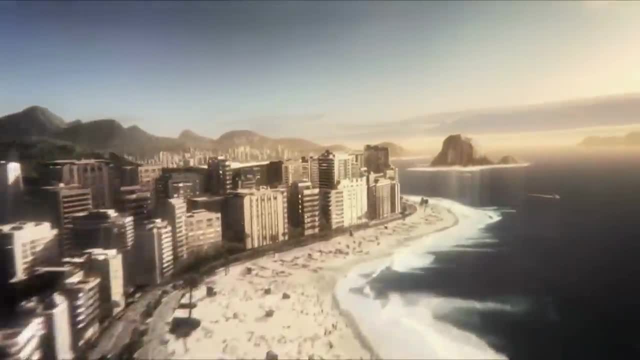 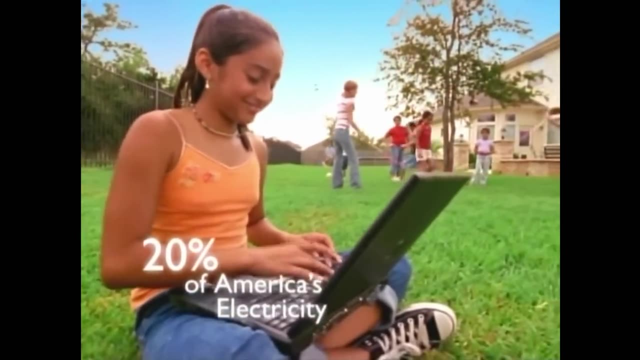 Energy is a story that is still being written. Let's continue writing it with less CO2.. By the 2000s, people had begun to realize that global warming was a severe problem And people, even leading environmentalists, began to say: 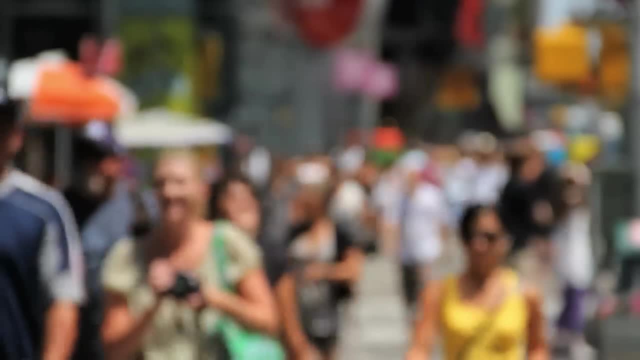 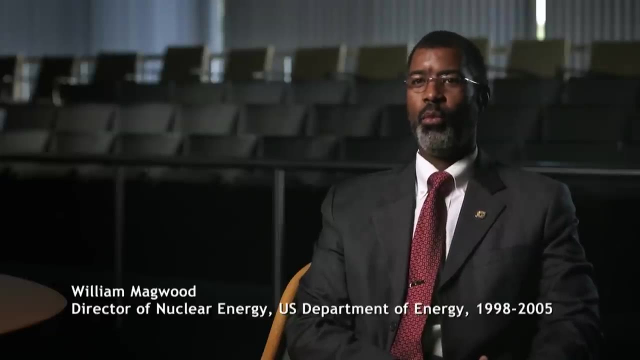 well, maybe we'd better rethink nuclear power. The threat of climate change prompted us to ask the question: if we wanted to build nuclear plants in the United States by the year 2010,, what would it take? So we started to ask that question to the Department of Energy. 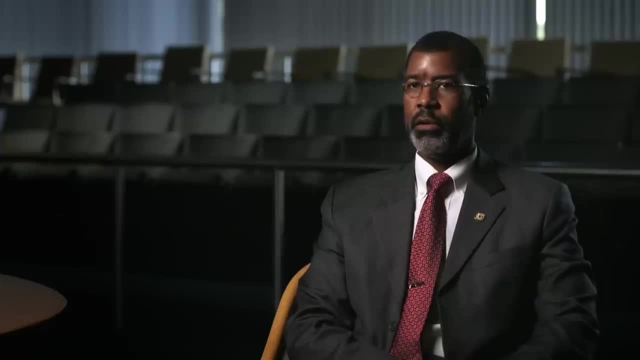 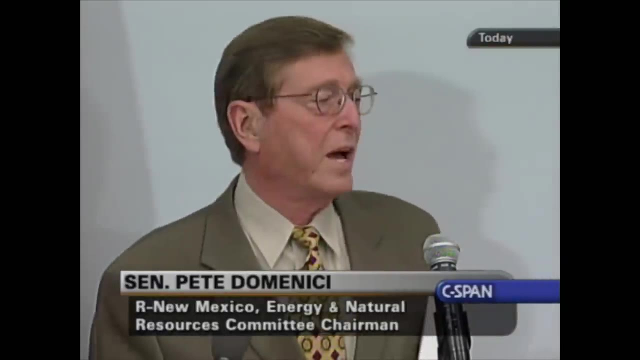 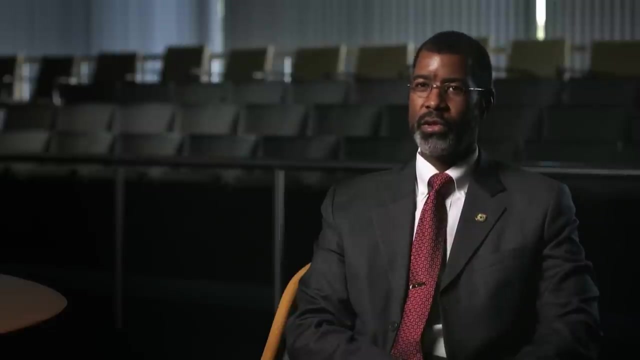 But also there were policymakers. Senator Pete Domenici was a leading voice in the Congress on this. I think we all know that the world must have nuclear power as soon as possible. We funded and co-funded with industry various activities to try to break through some of the barriers. that made nuclear a non-viable option for the industry And that, I think, was the beginning of the turnaround. It is time for this country to start building nuclear power plants again. We are announcing roughly $8 billion in loan guarantees to break ground on the first new nuclear plant in our country in three decades. 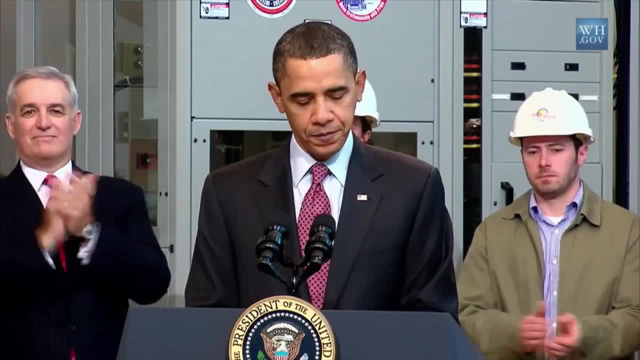 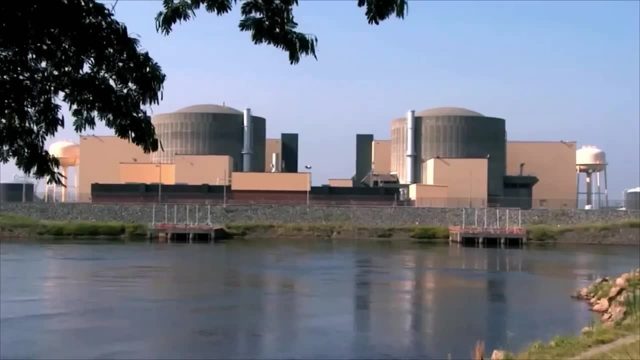 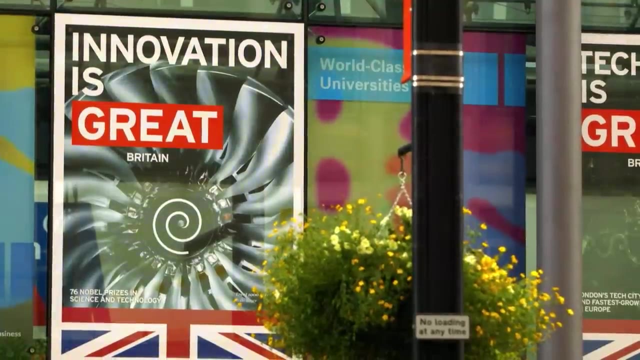 The first new nuclear power plant in nearly three decades. The US nuclear industry brimmed over with renewed confidence as 13 companies applied to build 25 new reactors, And the mood was changing in the UK too. By 2025, if current policy is unchanged, 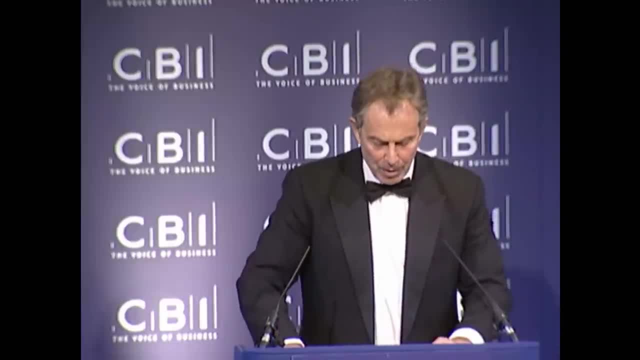 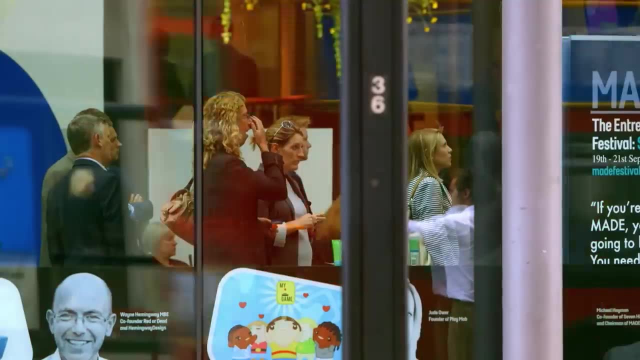 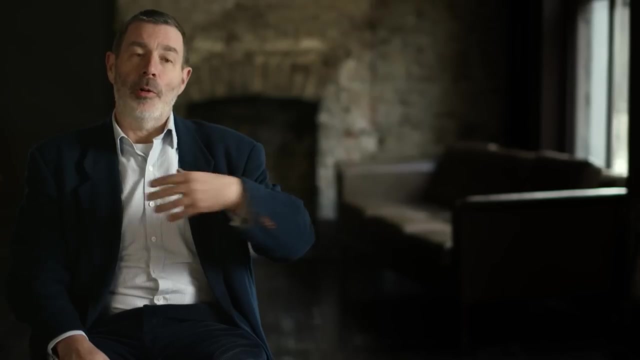 there will be a dramatic gap on our targets to reduce CO2 emissions. These facts put the replacement of nuclear power stations back on the agenda with a vengeance. I suppose we shouldn't be surprised that politicians say one thing in opposition and another thing in government. 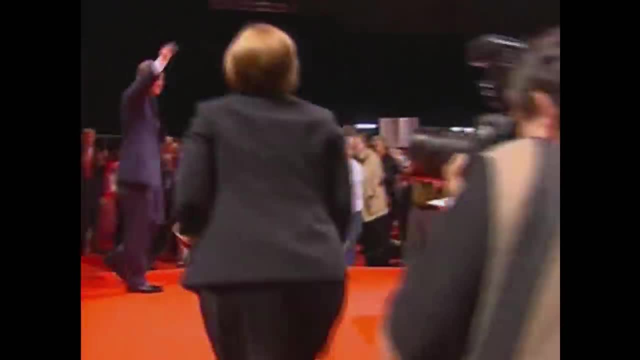 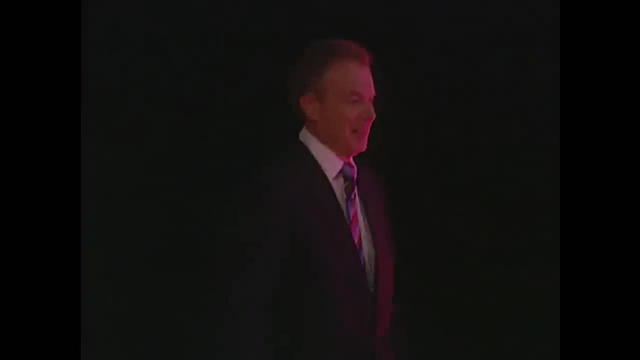 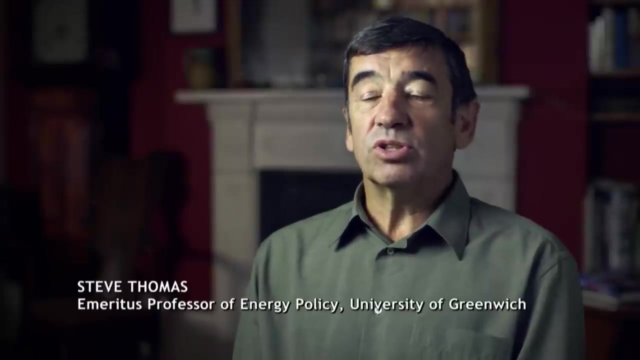 but that's what happens, and that's certainly what happened to Blair. It was often reported that Tony Blair wanted to leave a strong legacy, and that part of his legacy was perhaps launching a nuclear power program that would solve the problem of global warming. 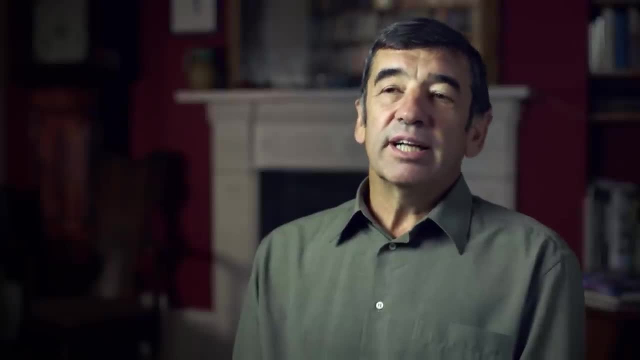 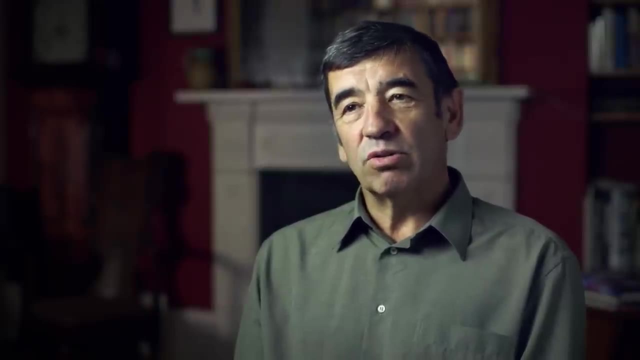 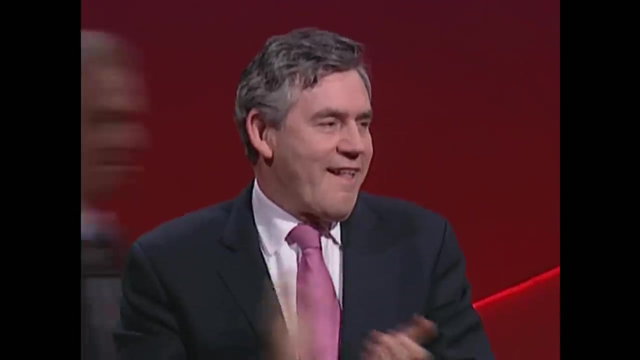 Insulating a few lofts, bringing in a few small wind turbines on land, doesn't have that same impressive sound to it as launching a huge nuclear power program. Blair's successors were equally enthusiastic. In 2008,, Gordon Brown called for eight new nuclear plants. 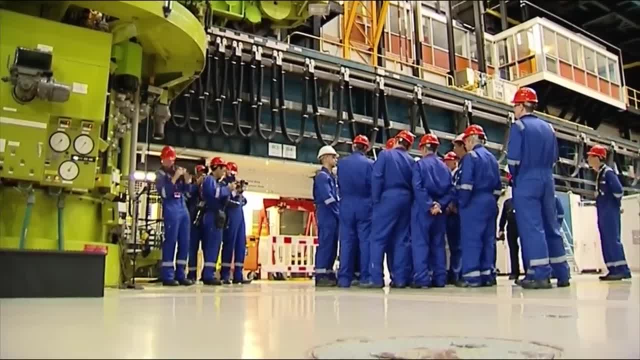 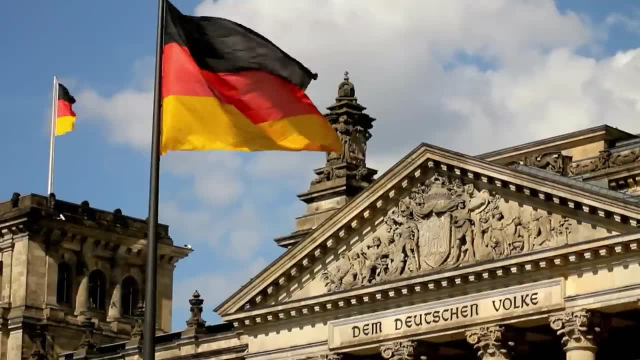 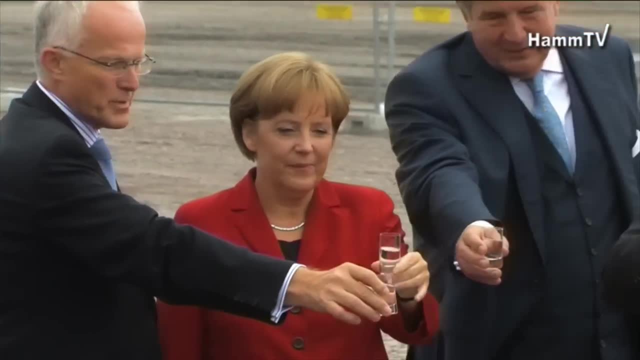 to be built across the UK And in 2010,. David Cameron's new coalition government greenlit these plans. Even the Germans looked like they might be willing to give the atom another chance. The nuclear industry knew that Merkel was rethinking her previous position. 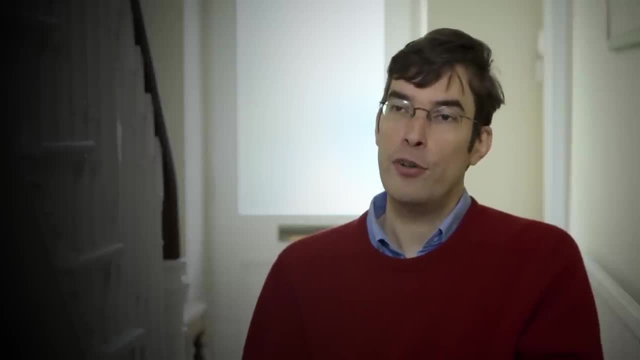 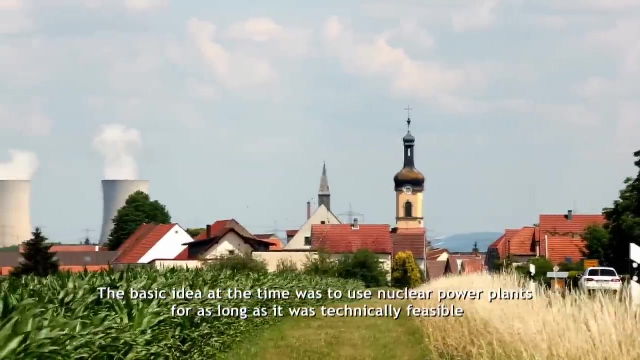 and then, when the CDU and the Liberal Party, the FDP, formed a government, they actually agreed to go back on their decision and not to phase out nuclear energy. The nuclear power plants were able to use the power as long as it was technically feasible. 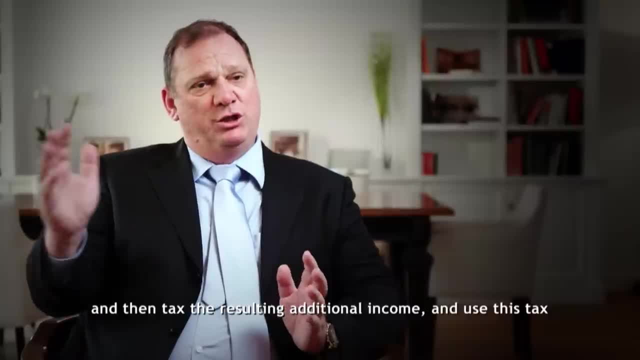 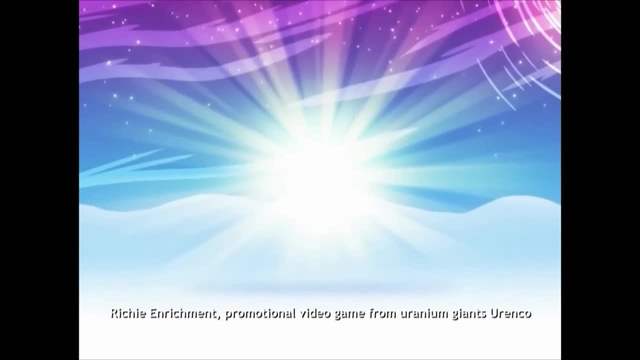 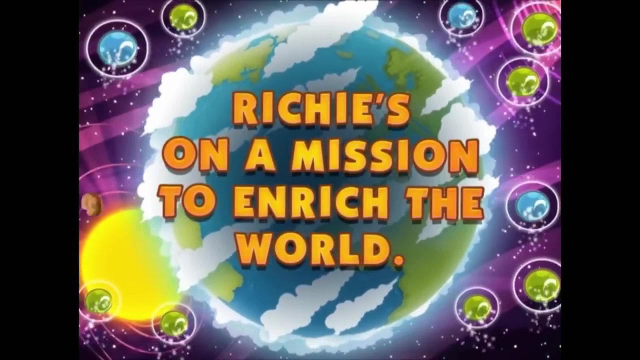 and to control the additional yields from it, and to use this power to finance energy changes in the energy-political landscape in Germany And the French were now hoping to repeat their nuclear success on the international stage. When Sarkozy came to power, many of the trips he made abroad 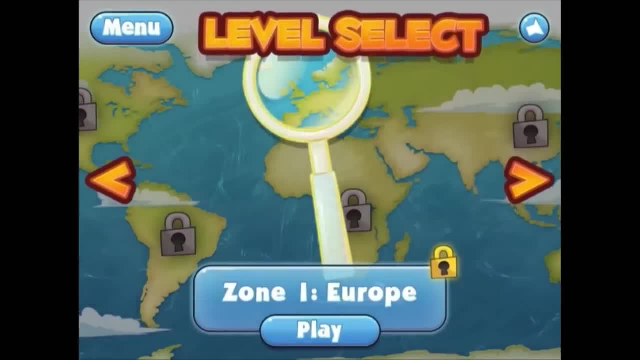 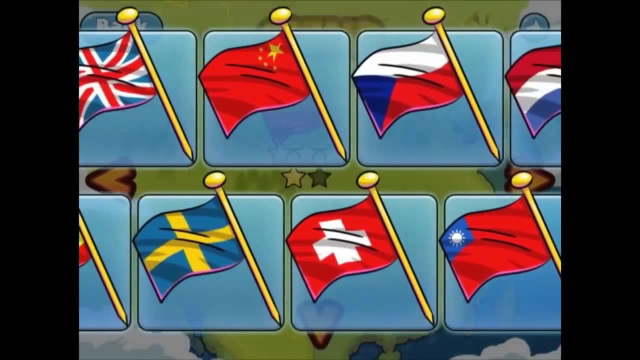 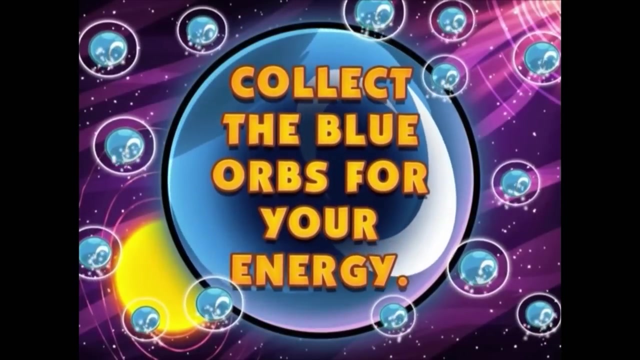 involved seeking nuclear power. He signed nuclear deals, He signed contracts with China. He signed nuclear cooperation agreements with several countries in North Africa and the Middle East. You need to keep in mind that you can't build endless numbers of reactors in France, no matter how enthusiastic you get about it. 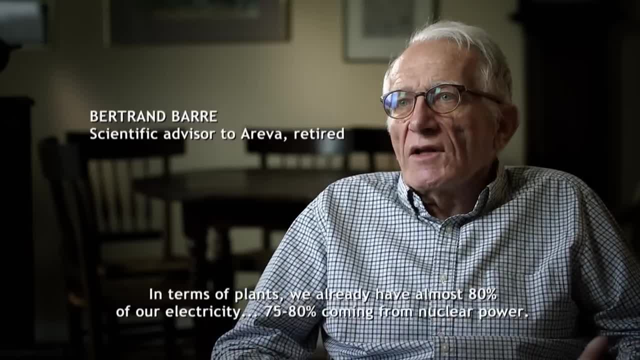 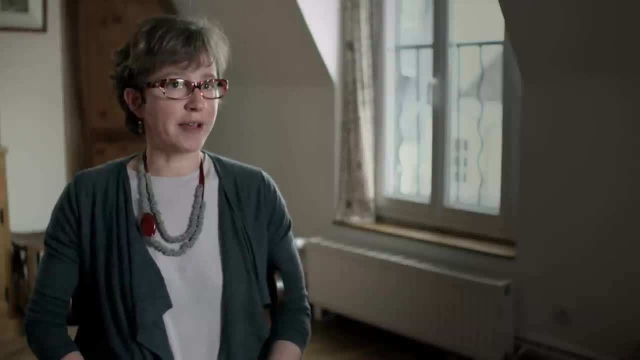 In terms of power plants, we already have 80% of our electricity, almost not 75, 80%- which comes from nuclear. So in order to keep Arriva and EDF in business, they have to export The extraordinary thing that happened. looking back, 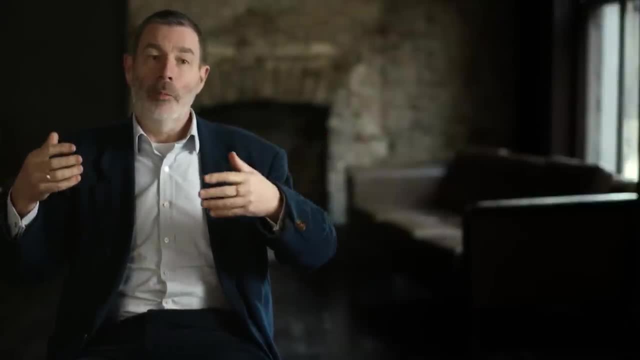 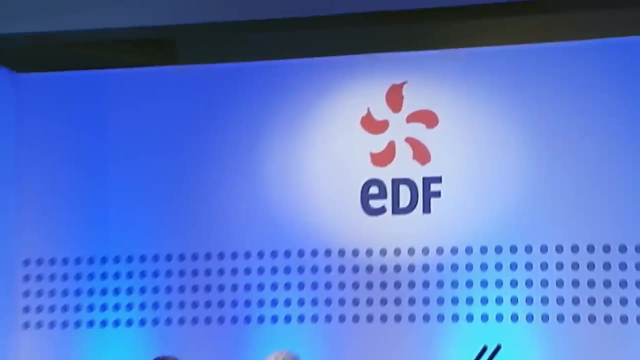 was that the British energy, the British nuclear industry, became effectively the French nuclear industry and was taken over by EDF, the French government's state-owned energy company. The British market, they say, is now their most important one, because our energy needs are the biggest. 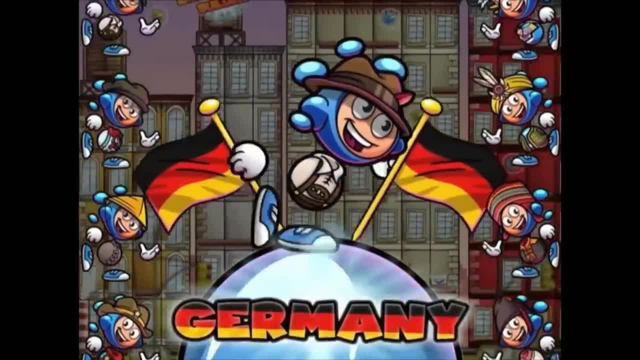 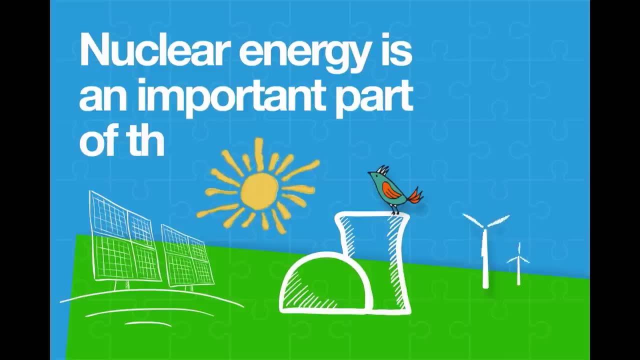 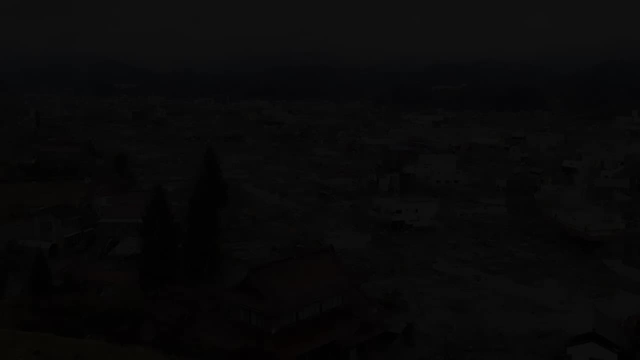 and the most urgent. So confident are they. they're committing for 60 years. As the first decade of the new century came to a close, the nuclear renaissance was in full swing. And then, You know, I still remember the morning. 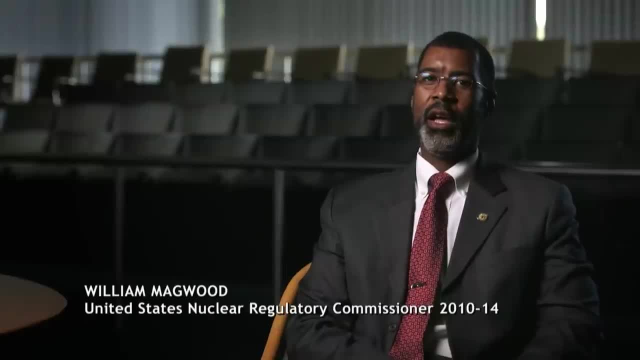 when I woke up and heard there was an earthquake and tsunami in Japan and I immediately started thinking about friends I have in Japan. so I went to the office and, you know, was trying to reach people by email, but also watching events on TV. 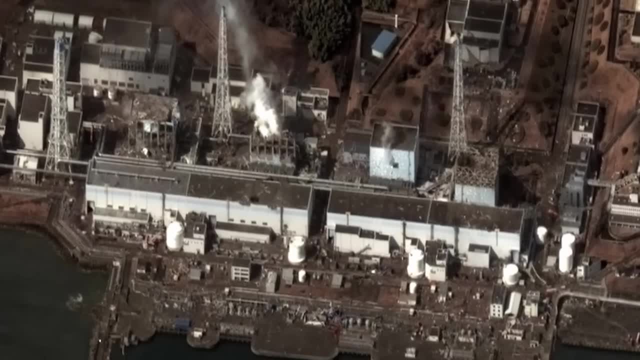 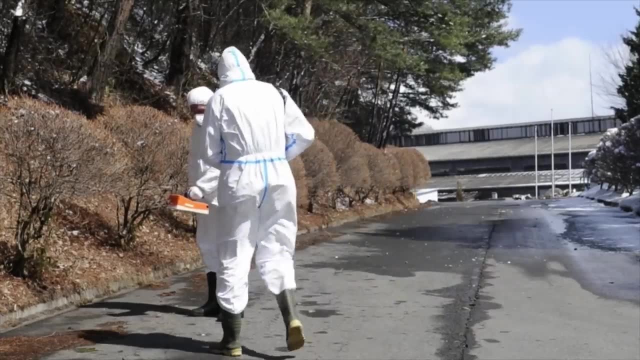 And then we started to notice that there was a problem that it wanted to do for power plants. In the early years, the worst radioactivity in the planet came from all the weapons testing. Now it's coming from the accidents on the civilian side. 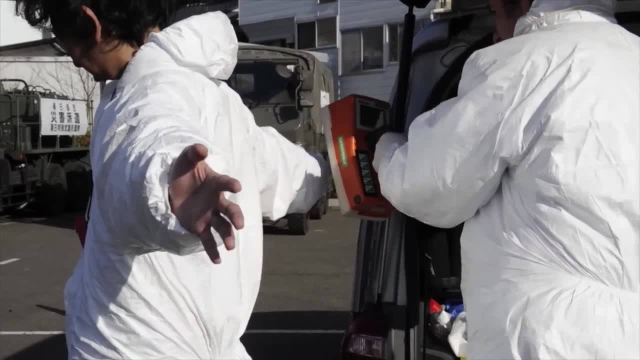 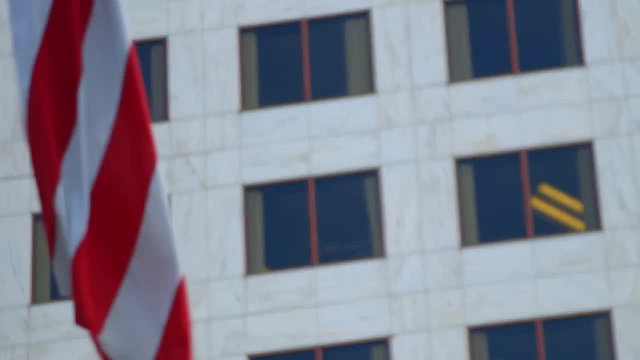 I remember there was one senior staff person who was watching the video on television and he was almost in tears And I remember he turned to me and he said: you know, I spent my whole career trying to keep something like this from happening. 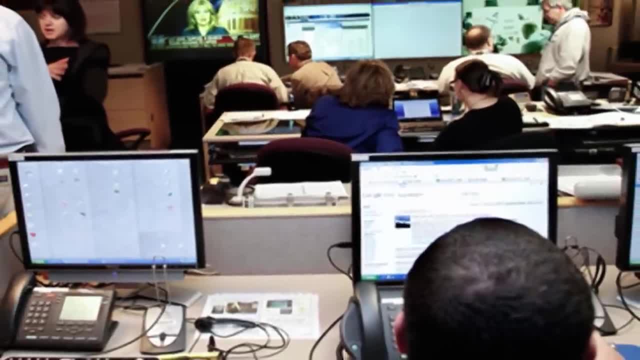 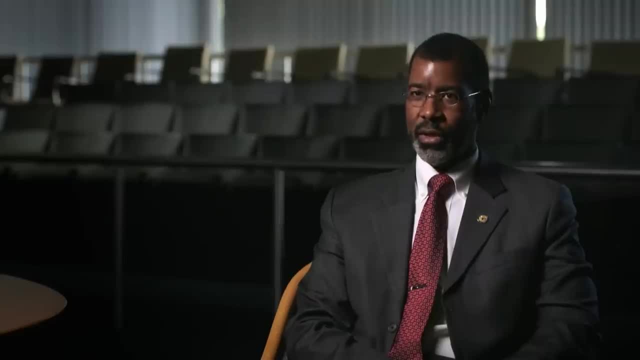 and now I'm watching it happen, And now I'm watching it happen on television, And it was really a very emotional moment. This was a Western-designed reactor and this was also Japan. You know, this is a country, a highly advanced country. 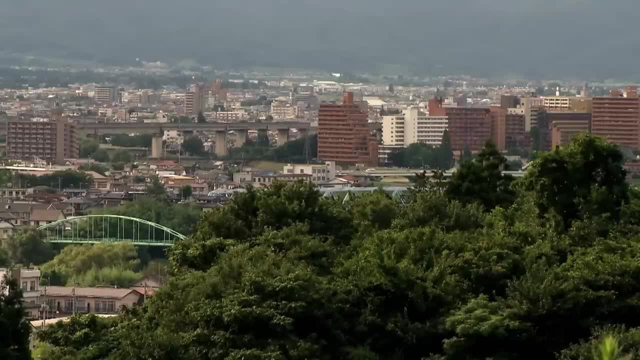 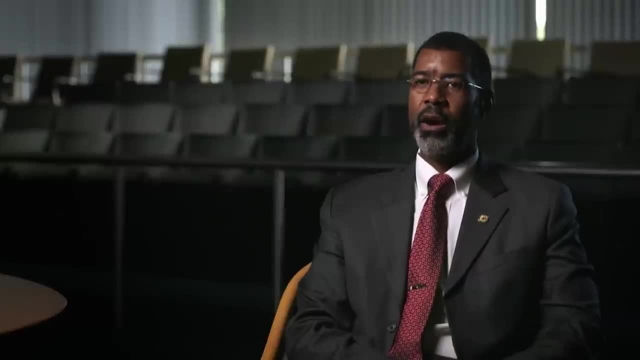 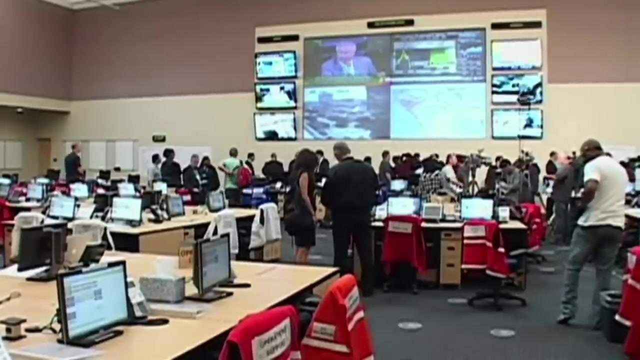 with excellent engineers and somehow this still happened. The most important lesson, I think, from Fukushima is that even if you do your very best in preparing for a natural disaster that could challenge a nuclear power plant, you might get it wrong. We do not believe that there is a chance. 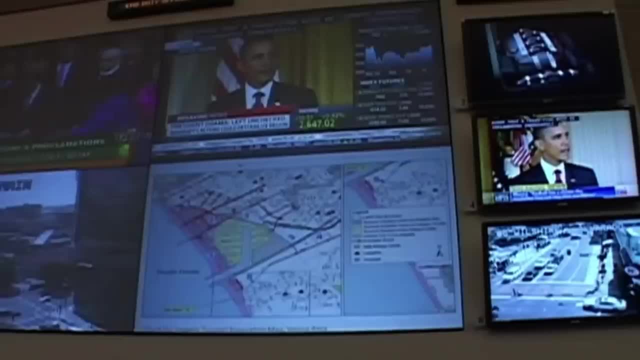 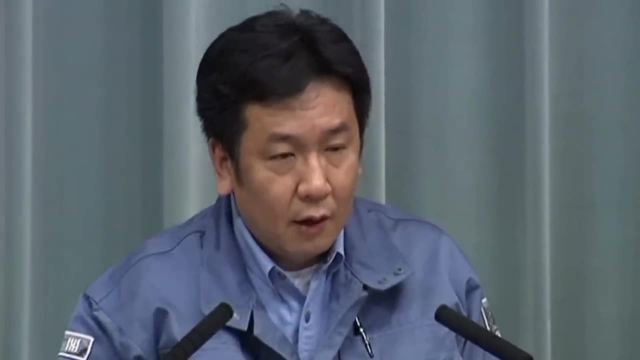 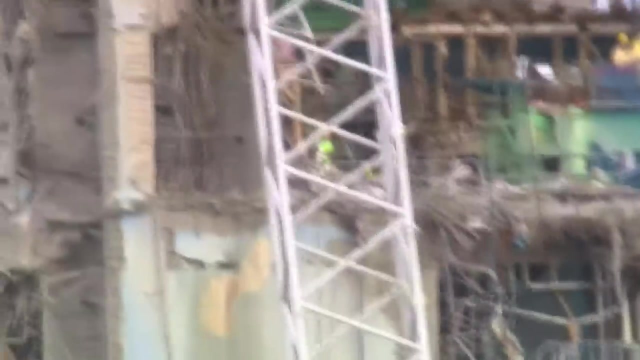 that there would be a significant chance of harmful radiation coming to Southern California. The country's chief cabinet secretary sought to calm fears. He said even if a second explosion were to happen, the reactor itself may not be affected. When Fukushima happened, you could see that the nuclear industry's 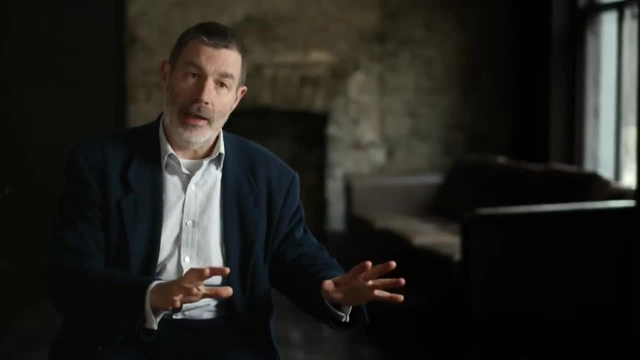 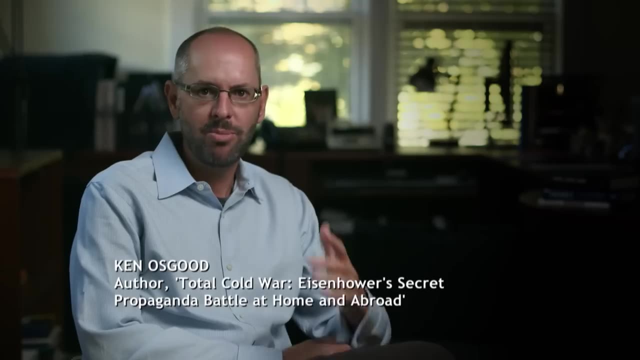 damage limitation machine had moved into action. As fate would have it, I was actually myself traveling with my wife through Japan, and for me personally, I remember hearing these reassurances from the Japanese government and I couldn't help but thinking of the sort of irony. 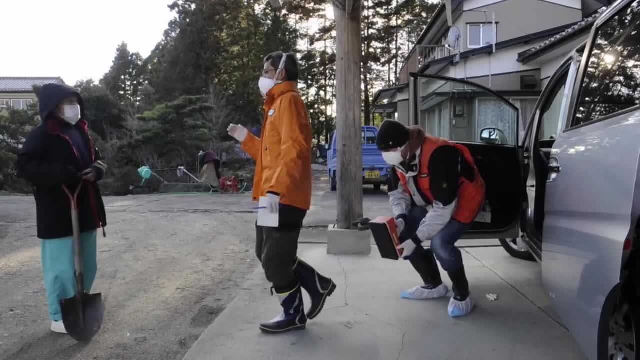 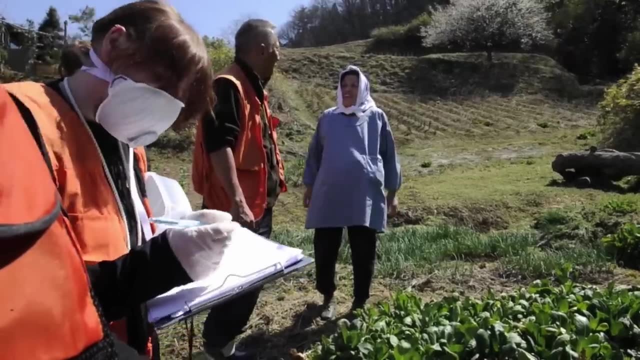 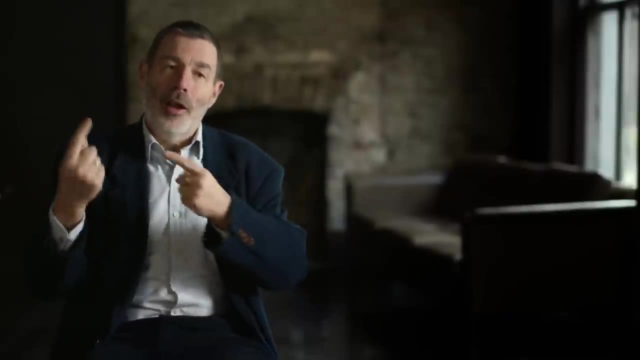 of this message, that the country that had been such a target of this peaceful atom message in the 1950s was now itself putting out its own version of reassurance of atomic energy, PR. There was some extraordinary evidence and so many memos and emails going around at the time. 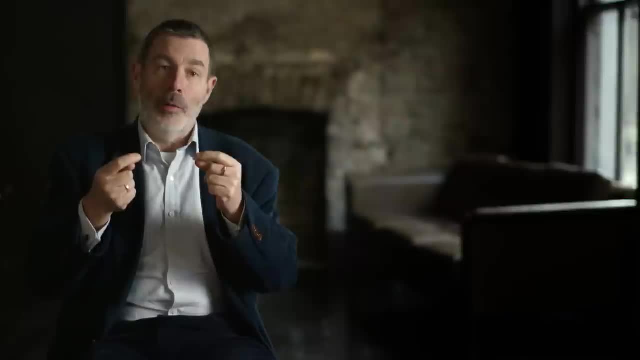 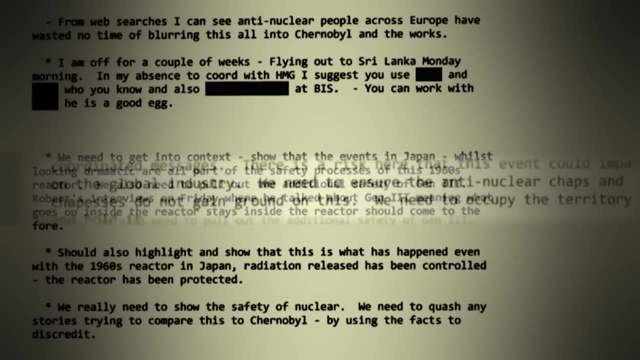 so that one senior official in the business department, whose name to this day I still don't know, but he's obviously old school, because he said we must do what we can to stop the anti-nuclear chaps and chapesses getting their messages across. 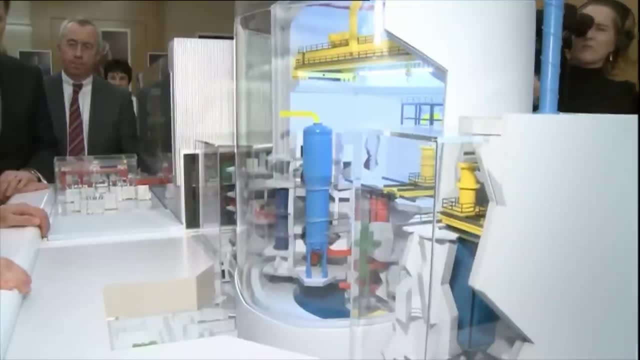 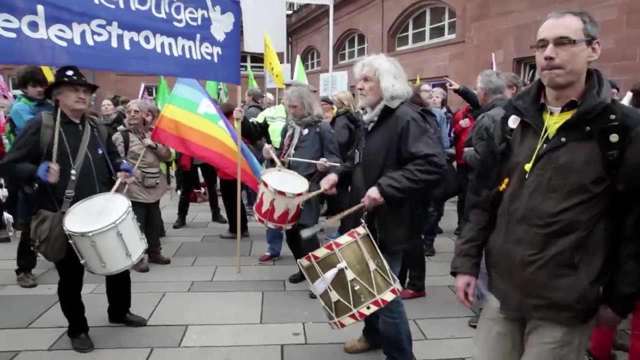 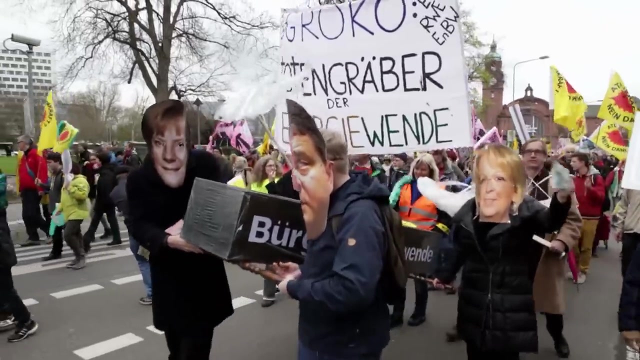 Faced with their biggest PR headache since Chernobyl, governments united with the industry to show their support for nuclear, with one very obvious exception: Unrelated automation Desktop Counter installed After Fukushima. it's about something else. It's about reliability of all risks. 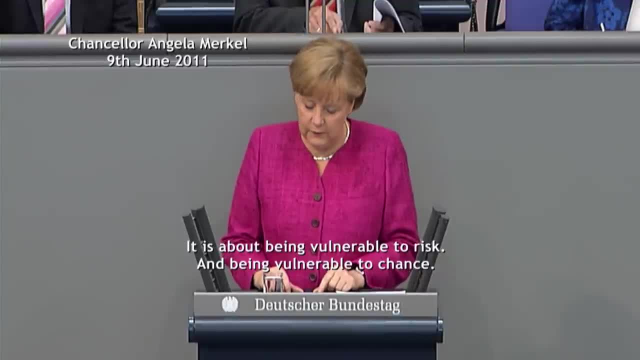 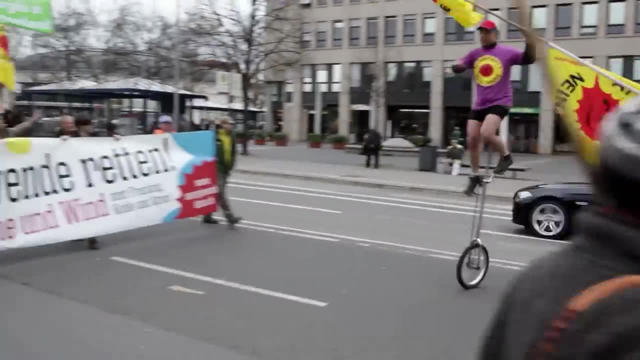 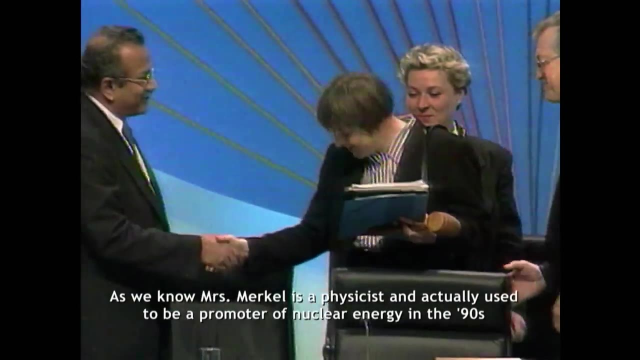 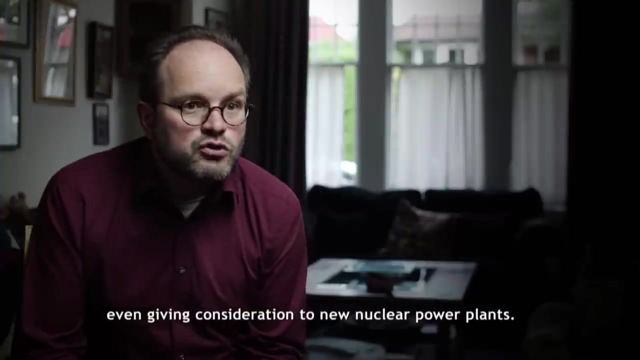 and about reliability of insurances of probability. By 2020, the use of nuclear resources is over in Germany, I think. for Merkel, the atomic hack- It was a big step. Mrs Merkel is known to be a physicist and in the 90s she was actually a supporter of nuclear power, including considerations for new nuclear power plants. 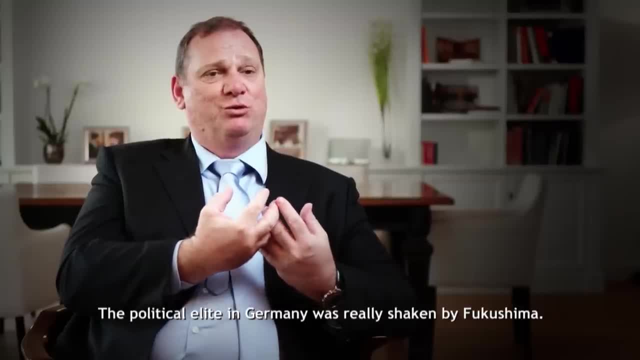 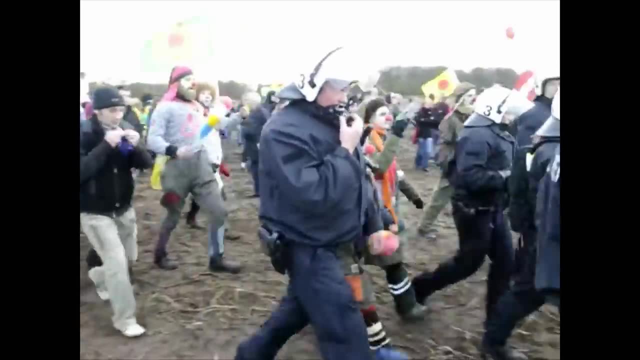 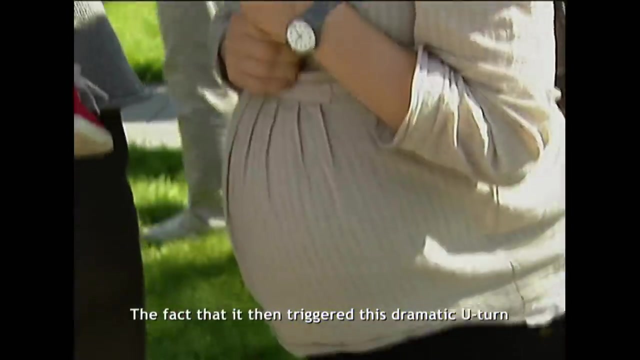 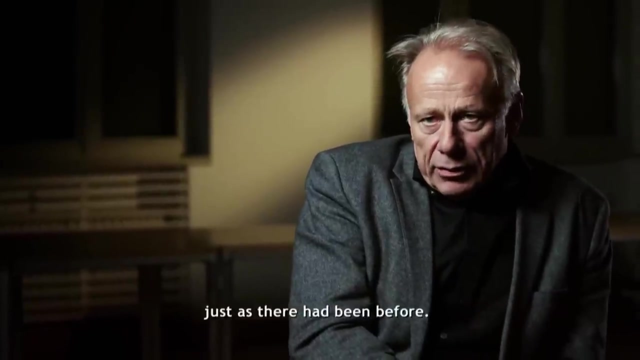 The political elite in Germany was really shaken by this Fukushima Danger, Danger, Danger Emergency. Fukushima alone would not have been enough. The fact that they have triggered this dramatic reversal in Germany- this had to do with the fact that in Germany there was still a broad consensus in the population against it. 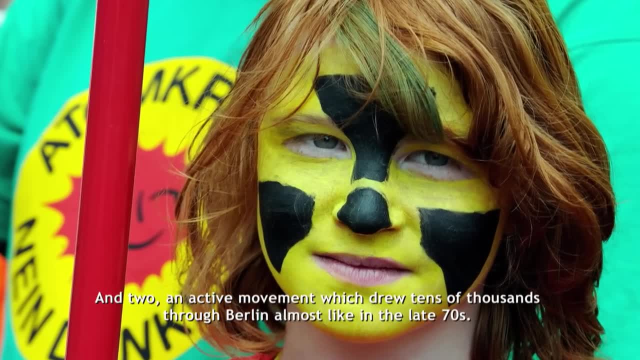 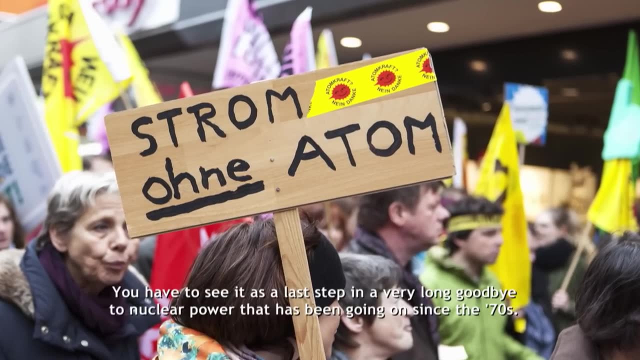 And secondly, an active movement that, almost like in the late 70s, was pulled through Berlin by tens of thousands. You really had to see this as the last step in a long farewell to nuclear power, which has been going on for centuries. 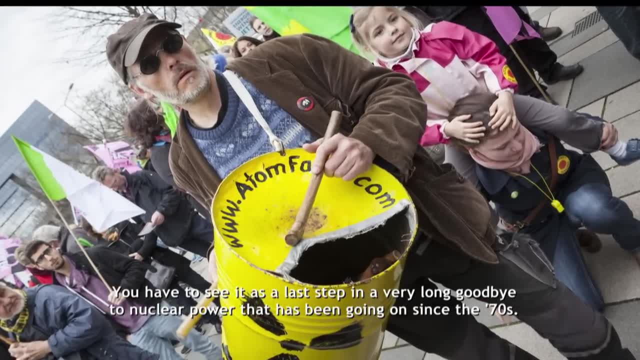 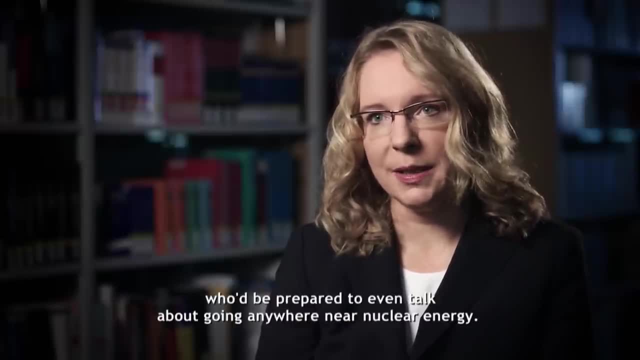 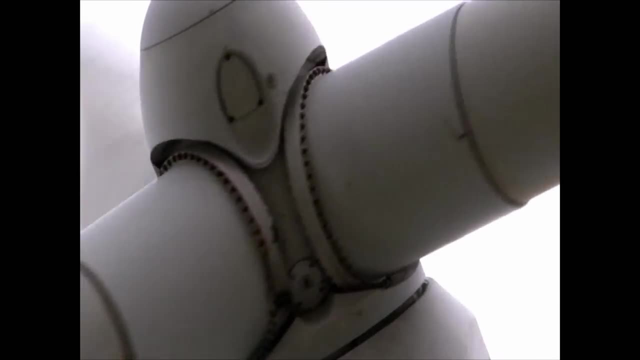 No party, no matter what colour, would want to discuss nuclear power in the first place. So the topic is completely gone. In Germany today, nuclear power is officially over Elsewhere. it's not dead, but it's not exactly thriving either. 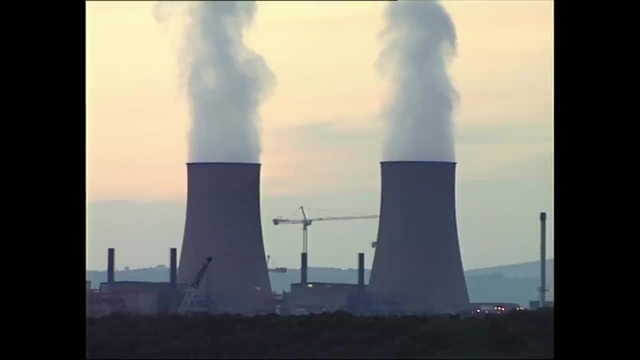 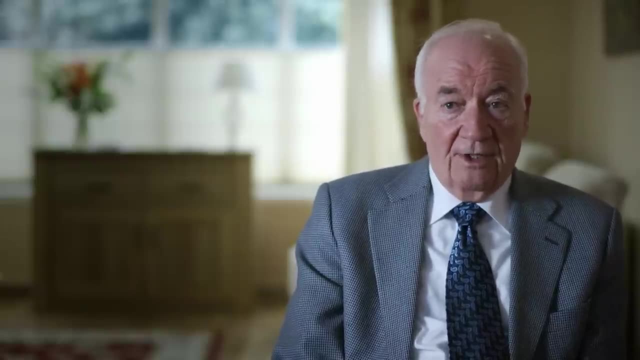 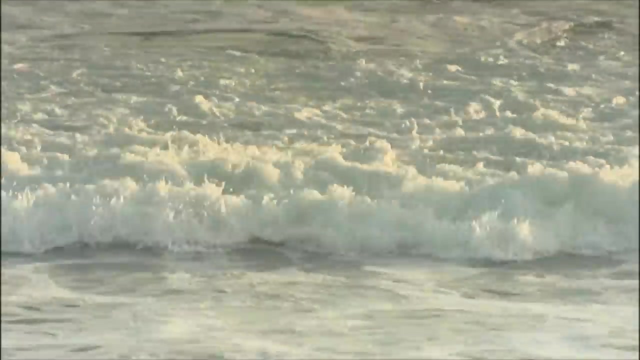 We don't have a British nuclear fuel anymore and I find that sad. Some of us older directors get together once a year for dinner- and one's due next month- And we sit around the dinner table all Wednesday and weep into our wine or beer about what's happened to our company. 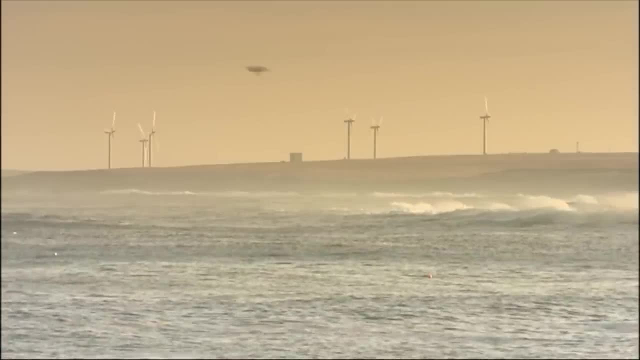 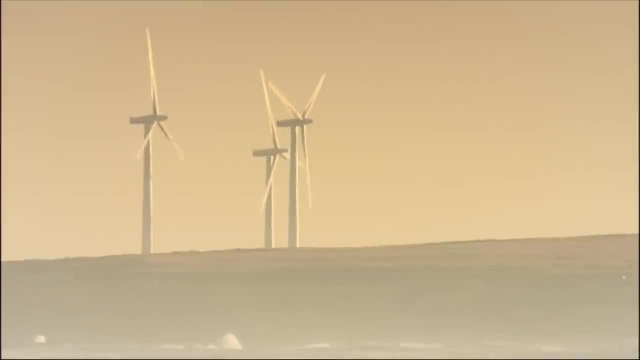 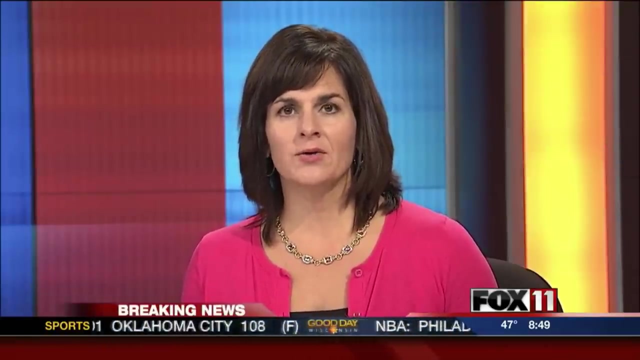 At this point. solar and wind power are growing so fast and the costs are declining so rapidly that nuclear is like this old dinosaur- It can't possibly keep up. Some breaking news to share with you: this morning The owner of the Kiwani nuclear power plant says it'll shut the plant down next year. 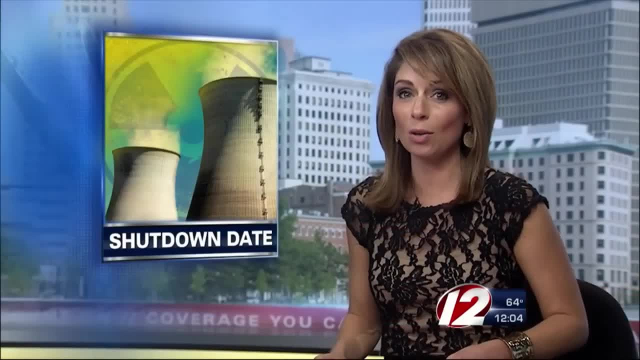 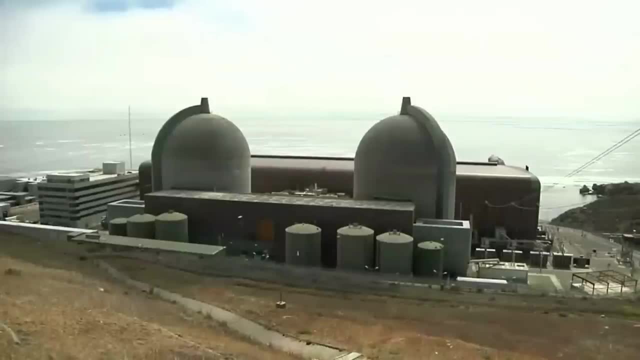 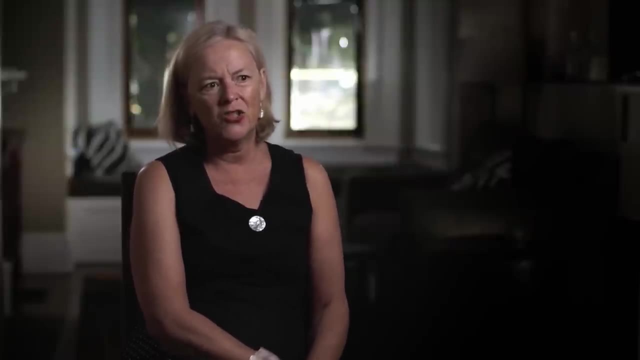 The only nuclear power plant in Massachusetts will be shutting down by 2019.. Citing California's changing energy landscape, Pacific Gas and Electric is closing Diablo Canyon. The real factor in the United States is just practicalities. I mean, we had the discovery of natural gas in large quantities and it's much cheaper and it's much easier. 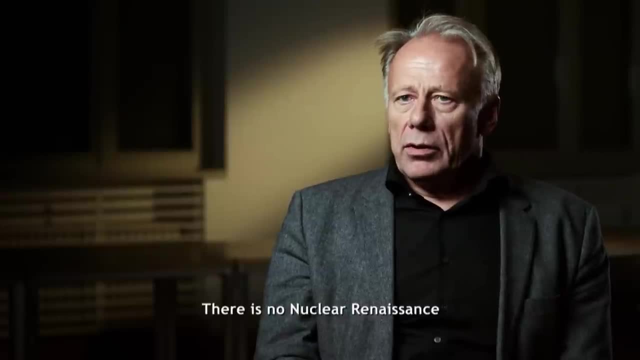 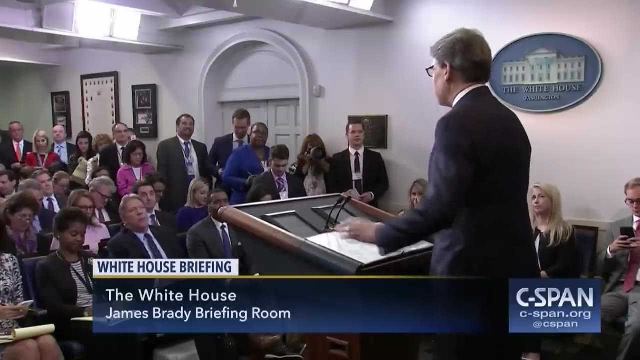 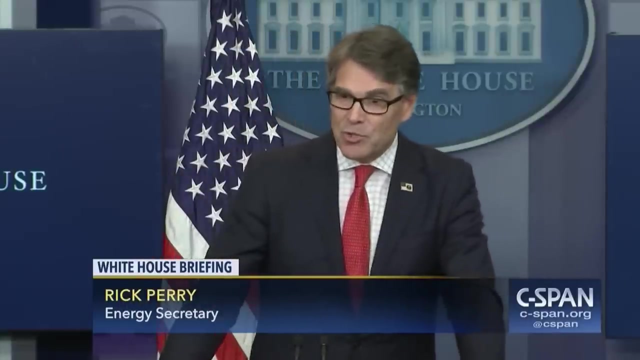 There's no nuclear renaissance. It's a fairy tale from the propaganda department. Of course, nuclear power still has its champions. One of the things we want to do at DOE is to make nuclear energy cool again. What are the problems that the people who object to nuclear power really have? And can we solve those technically? Can we make nuclear power that doesn't produce waste, that lasts for hundreds of thousands of years? Can we make nuclear power plants that can't melt down? And I think the answer to those questions is actually yes, And dozens of new nuclear start-ups are betting on experimental next-generation reactors to save the flagging industry. 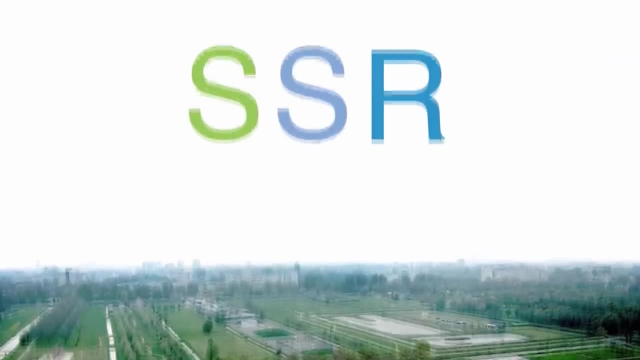 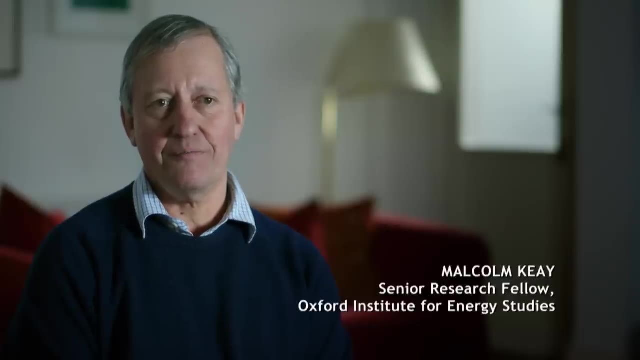 though it's not yet clear if they'll succeed. Whether it will happen or not, I think we can't say just now, because for the latest generation of reactors really there isn't enough experience, enough knowledge of whether you can bring these costs down. 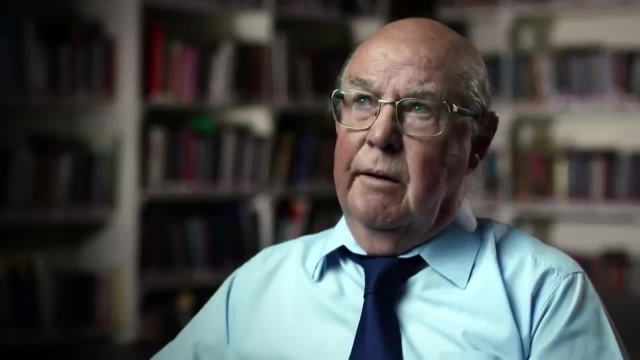 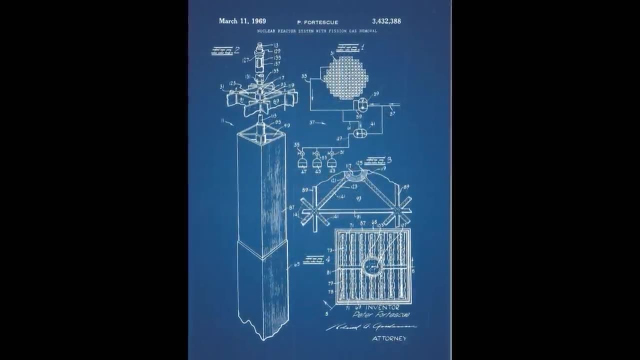 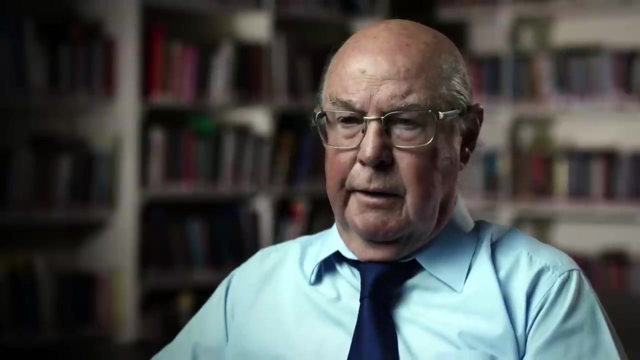 I used to say that the best reactor was a paper reactor. It was a reactor that only existed on paper, Because once you actually start to pour concrete and weld steel, it turns out to be a lot more difficult than you thought, And that has been historically the case with every successive design of reactor that has been tried. 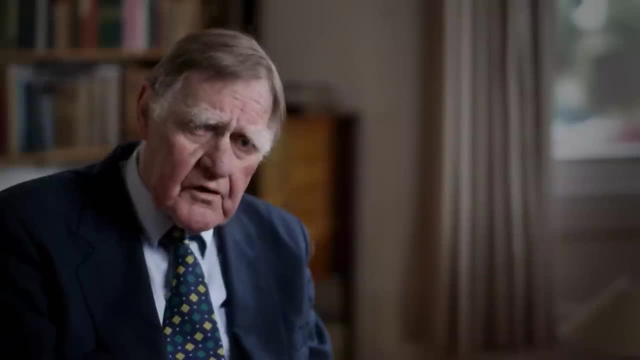 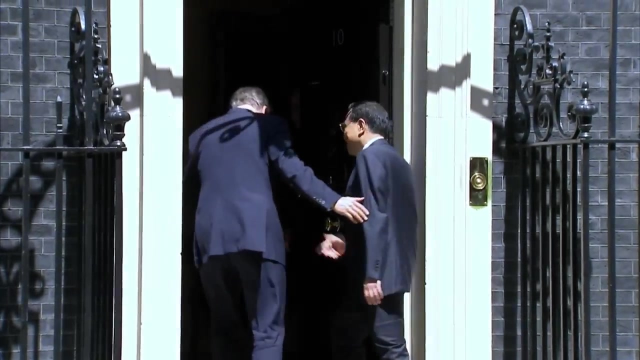 I don't think you can be confident that it is going to happen this time in the Western world. I think you'll be confident it's going to happen in the Far East. Some of the oldest players in the nuclear game are now turning to China. 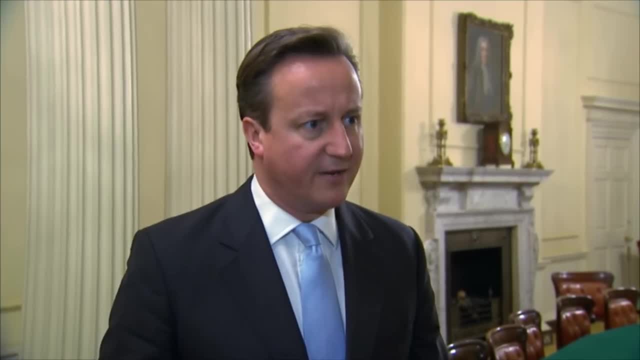 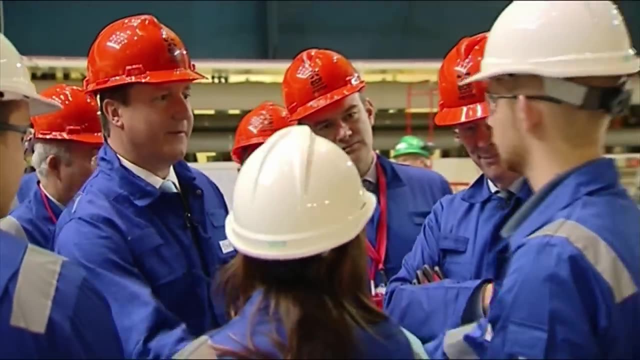 Make no mistake about it. this is an important day for Britain. Willing to pay whatever it takes to keep the nuclear dream alive. The focus has been on a plant called coal. The focus has been on a plant called Hinkley Point C. 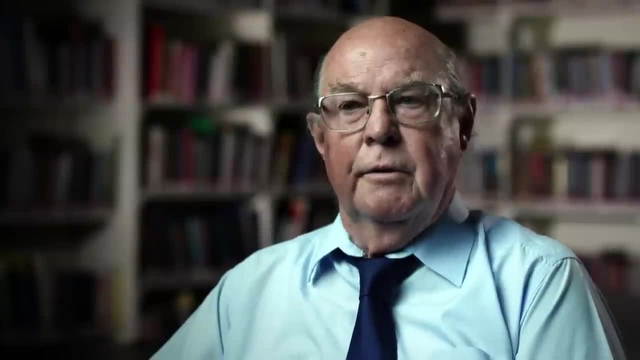 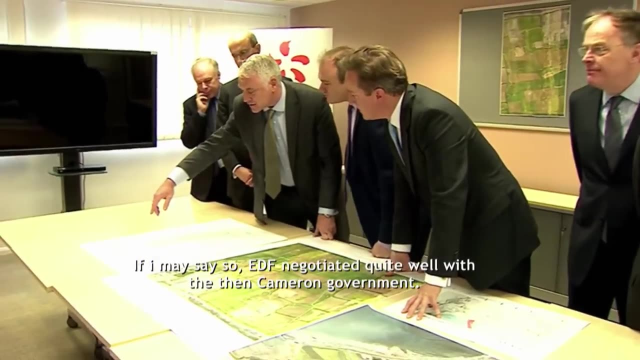 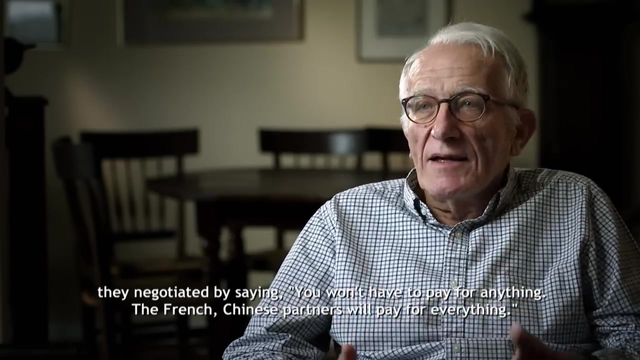 And the claim was made by EDF that this would be done absolutely without any public subsidy, Which turned out, of course, to be complete nonsense. EDF, if I may say, negotiated well with the government at the time. Cameron, They negotiated by saying: you don't pay anything. 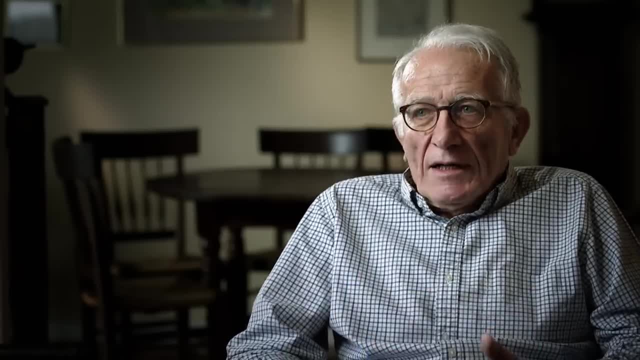 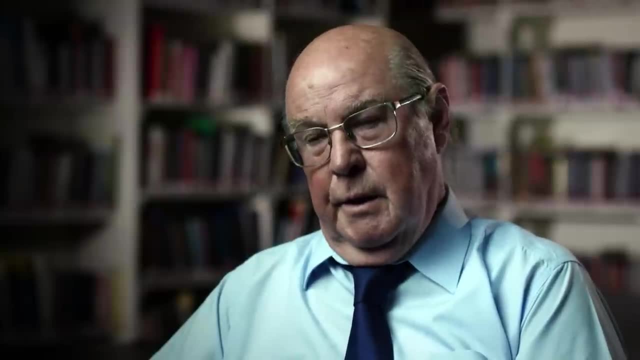 it's the French and Chinese partners who pay everything, But on the other hand, you guarantee us that we'll be able to cover our costs. The subsidies got less and less well disguised, until they got to the point where they were offering a guaranteed price for the electricity. 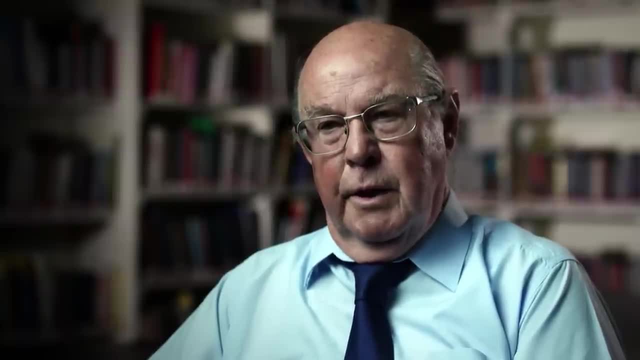 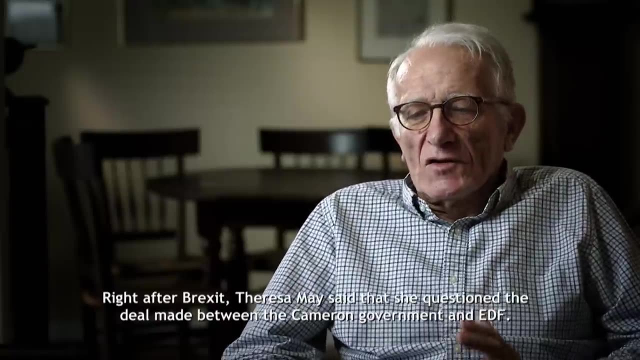 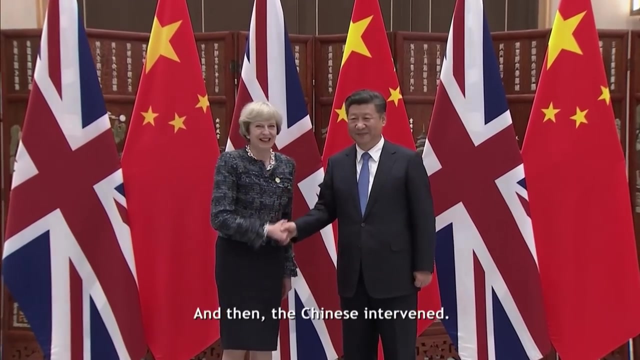 for 35 years, at three times the going rate in the UK. Just after Brexit, Theresa May said that she was questioning the deal that had been passed between the Cameron government and EDF, And then the Chinese intervened. It seems that this Chinese intervention 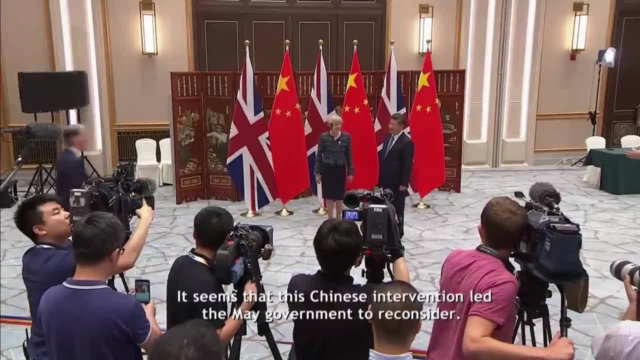 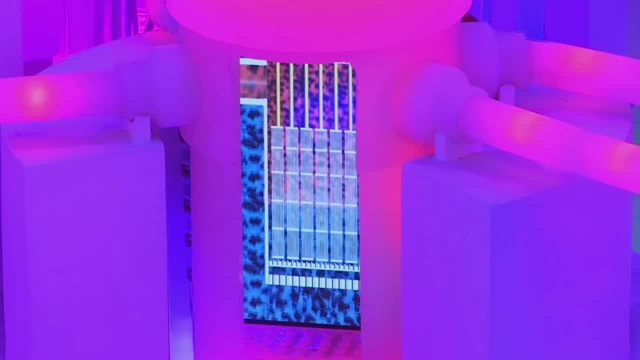 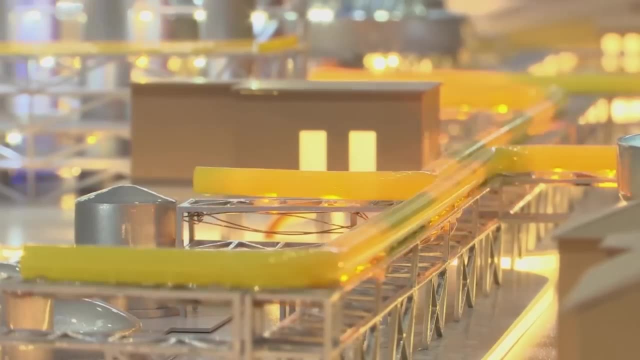 has led Theresa May's government to reconsider, and the deal is off to a good start now. China is today the only major country successfully building reactors at home and selling their expertise abroad, But only time will tell whether the Chinese nuclear barons can escape the political pressures that have bedevilled their Western counterparts. 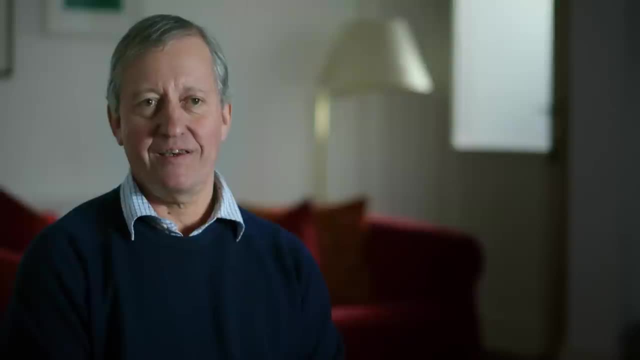 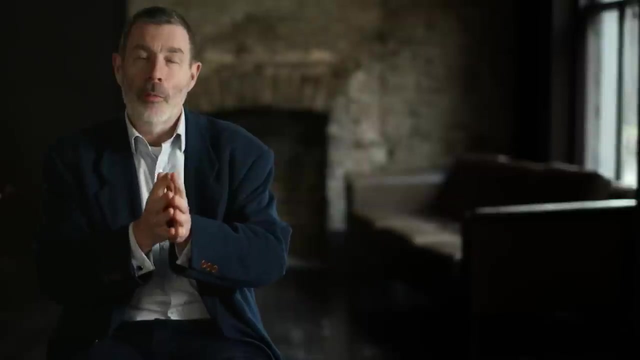 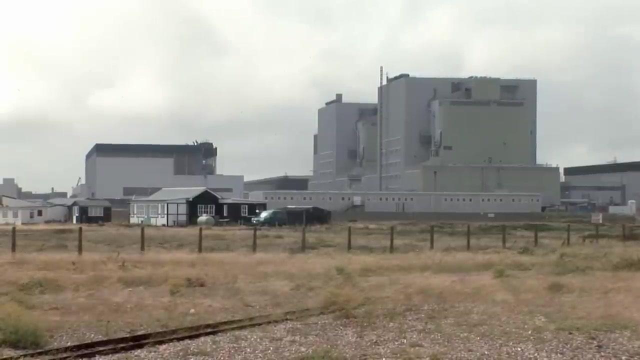 for so many decades. It's an inherently political technology because of the nature of the risk and the safety aspects. It's economically so complex, so difficult, so tricky. It's kind of pulled under by its own dead weight, Unless there's a major breakthrough. 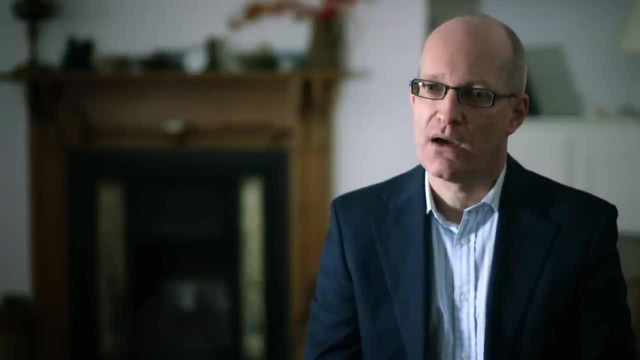 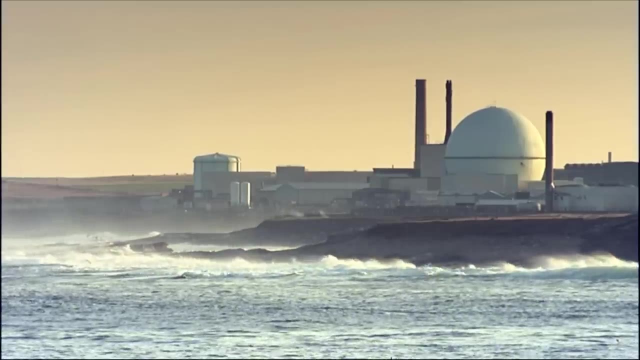 to a fundamentally more economic form of nuclear power. nuclear is always going to be struggling to survive. Nuclear power always enjoyed powerful backing from scientists, engineers and politicians, And it was the Chinese and the Chinese and the Chinese, the Chinese and the Chinese. 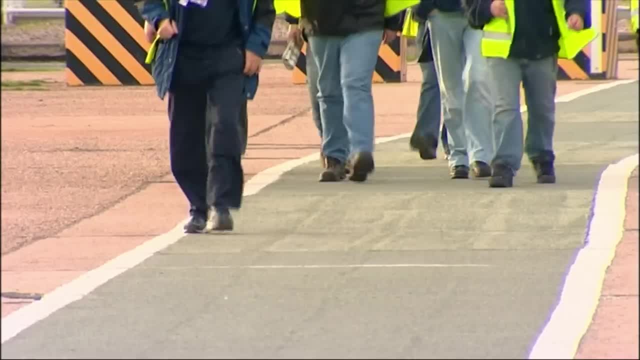 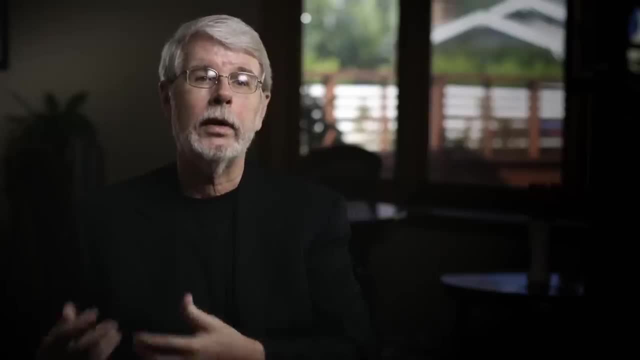 who felt that they were best equipped to decide its future. It felt like if the public would just leave them alone, they would control the technology, they would fix the problems with the accidents. You know, if they just let us keep working, we're going to take care of all your concerns and all your problems.